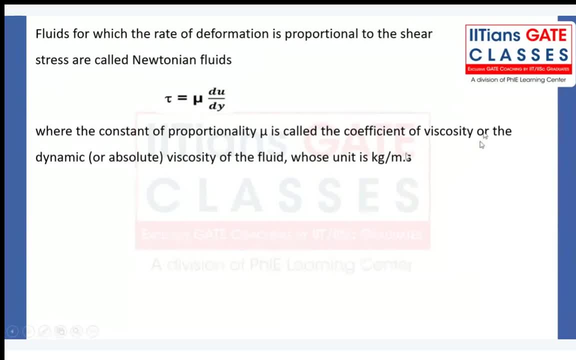 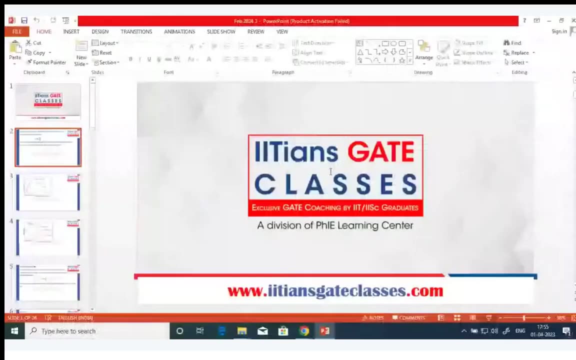 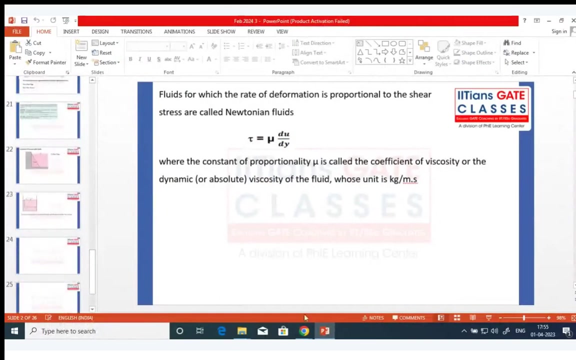 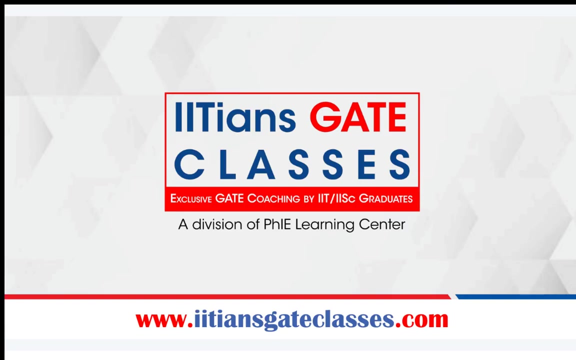 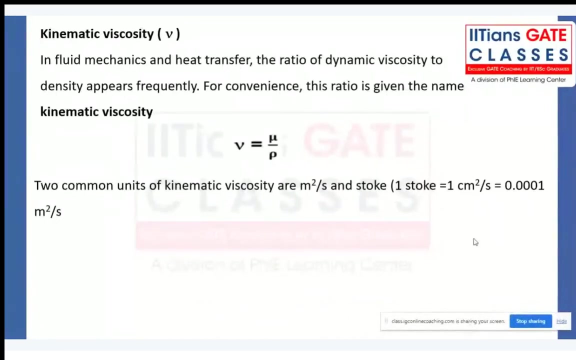 So we have discussed. the fluid which follows the Newton's law of viscosity will be called as Newtonian fluids, and the fluid which does not follow the Newton's law of viscosity, that is, non-Newtonian fluids. Just wait, Just wait. So note down one more term: kinematic viscosity. 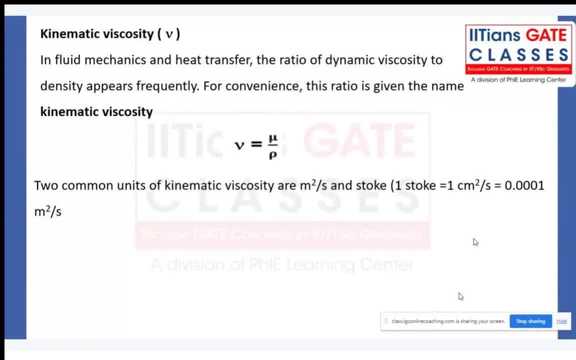 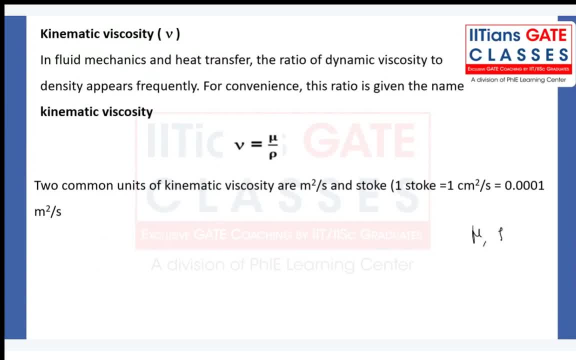 So you have to know that the fluid is going to be very important. So you have to know that the fluid is going to be very important Generally whenever the term is coming like mu by rho, right, Generally, whenever the term is coming mu by rho. 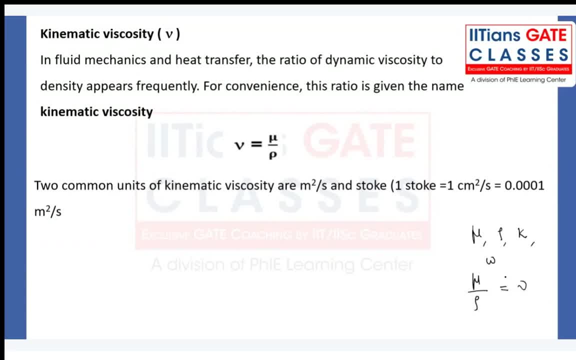 we directly replace it by kinematic viscosity. Only for that purpose we have extra term in our fluid mechanics or heat transfer. that is kinematic viscosity. There is no any other reason. If you ask me, sir, why there is a dynamic viscosity there. 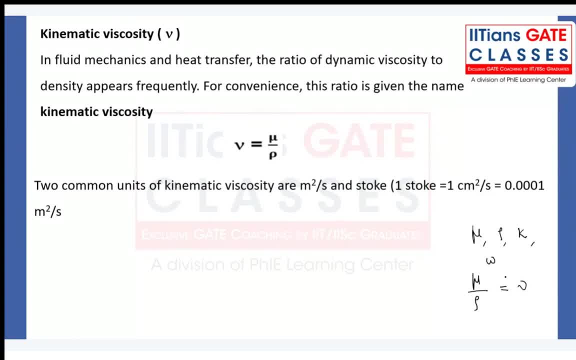 then why the kinematic viscosity? it is present there. So that is only the reason I told you, right? So it is basically All the definition which is given by the researchers when they started doing the fluid mechanics research during the 16th century, right? 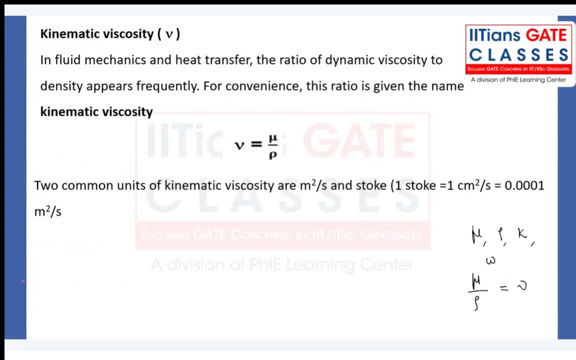 So what? I will be suggesting you that we cannot do much, in that We cannot go back to the history and see that what is a reason for origination of these parameters So directly, blindly. we have to trust that, whatever the research they have done, that is accurate. 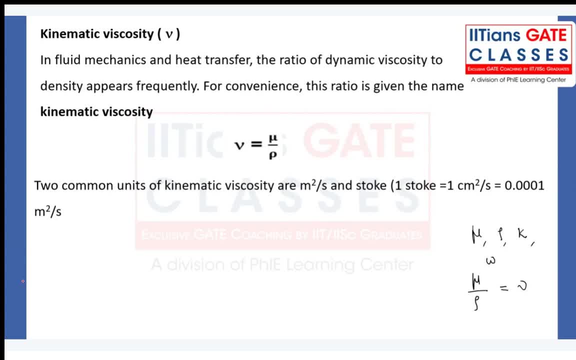 Now here you just note down. It is a ratio of the dynamic viscosity to the density right. That is called as kinematic viscosity. Now, that is a very simple definition. I can directly tell you without telling you the 5-minute history of that. 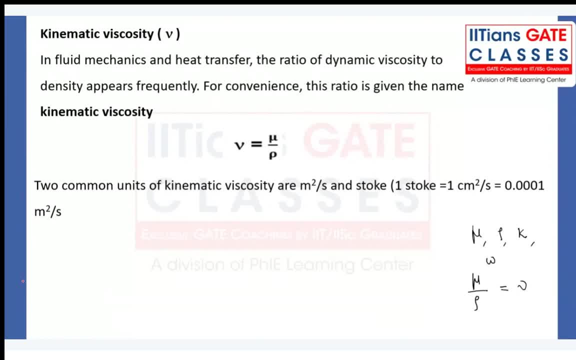 But again, you might be thinking: okay, that is a separate term which is being defined in the fluid mechanics at the starting only. No, it is not like that right. So to give you idea about that, I have just told you this thing. 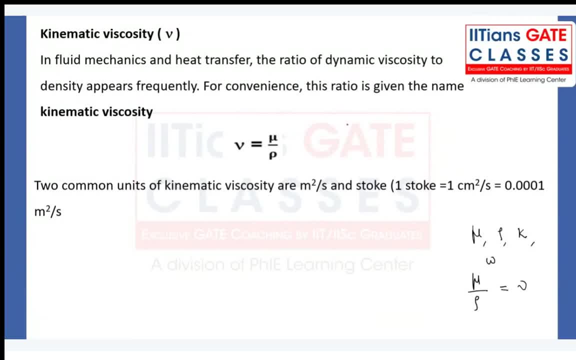 Now, what is a unit? So, unit of viscosity, we know that, Pascal's again. And density will be kilogram per meter cube. So when you see this, I am talking about the SI unit- Then Pascal's again, Then Pascal's again. we can write further as Newton per meter square second. 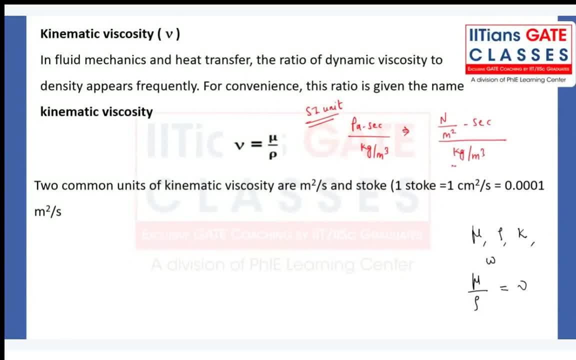 divided by kilogram per meter cube. Once again, I am writing from here to here. What is that? Newton Further? we can write kilogram meter per second square into second divided by kilogram per meter cube. So when you try to solve this one, you will be getting meter square per second. 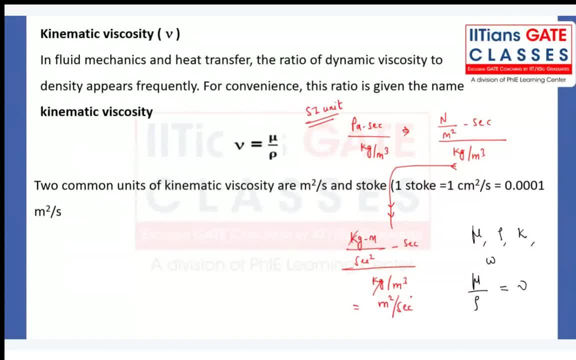 Make a note of it. That is a SI unit, right? And if I will be asking you CGS unit of kinematic viscosity of nu, then what you will write, The CGS unit, will be what Centimeter square per second right? 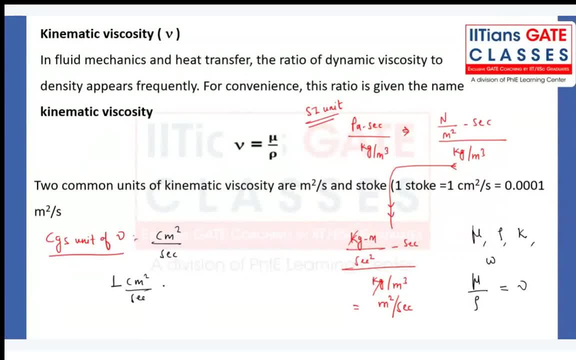 And one centimeter square per second will be what? One centimeter square per second will be 10 power minus 4 meter square per second, And what we can write this one. Anyone know that Any other specific name is there for that? 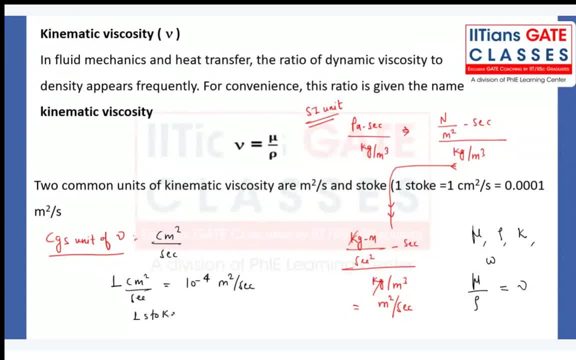 One stope Stoke will be equal to 10, to the power, minus 4 meter square per second. Make a note of it. And, in terms of dimensions, what we can write: Meter square, L, square by T. So what we can write. 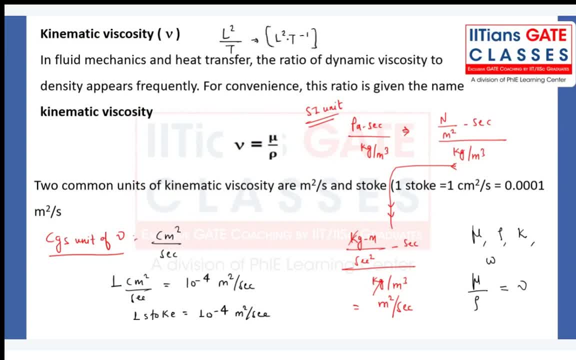 Like this. So one is stoke, Stoke is nothing but CGS unit of kinematic viscosity. So if you know further, we used to get the question like this: What is the difference between dynamic viscosity and the kinematic viscosity? 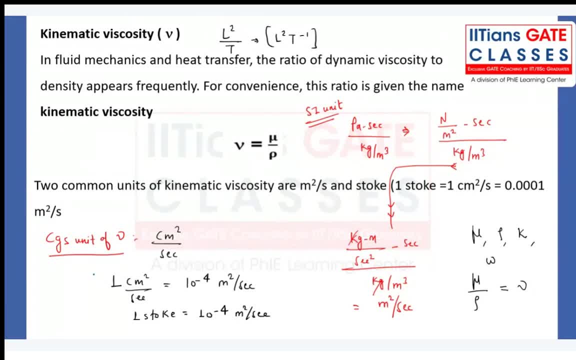 So dynamic viscosity. when you see that how to determine the dynamic viscosity practically, We have to take the fluid element in a container and then we have to rotate it right And whatever the deformations rate will be there and whatever the amount of shear stress we have applied into the container, 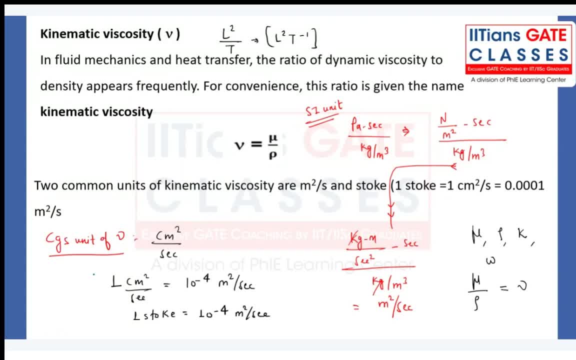 then If you just divide those two terms I will be getting the viscosity. So with the application of the external force we are measuring that one, Which one, What we call dynamic viscosity. But here in the kinematic viscosity, if I want to measure for any fluid, 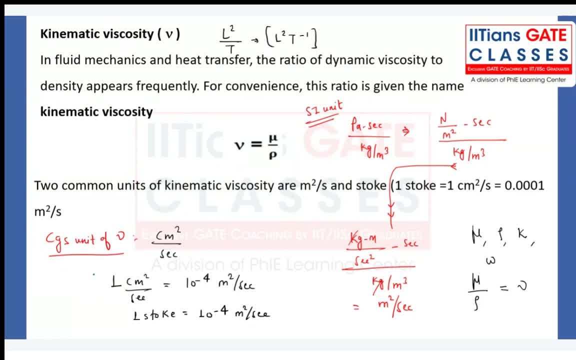 directly, I will not be applying the shear stress right, It is just being rotated with the help of maybe some gravity right, For example. And in that case, directly, I will be measuring the deformation rate And I will take the, you know, basically the ratio of what- the actual dynamic viscosity of that particular fluid to the density of the fluid. 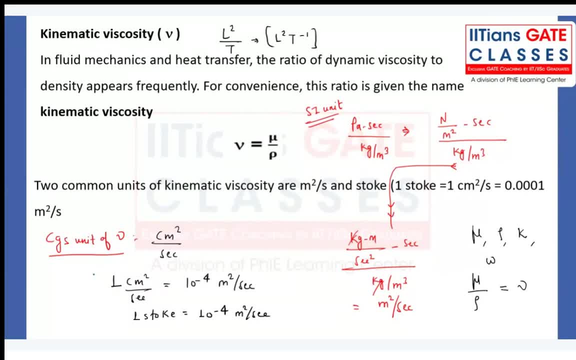 So that will give me directly kinematic viscosity. So why the name itself is coming over here: kinematic, Because there is no particular force has been involved. right, If you see the unit also: meter square per second right. 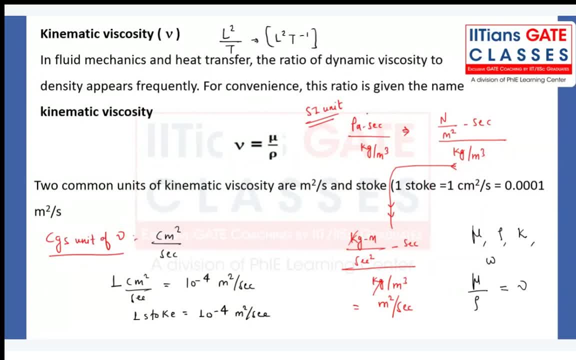 There is no such a term called Newton there, But when you see a dynamic viscosity, that is a Pascal second right. So that is a. They are the terms. The term involves Newton, So that is why the name is given: dynamic viscosity, right. 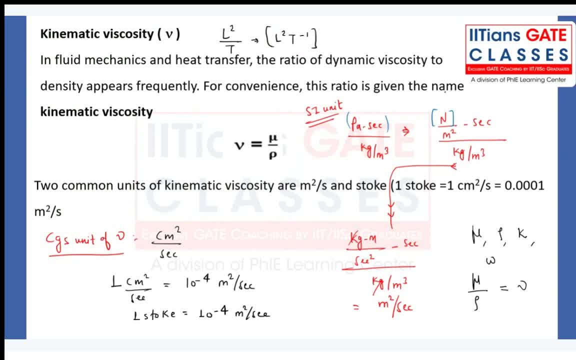 Now make a note of it. Now, one drawback of my teaching is something you might be, you know. you may be thinking that, Sir, in all the subjects, the particular topic you know, we have to learn like this only right. 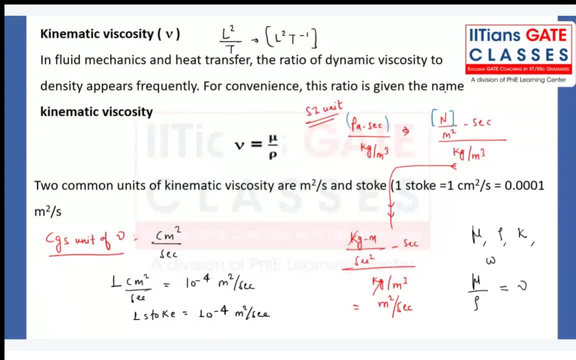 We have to go back to the history And fundamental concept, the numerical. But I will be suggesting that do not do PhD in any particular topic. That is my first suggestion. If you do PhD with less number of numerical, you may be end up getting only 40 marks or 30 marks. 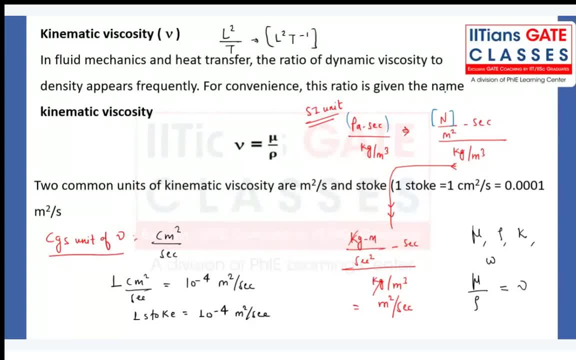 Sometime you may not be able to clear the cutoff also, right? So please, whenever it is required, then only do the PhD, Otherwise it is not at all required. right, Because you might be thinking right, That is a temptation because of my teaching, right? 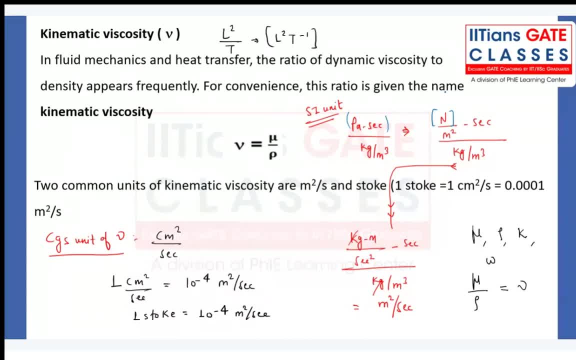 So, please. So that is what I am just. you can consider it like a precaution. Only fundamental thing has to be clear. Plus, you have to solve enough amount of problem regarding that particular single topic. Remember that Now all of you have noted down. 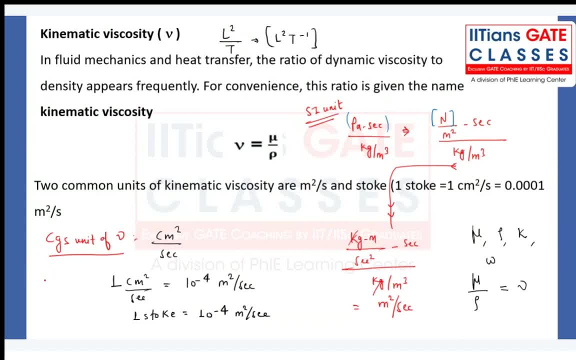 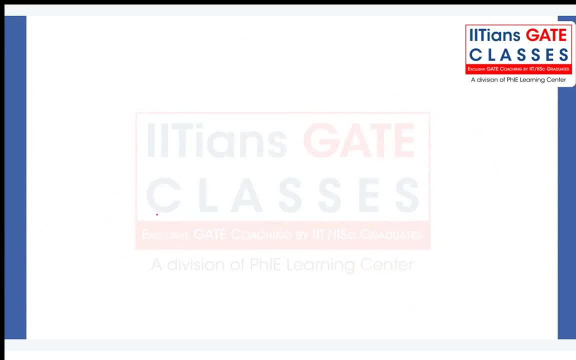 Can I move to the next one? Okay, So here I would like to tell you the reason of viscosity right In liquid and gases. So note down the first topic: Reason of viscosity In liquids. What is the reason of viscosity in the liquids? 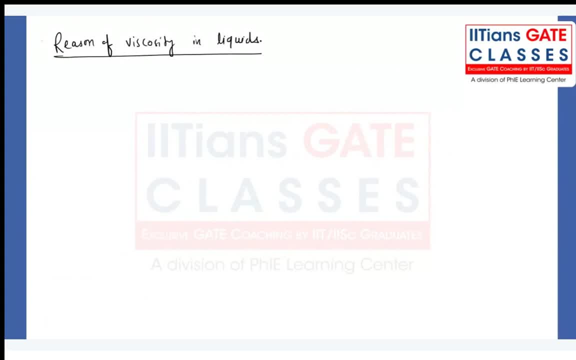 Anyone know that. So liquids and gases, if I just say So, they are basically two major, you know, factor or mechanism responsible for the viscosity, Two major what you call factor or mechanism Or mechanism responsible for viscosity. So one will be definitely I know everyone know that. 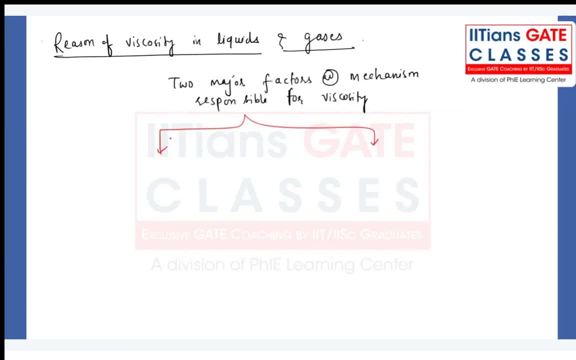 I just categorize into two. One will be the cohesive force, right, One will be the cohesive force. Like you know, that cohesive force, adhesive force, Like that, here we are telling about the cohesive force, or molecular bonding force, Molecular bonding force between the same kind of molecules. 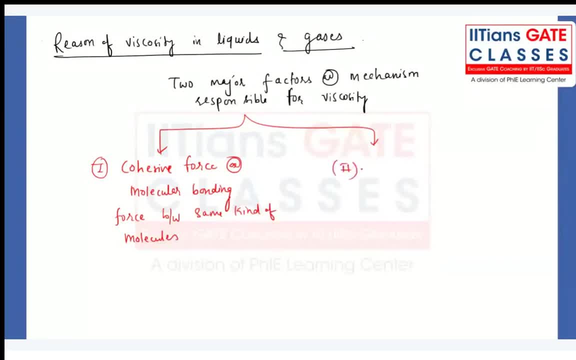 Second mechanism, we will be having mixing or molecular momentum exchange, Molecular momentum exchange. So basically, if I will be talking about the liquid case, In liquid, which one will be responsible? This will be responsible For the liquid. the major factor which is responsible for the viscosity is nothing but cohesive force. 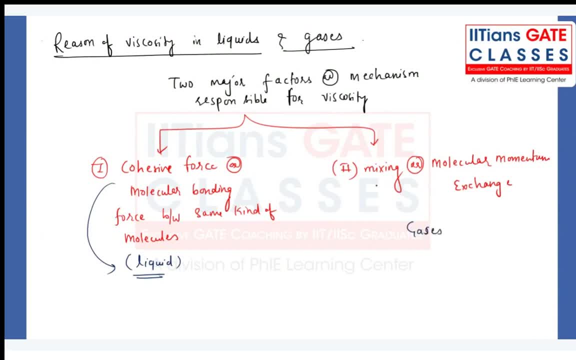 In case of gases, this is the basically responsible. See, don't think that in liquid, only cohesive force is there. There is no momentum exchange. But out of these two, the major which is affecting the reason of viscosity, is that, Or the reason, accurate reason that is responsible for viscosity is cohesive force. 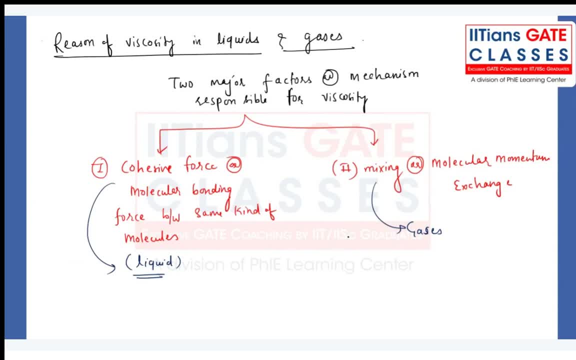 Between the liquid molecules. right Again, molecular momentum transfer is also happening in the liquid also, But that is less dominating as compared to cohesive force. Again, in the gases also we have the cohesive forces, But that is less dominating as compared to mixing or molecular momentum exchange. right. 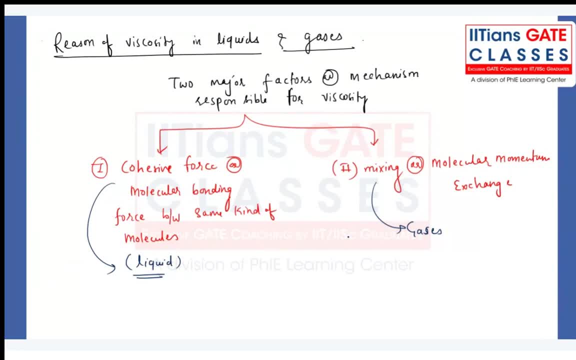 Make a note of it. Now we have to see, my dear friend, the effect of temperature and pressure on the viscosity of the liquid and gases. For fluid mechanics to understand completely, you should be finished your differential equation. That is a mandatory. 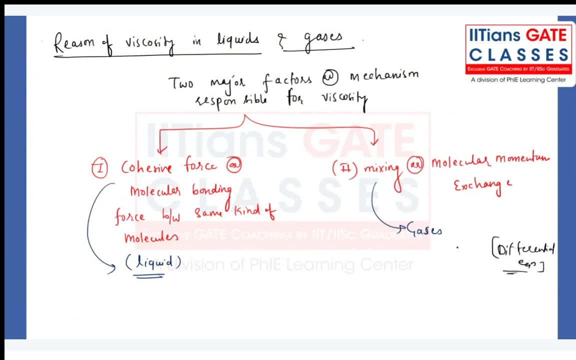 Otherwise, always you will struggle in partial differentiation, partial integration. Why constant has not been added? Why some other arbitrary variable has been added, been added? so all these doubts should be there, but please make sure that you you know, clarify from the mathematics, because fluid mechanics is nothing but mathematics, only it is just. 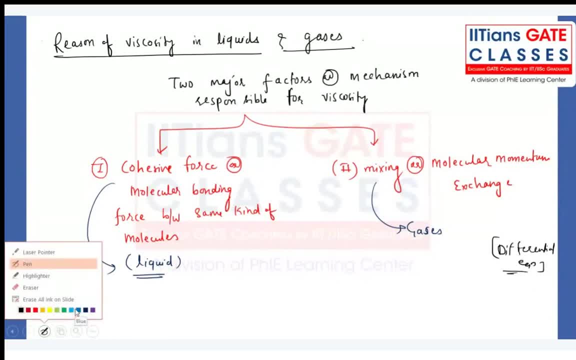 added that we are doing the mathematics of, not the numbers. we are doing the mathematics of fluids. that's it why, because i have seen in the last, particularly, you know, for the gate 2023 batch, some of these strengths, not all one or two students, they are doing actually you. 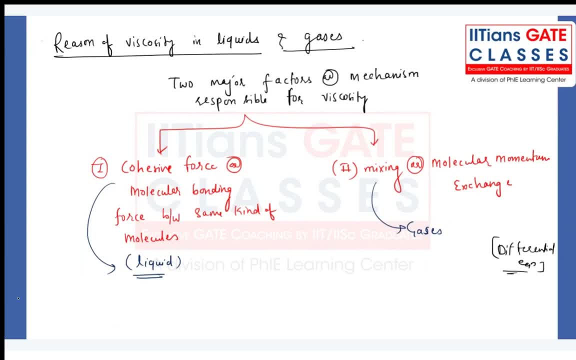 know. always they used to get the doubt. doubt is genuine, but they used to do phd. in every topic they end up getting only, you know, 26 or 28 marks only. so there is no use of that, all those research work you can do after getting good rank in gate exam. 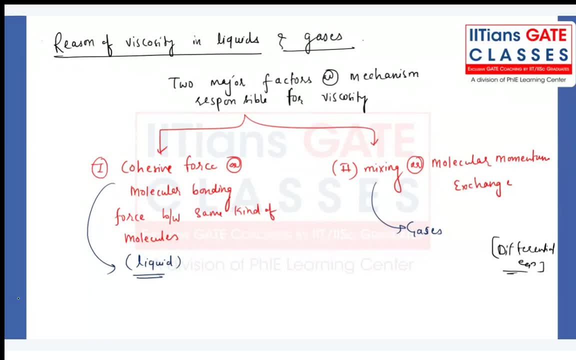 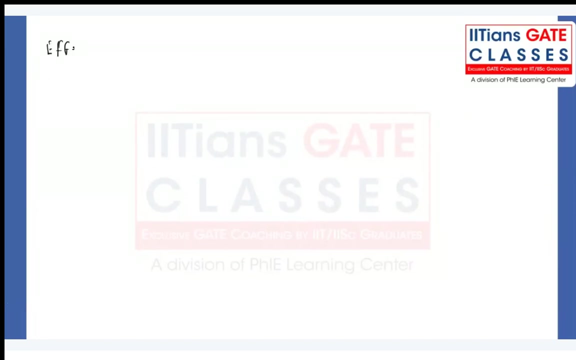 now, once it is done, let me know done. okay, so note down, uh, the effect of temperature and pressure on the viscosity of the temperature and pressure of the liquid. what are all? the effects will be there of temperature and pressure on the viscosity of the liquid. now, what will happen when i increase the temperature? 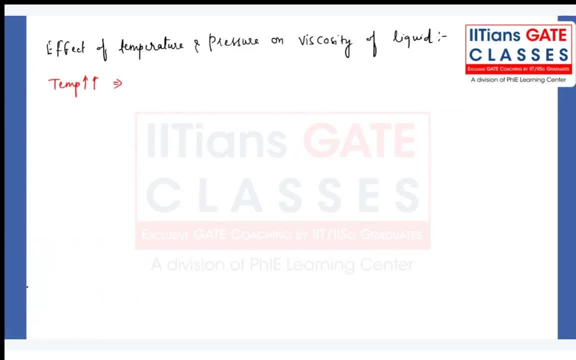 tell me, guys, whether, uh, whatever the cohesive force is there, that will decrease or increase. so viscosity of the liquid, viscosity of the liquid will decrease. now why it will decrease? because cohesive forces between the molecules. because cohesive forces between the molecules, between the liquid molecules, decreases. right, correct, whatever the bonding force is there, that will decrease and that will. 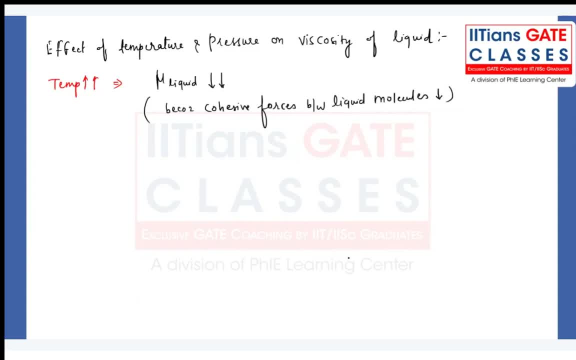 decrease the viscosity, right? so if viscosity will decrease, definitely flow will be very, very easy for us, right, the flow will be very, very easy for us. now, what will happen? uh, simultaneously i'm discussing for the liquid and gases. so, when the temperature will increase, what about the viscosity of the gases? 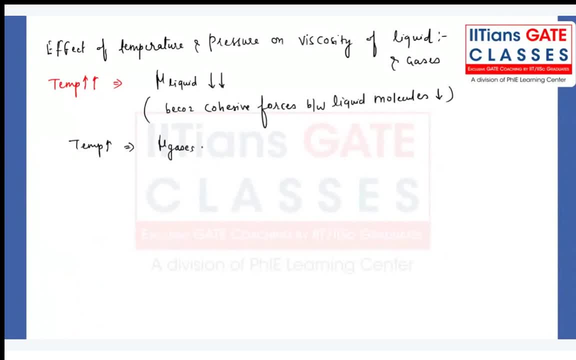 so basically, when you see that viscosity of the gases generally it will increase, right, because when i increase the temperature then molecular momentum exchanges will be very, very high, because molecular momentum now in a container when you try to increase the temperature, right, definitely you are trying to giving the energy to the molecules and the gases. molecules, they will. 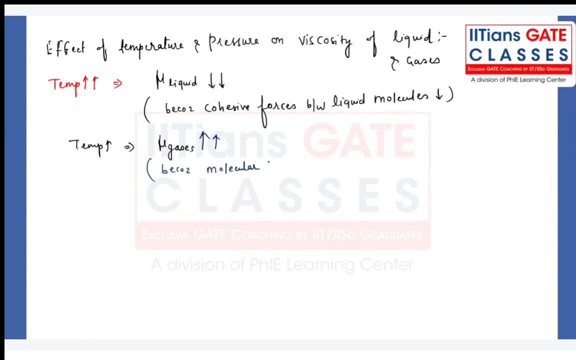 try to collide with each other. molecules, you know, and they will try to impart the uh, whatever the you know, whatever they have the velocities right. so definitely there's a lot of momentum exchange will be there and the viscosity of the gases will decrease, uh, will increase now because the molecule 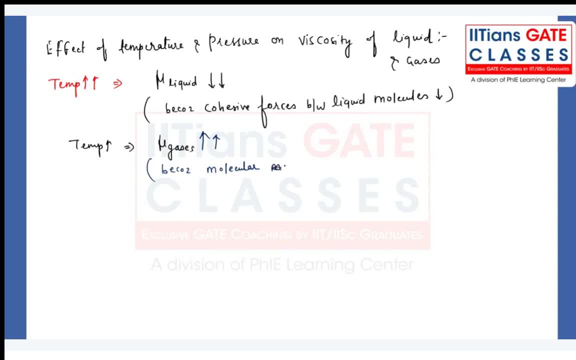 momentum, molecular momentum exchange will increase. what about the pressure? when i increase the pressure, what will happen to the viscosity of the liquid? so generally, viscosity of the liquid will remain same right. this is not to be fit about. you know, it's basically: there isn't any pressure. 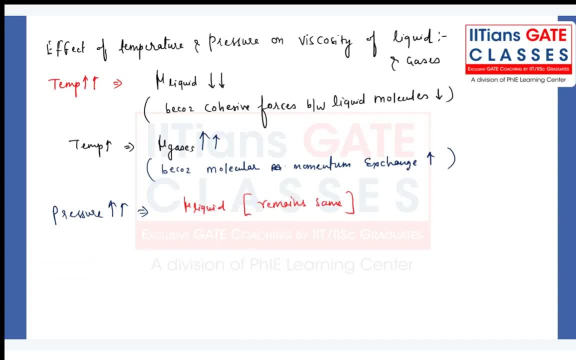 of the dah Straight truth now. so for us generally, this pressure, generally, remember that for a very, very one percent or 0.5 person, only 99 of the cases, the liquids are highly incompressible. right, even though you put elephant on that, you know they will not be getting compressed right, there will not be any chance of decreasing or increasing. 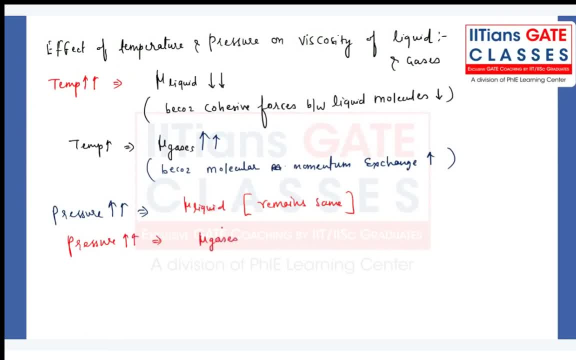 the viscosity of the gases. once again, that will be same or different. once again, it will remains same. once again it will remain same right why it will remain same? because molecular momentum exchange. molecular momentum exchange is directly proportional to root mean square velocity. right root mean square velocity will not be depending on the pressure. it will directly. 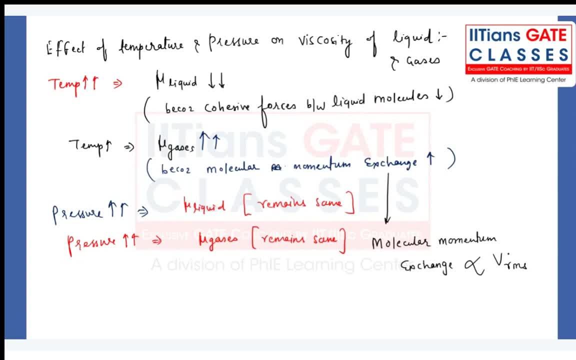 depending on the what temperature. remember that it will be directly depending on the what temperature, right? so if i write the formula of root mean square velocity, right, that will be 3 RT by m, so it is directly proportional to temperature, right? yeah, that is a kinetic energy, right? that is according to kinetic theory of gases and more. 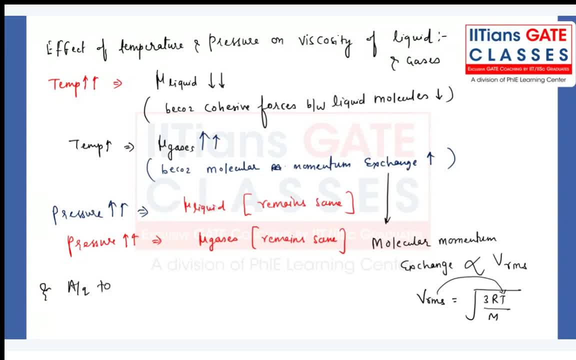 sources are suggesting that, according to kinetic theory of gases, according to kinetic theory of gases, that is for ideal gas. when you just apply, that is for ideal gas. when you just apply, that is for ideal gas. when you just apply, viscosity will be directly proportional to temperature and canametric viscosity will. 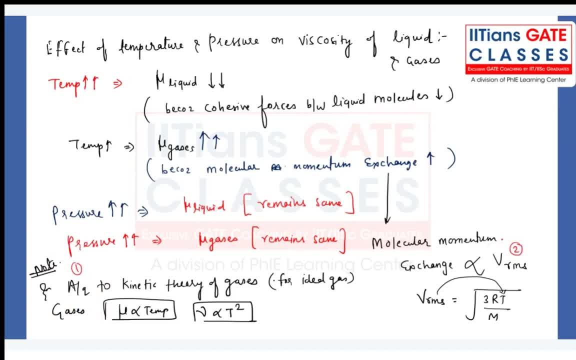 be directly proportional to ts. many talking about the gases make a note of it. so this is the another proof, one proof with this one second to be this one. so both the proofs are suggesting that it is independent of the pressure under root of- sorry, this will be under root of t and this will be 3 by 2. this has to be. 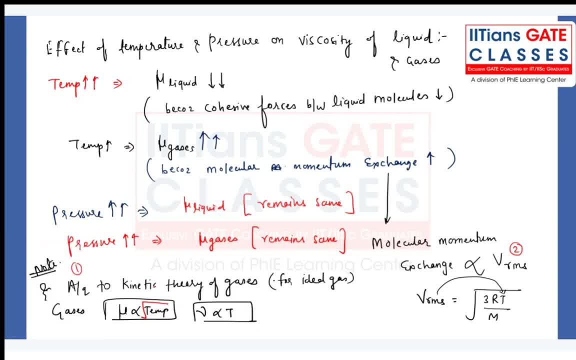 corrected. yeah, 3 by 2. whatever the randomness is there in the gases, that will be coming because of the velocity only and that velocity will not be changing because of the pressure. remember that that velocity will not be changing because of the. yeah, i will discuss. ravitej, i will discuss. 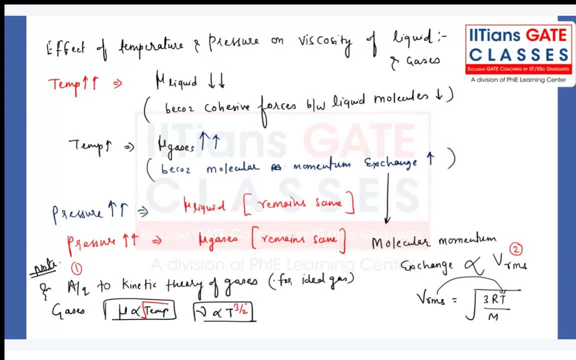 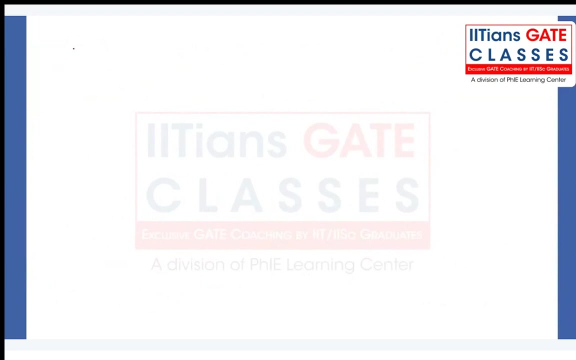 now. so whatever the momentum is, exchange will be there. that will be directly proportional to what temperature. that will not be proportional to what what we call pressure. oty, is it done for all now? so the next concept will be: if i increase the temperature, then what about kinematic viscosity of the liquid? 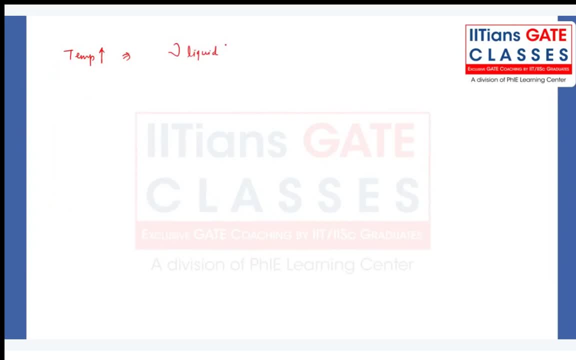 then what about the kinematic viscosity of the liquid, whether it will increase or decrease? So, when you think of this one, this particular case, what you are observing, mu by rho, right. So mu of liquid is decreasing and the liquid case when you increase the temperature. I am not. 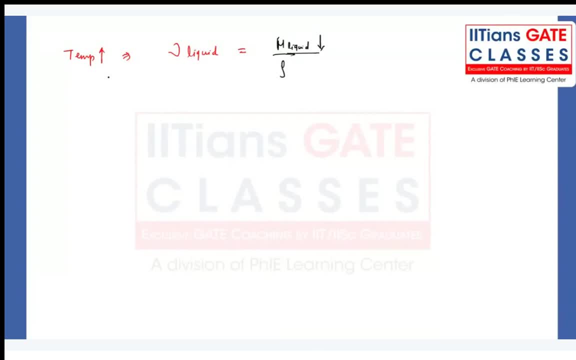 talking about the water. For a very general case, we have observed that for a fixed pressure, for a fixed pressure value, when I increase the temperature that means I am fixing my pressure value. So what you are observing at a very, very low pressure, then what will? 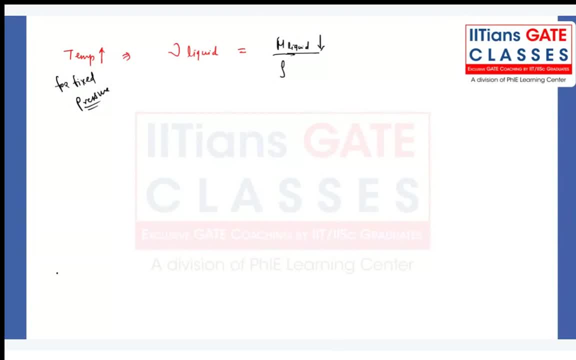 happen, The density will also decrease. right Then, what you are observing from here. So we cannot say about this one right, We cannot say about this one right. So we cannot say about this one right, We cannot. 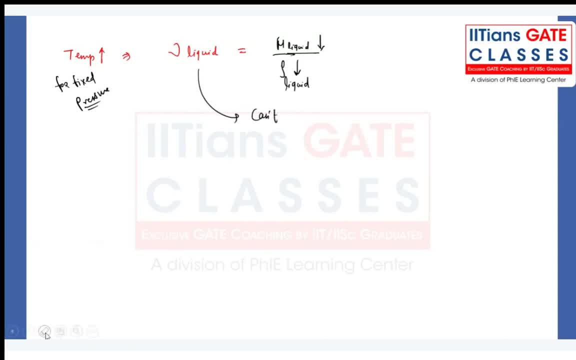 say the kinematic viscosity of the liquid. We cannot say exactly what is happening with the kinematic viscosity of the liquid, But in generally it has been found experimentally that kinematic viscosity of the liquid slightly decreasing on increasing the temperature. Yes, yes, Because anyway, effect of density. you know, whatever the effect of density is, 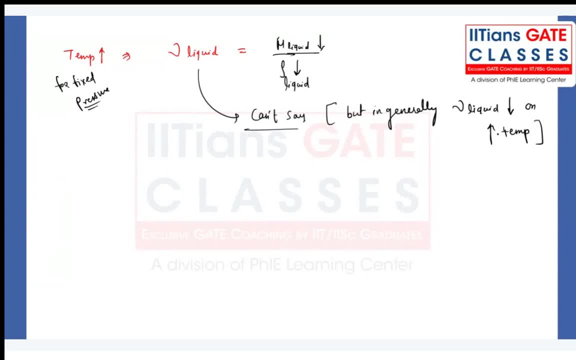 there. hardly any effect is there, right? Hardly any effect is there on the density changes when you try to increase the temperature. So it totally depends on the dynamic viscosity right Now, the density difference of the liquid. the density difference of the liquid. 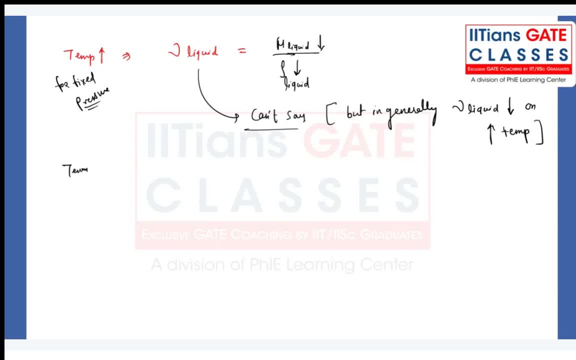 we can say the temperature will increase. then what about the kinematic viscosity of the gasses? Then what about the kinematic viscosity of the gasses? will it increase or decrease? So for that we have to write Rho of gasses. So automatically, this is: 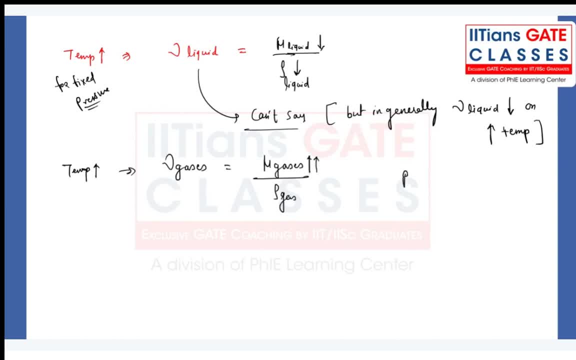 increasing and density of the gases is what. P is equal to Rho RT. right For a fixed pressure, for this one is to be fixed one. This will be equal to Rho RT. So this one is to be be what inversely proportional. so when i increase the temperature, the density will be what decreasing. 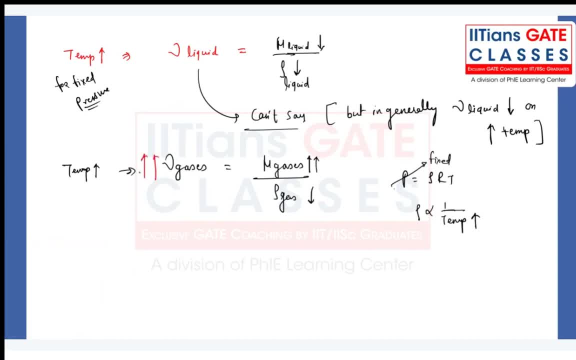 so both are contributing to increase rapidly the kinematic viscosity of the gases right further. my different, uh, the pressure value. when you increase the pressure, what about kinematic viscosity of the liquid? tell me guys, yes, when you try to increase the particularly, you know mu by rho mu of liquid. 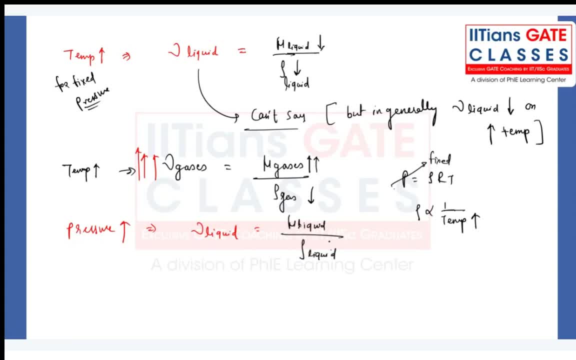 by rho of liquid now, but have to very careful. the pressure does not. basically what increases or decreases the density of the liquid. it is incompressible, right? no change. maybe any changes will be there. that is 0.5 percent, right, and this will also be no change. so what we are observing? no change. 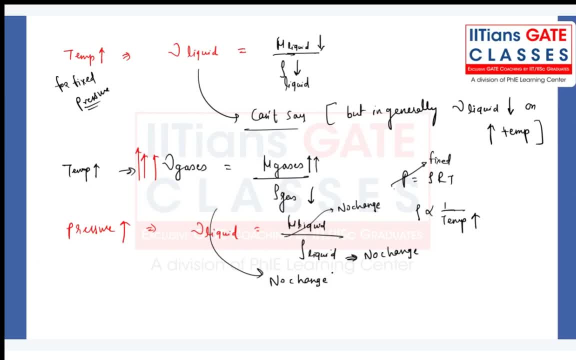 right, correct. what about the? yeah, perfect, what about the? when i increase the pressure value, then kinematic viscosity of the gases- mu of gas, by rho of gas, mu of gas- is what increasing or decreasing for a fixed temperature? when i just increase the pressure value, my, uh, my dynamic viscosity is increasing or decreasing? tell me guys. 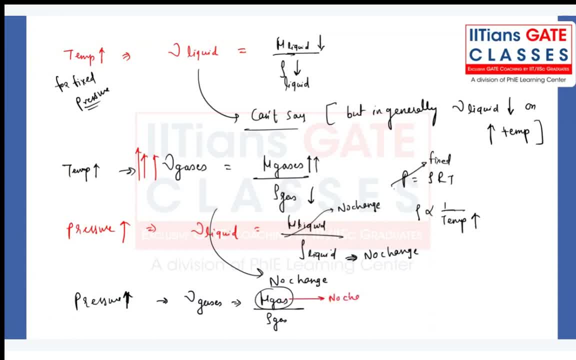 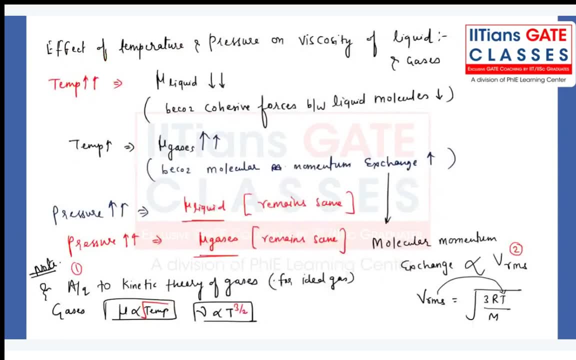 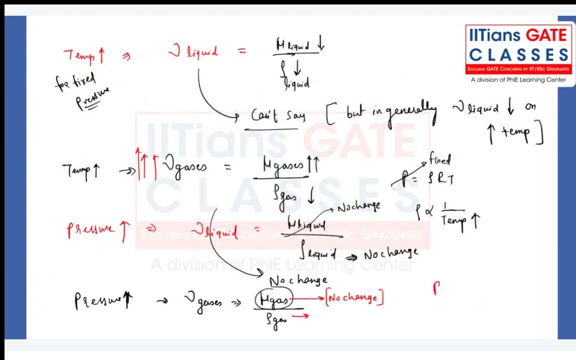 this is to be what? no change. once again, as we have discussed earlier, also as you can see here, that kind of that dynamic viscosity of the gases will remain same right. so here also it will be no change further. what about this one for a fixed temperature? pressure is what directly proportional to density? 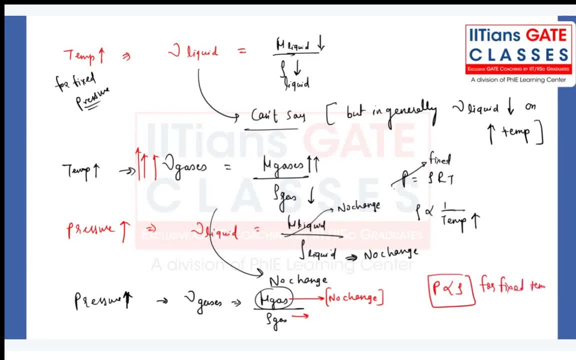 for a fixed temperature, right, so what we can have, this will increase so further. it will decrease the kinematic viscosity of the gases, right? make a note of it. so whenever we try to do the any experimental kind of thing, we try to vary only one parameter, right? we? 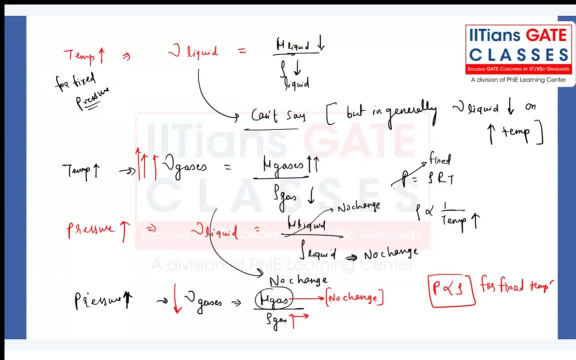 don't vary both the parameter. now you have the while thinking, sir, when, what will happen when i change the pressure and temperature both? then again it is very difficult to predict and you can't perform the experiment. also, getting my point, all of you, because some of these friends, again, they will waste the time after the class. they will be start. 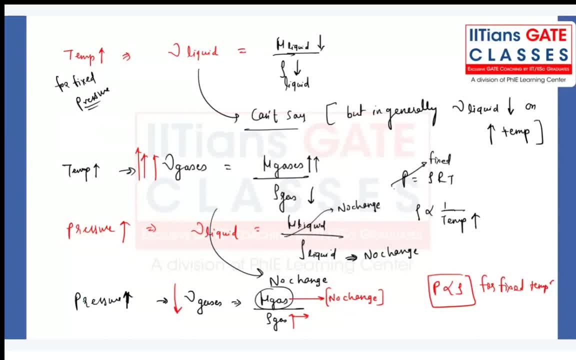 thinking: you know, uh, in a special, in a spacious world, that sir, what will happen when i increase the pressure, decrease the temperature, decrease the pressure, increase the temperature, and they will start playing like that. so please don't do that. give a point, or not? all of you? these are all i'm telling you based on the experience. 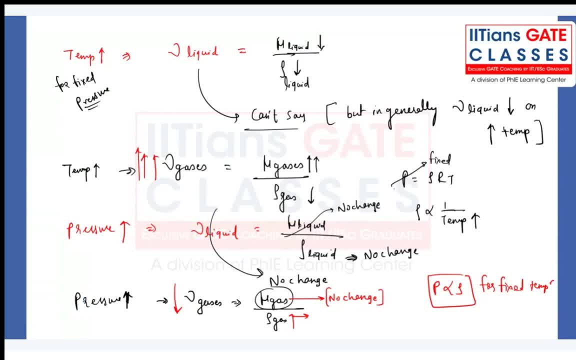 basically what experience which is being faced by these. you know, students, so try to stick with the content which i'm telling you regarding fluid mechanics. that will be more than sufficient for a good exam. so, um, now i have understood. the topic, which is whish, is very interesting to me. 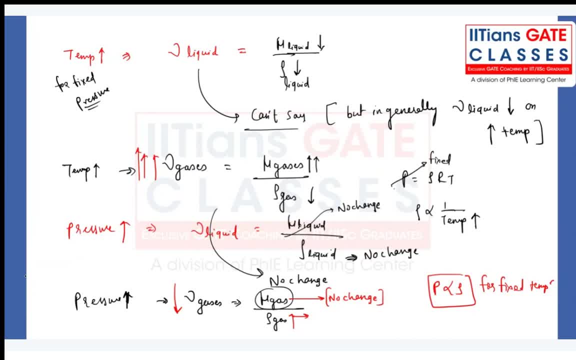 because at the initial phase of the preparation you know you can think of topic, you know you can have some imagination, some thinking. but after certain point of time, when the time will be passing and when the july or maybe august month will be coming, you cannot invest that much amount of time in theoretical portion. lot many subjects will be there, right? 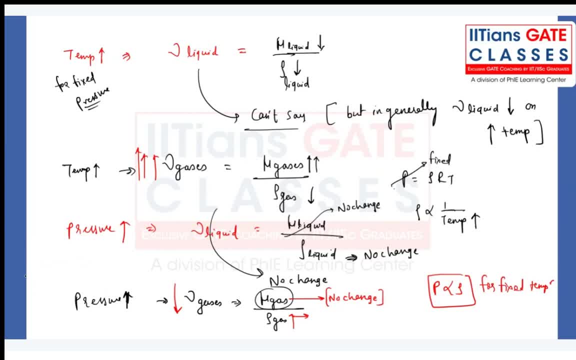 again the student will be start getting pen. i know those times and some of them will be start demotivating and they will leave the preparation and they basically what. coming again back to uh, in the month of what? the summer and january, with the so much of expectation that i will be getting good mark. but 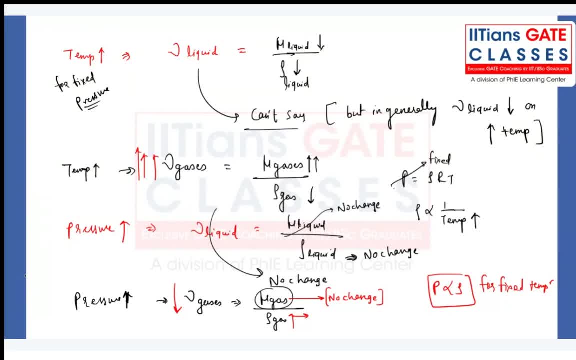 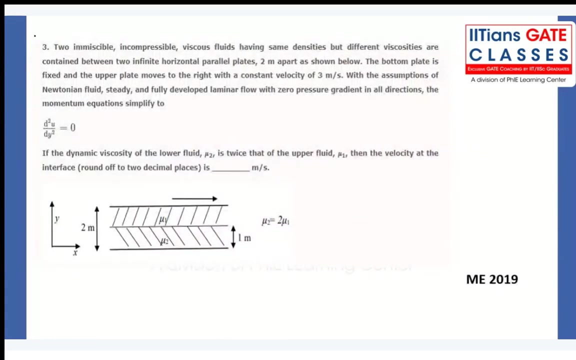 practically that is not going to be possible. now, is it done for all? can i move to the next one? done? no, how many of you have tried that particular question which i have given to you, this one? anyone got the answer for this question now. so what they are asking? what is the velocity at the interface of the, you know, flow condition? 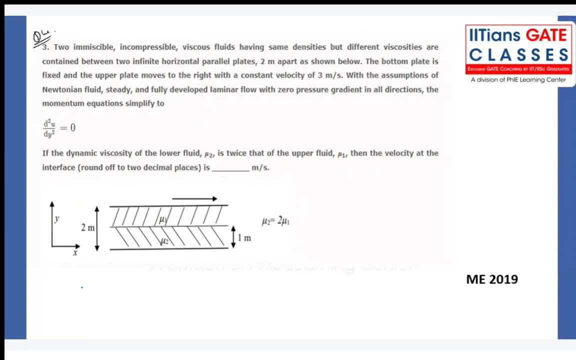 which is being imparted. anyone has tried this one. so when you see this one, they have directly given the uh two immiscible, incompressible viscous fluids having same density but different viscosity, contained between the two infinite horizontal parallel plates, two meter apart. the bottom plate is fixed and upper plate. 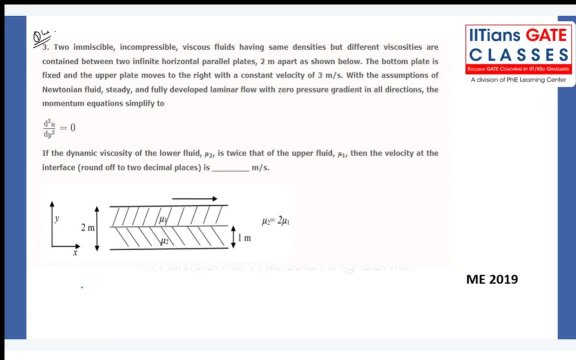 is moving with the velocity called uh. three meter per second correct. one meter per second is correct with the assumptions of the newtonian fluid is steady and fully developed lambda flow with the 0 pressure gradient in all the directions. the momentum equation simplifies to be d square. 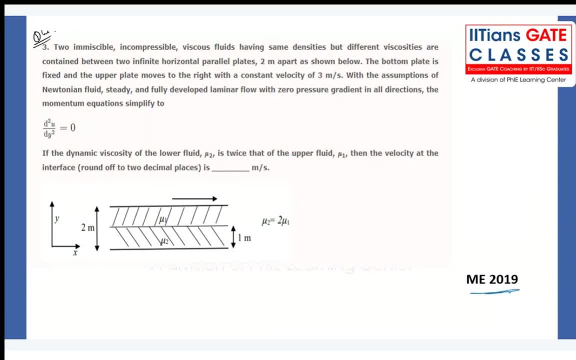 u by dy square. now when you see this question they have asked in gate exam in mechanical fusion 19. but this question has directly taken from singelle. you know unsolved. when you see the lambda flow or the navier stokes equation In that particular chapter, whatever the unsolved is there directly. they have copied from there. 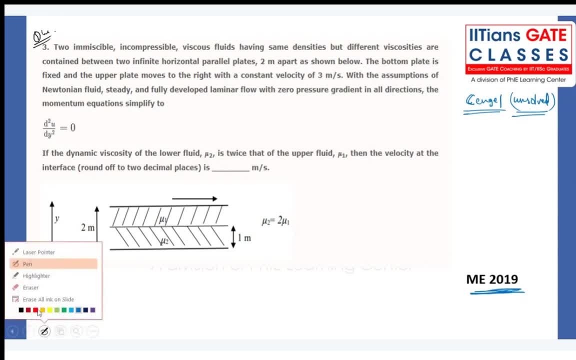 So we have to follow certain standard test book so that we will be directly getting the question from there itself. So what is the meaning of this? When I do the double integration after double integration, I will be getting: u is equal. 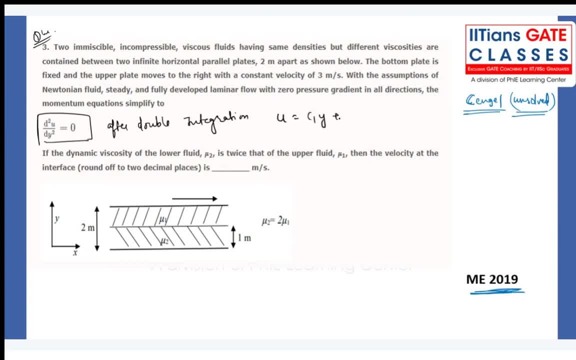 to c1y plus c2.. That means u will be varying linearly. That is what they want to tell us. Now, when the u is varying linearly, my dear friend, then how will be the velocity profile for that? So when you just look at this mu2, lower fluid, which is having the viscosity twice, 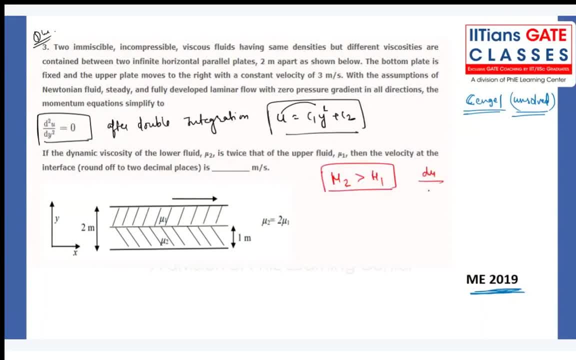 that means, whatever the du by dy will be there, the velocity profile for the second case will be lesser than that For the same amount of save force, For the same amount of save force or the viscous save force Now. so definitely second fluid will be having less velocity gradient as compared to the 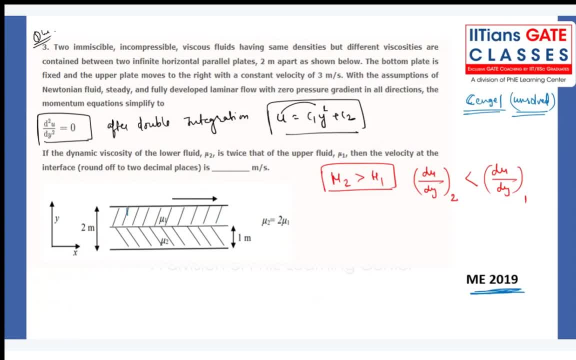 first one. So what we can have. We can draw the velocity profile something like this: Now make a note of it. This will be theta1.. This will be what Theta2.. This is what. Sorry, this is theta2.. 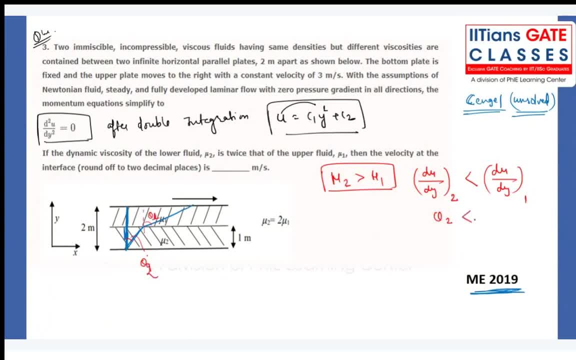 This is theta1.. Theta2 is what? Less than theta1.. When you observe from the vertical, that is being observed. But the question over here is: what is going to be happening, right, What we have to find? We have to find the interface velocity, right. 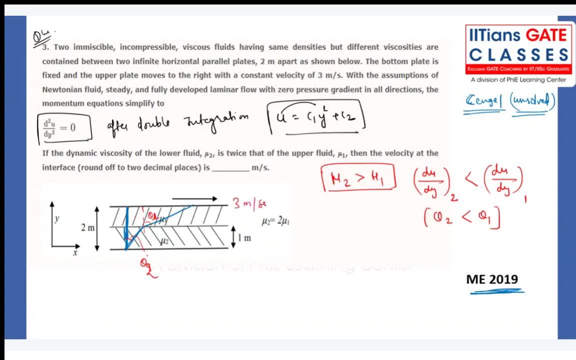 The top plate velocity has been given as 3 meter per second. So what we have to do. So, when you draw the free body diagram of the mid plate, When you draw the free body diagram of the mid plate middle, or basically what, 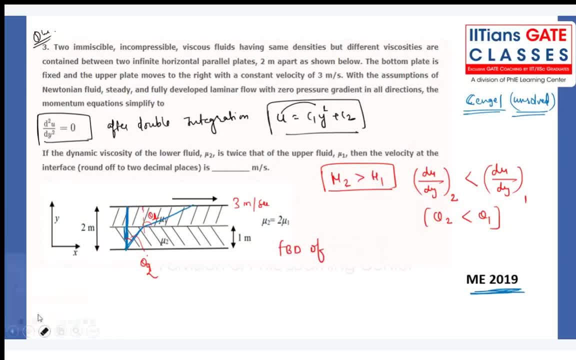 When you draw the free body diagram of the interface. so draw the. basically what? Draw the free body diagram of this particular interface, So what you will be getting? Yeah, that is correct, Based on putting the boundary conditions. You can get the answer from there itself. 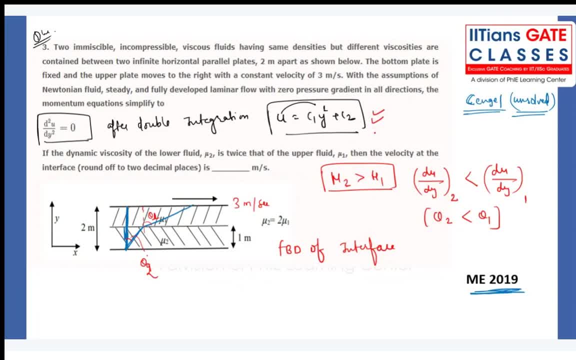 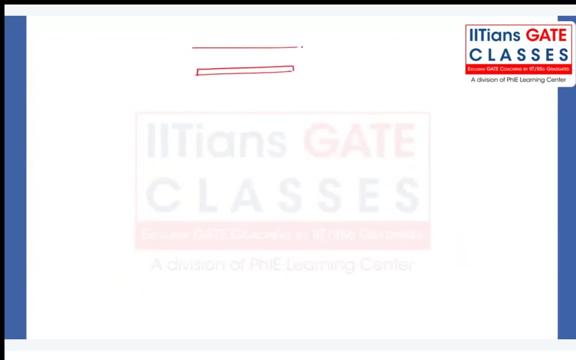 Getting my point, But I am telling you some other way through which you can get the answer once again right. So here, free body diagram of interface when you draw this one. So I am drawing over here mu2b1.. 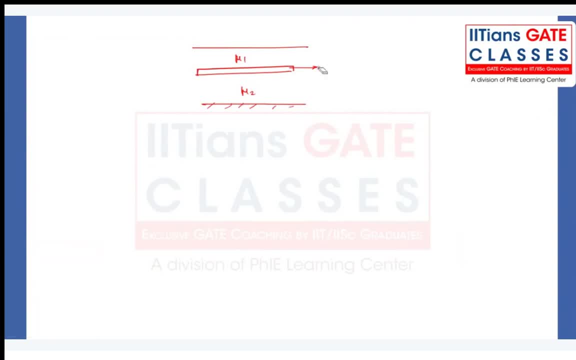 This is what, Sorry, We are applying the forces onto the top plate. What the interface will do? It will try to apply some kind of force in this direction. right, And I told you, whenever we have the linear velocity profile, whenever we have the linear 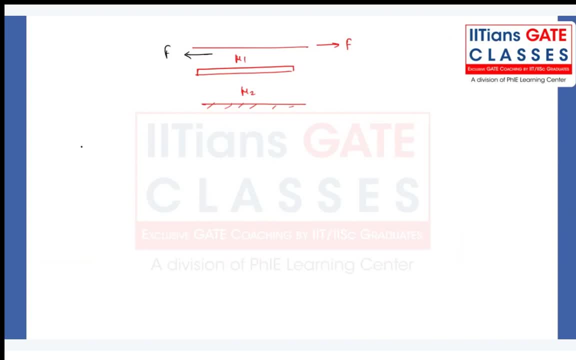 velocity profile. always remember: each and every fluid layer will be subjected to same kind of shear force. And what about this plate? Plate will offer force in this direction And you also know that, my different, you also know that fluid is not accelerating that. 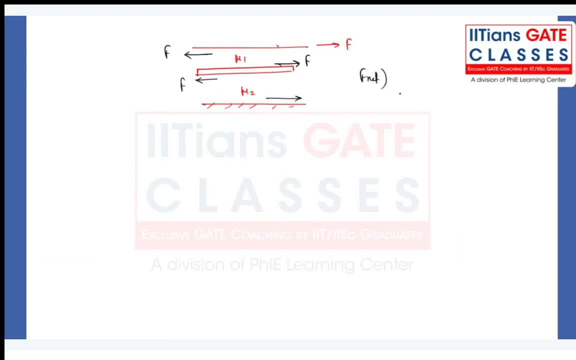 means the net force in the direction of motion. Yeah Yeah, In the engineering mechanics we have done right Newton's second law: The net force in the direction of motion is what Mass into acceleration? And for this particular plate, for the middle one, what you are observing? 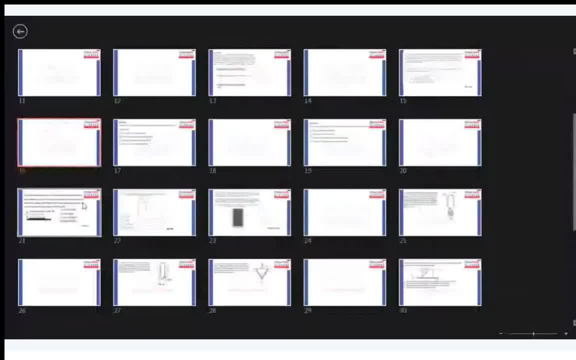 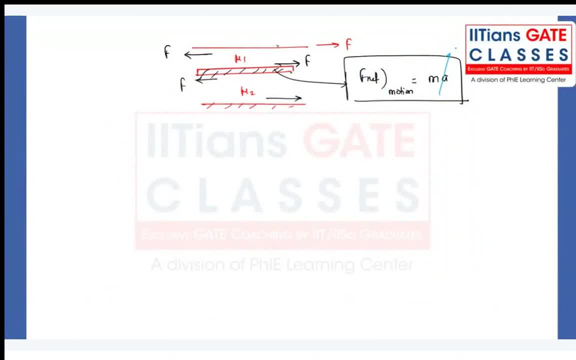 You just think it like a plate, interface plate or maybe intermediate plate. What you can have, Tell me guys, Acceleration is zero, because every fluid is what Moving with some constant velocity. Then what we can write This F1.. Whatever is there, let's suppose F1 minus F2 will be there zero. 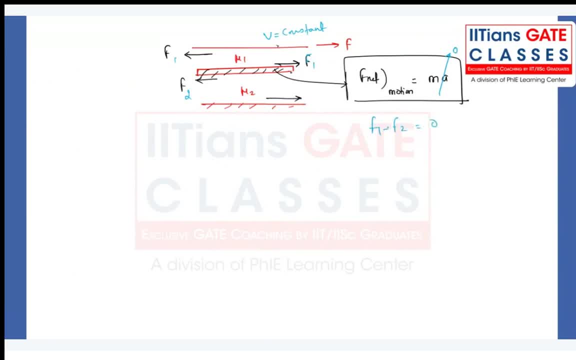 Then what about F1?? What about F1 and F2?? How to find that? What is the formula for the viscous force Mu into du by dy into area. Getting my point: F is what Tau into area right. 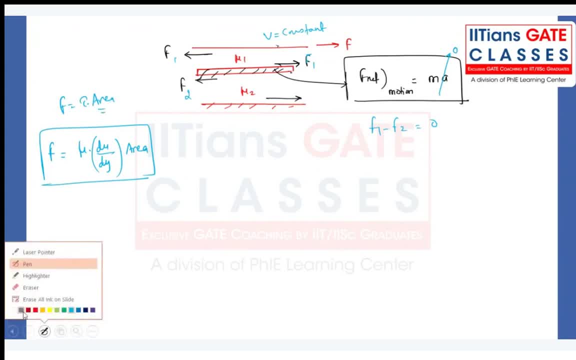 Getting my point Now, what we can draw, my different, What we can find out, the F2 value, F2 value, we can easily find it out something like this: Let's suppose this is the interfacial velocity u, this is v, three meter per second, and this: 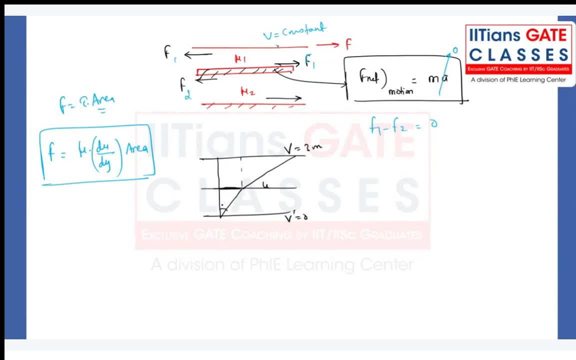 is zero, right. So what we can write, What we can write, my different Force 2. we can write Force 2. we can write what Mu into du by dy into area, Du by dy of second fluid into area. What is the area? 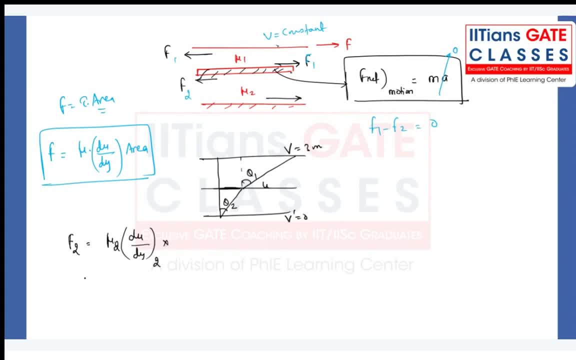 Let's consider the area to be what, What they have mentioned, the area Area I can consider whatever the width will be there, Width, I can consider it as 1, and the length of the plate to be, let's say, L. right, And what about force 1?? 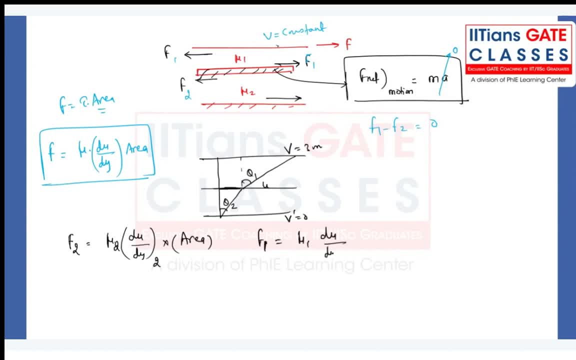 Force 1 will be mu 1 into du by dy. for the second, for the first, fluid into same area, into same area. Okay, So what about force 2?? Mu 2 into du by dy will be what u tell me, guys. 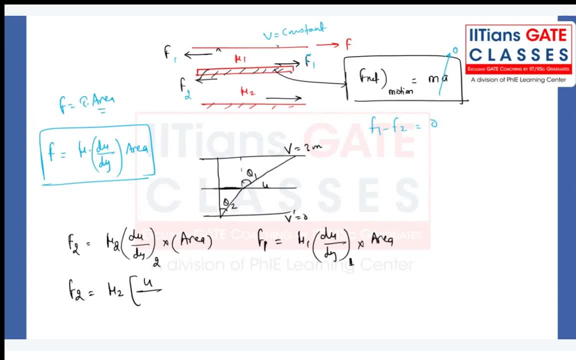 u divided by what Gap? What is the gap between the plate 1 and 1 into area? And what about force 1?? This is the total velocity, right, And this is what Intermediate plate velocity. Then what about this one? 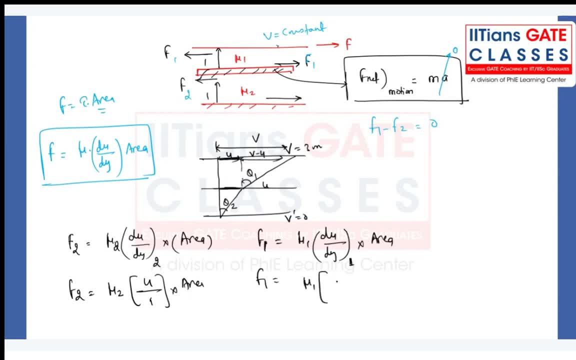 v minus u, So mu 1 into v minus u, v minus u by 1 into area. Now try to equate f1 minus f2.. f1 is equal to f2.. So what you will be getting, my dear friend. 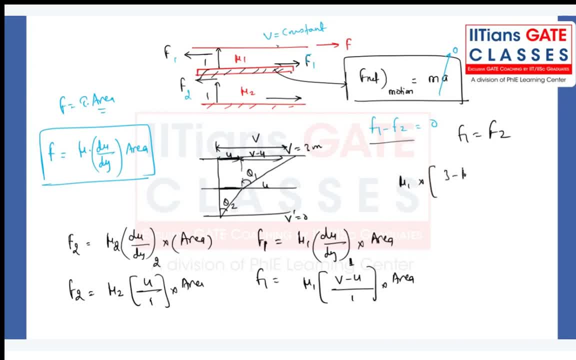 Mu 1 into what? 3 minus u divided by 1.. That is, mu 2 into u divided by 1.. Mu 2 is what They have given, 2 times of mu 1.. So what we can write: 3 minus u. 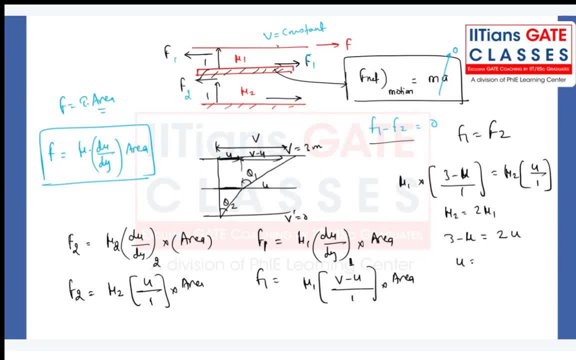 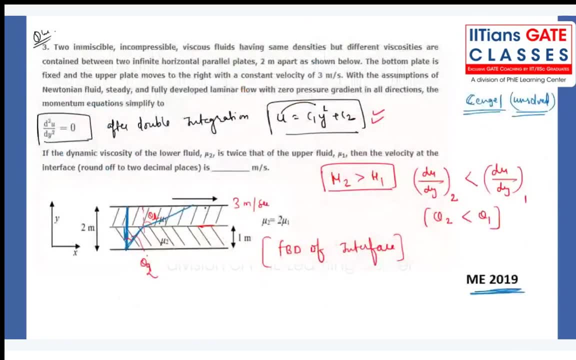 That is 2 times of u. So what we are getting? 1 minus u, That is 1 meter per second. When you draw the velocity profile to be something like this, This is wrong. When you draw like this, they will not be having a constant slope. 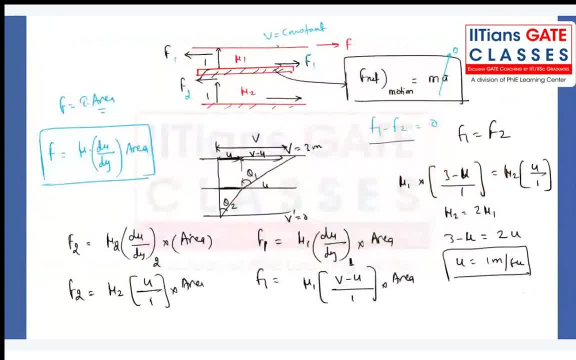 Remember this is wrong. right, They will be having different, different slope, because I told you, for the same CFOs viscosity will be inversely proportional to the? u by dy. Higher the viscosity of the fluid, lower will be the tendency to flow easily. 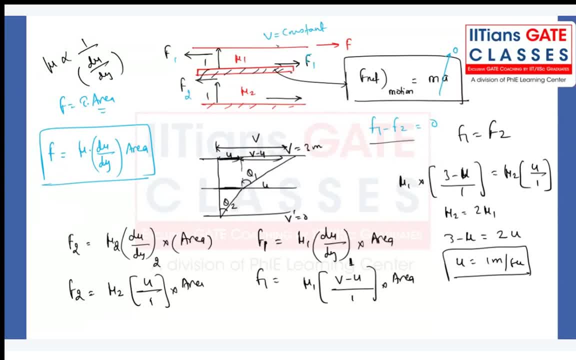 all of you are getting my point. so this is what they have given the equations. remember we have to write f1 right, mu 1 into theta 1 into what area? theta 1, dot d, theta by dt right. basically we used to write slope rate right, not d, basically. 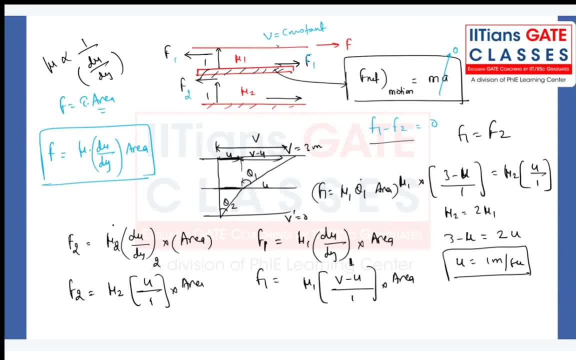 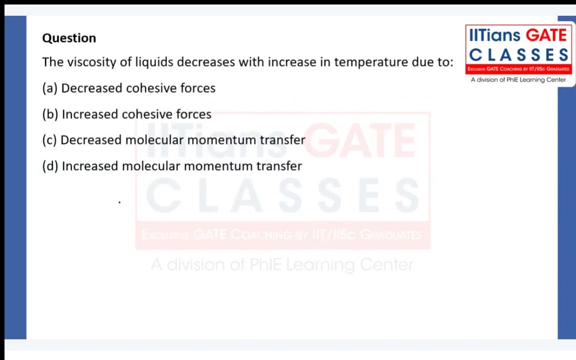 exactly the slope right, because exactly, uh, without rate, that we used to write in case of solid, but this is a fluid, so d theta by dt will be coming, getting my point, all of you. once it is, let me know. Can I move to the next one? No, So again, this is a very simple question. 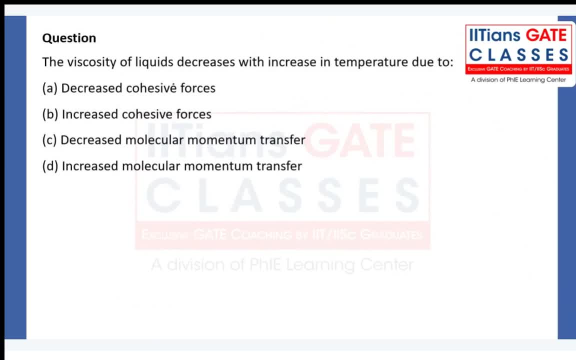 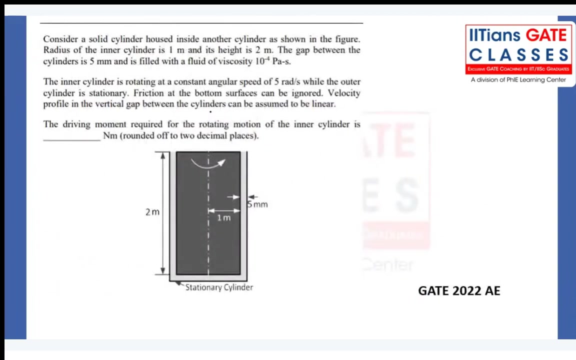 The viscosity of the liquid decreases with the increase in temperature because decreased the cohesive force. Yes or no, guys? Yes, This, we have discussed, This also we have discussed. Now try to solve this question. No, again, you will say that chapter number one is not that important for the aerospace. 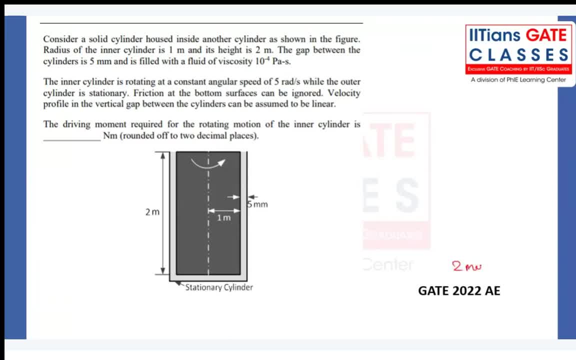 But what you will say when they give out two marks? Again, sir, again you will answer me back. That's how I will leave this question. How many questions you will leave like this? So you have to prepare. When the things are very simple, you try to prepare, Don't skip. 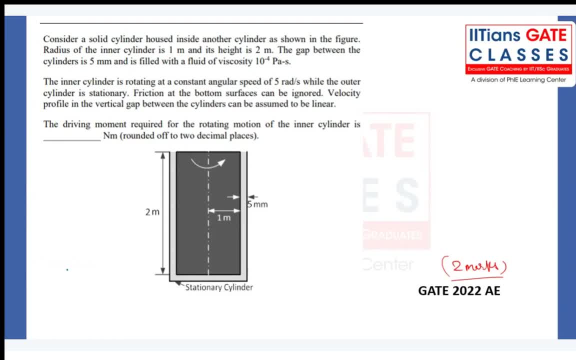 that. Put some effort, Definitely you will be getting the answer for that question Simply leaving that- sir, I am not going to study that because it is a very tough topic- Then definitely you will not be getting a good rank, Because if you are not working hard, 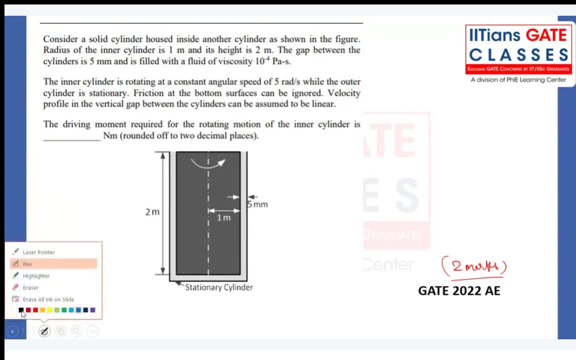 definitely someone is there who is working very hard. So whether you will be in the 21st century, 22nd century or maybe 30th century, competition will always be there. Consider a solid cylinder housed inside another fixed cylinder right This outer cylinder. 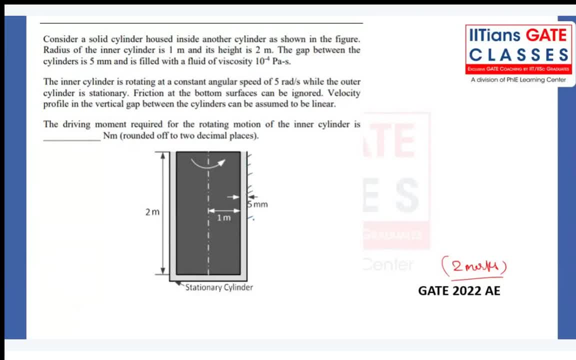 we might be thinking of. This is a fixed one. for example, Now, as they mentioned also stationary cylinder, The radius of the inner cylinder they have given as 1 meter and the height they have given it as 2 meter. The gap between the cylinder is filled with. 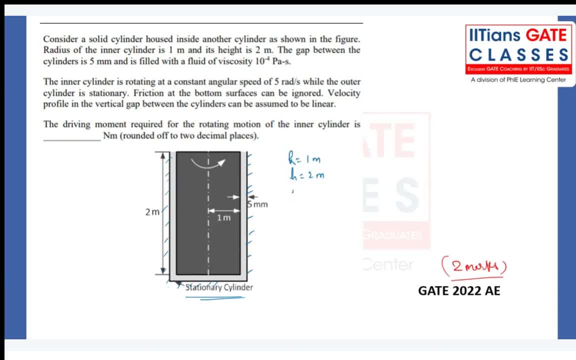 the the gap is. they have given what The gap, they have given as 5 mm, with the viscosity 10 to the power minus 4 Pascal. second right, The inner cylinder is rotating at the constant angular speed, Omega, that is 5.. 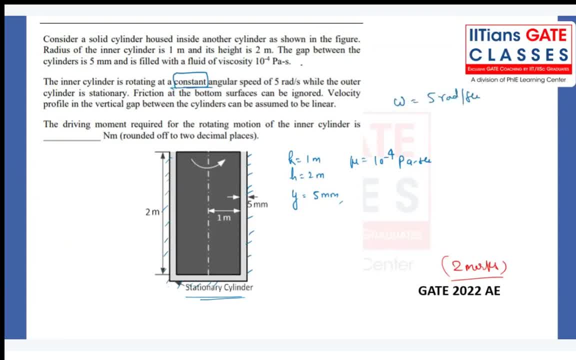 That is 5 radian per second. While the outer cylinder is stationary, the friction at the bottom surface can be ignored. That means there is a very good meaning in that. The friction at the bottom surface, that means this one: The friction see the fluid is. 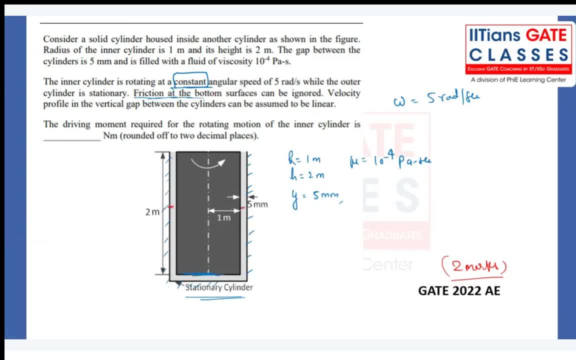 there, here also. The fluid is here also. is there right? So definitely we will be having the linear velocity profile like this, But the fluid is here also. But they have mentioned in the problem very clearly that we have to neglect that This bottom surfaces Right Only we have to consider this side one. 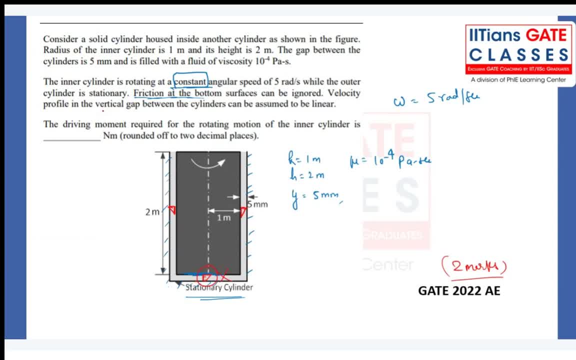 The velocity profile in the gap. that is the correct answer: The velocity profile in the vertical gap. they have clearly mentioned that linear one When they mention already they mentioned that linear, So we have to assume the linear velocity profile. They are asking what the driving movement required for the inner rotating motion of the cylinder. 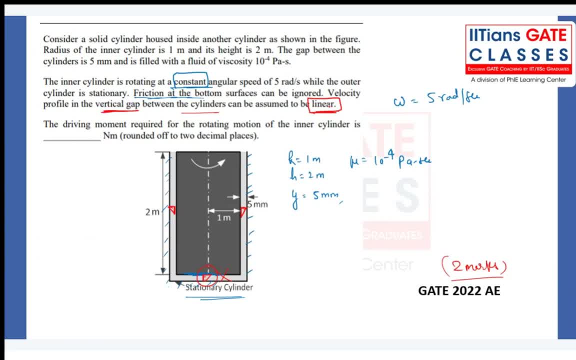 in Newton meter right. So once again we have to determine the torque, How much of torque I need to apply right. so make a note of it first of all, then we will discuss so very first of all. everyone know that the fluid is there. the fluid will offer some kind. 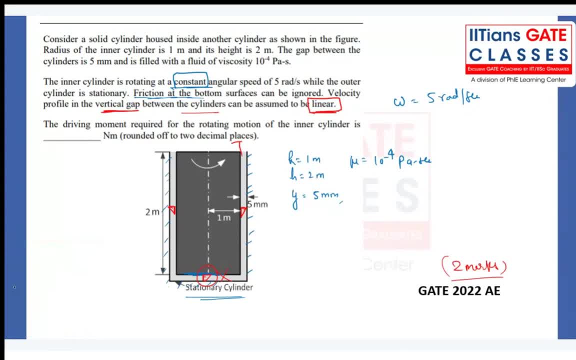 of resistive force and to avoid or to basically balance that resistive torque. you know we have to apply some external torque so that it can be rotated. you know, otherwise, definitely, how much amount of power i will give. you know, if i use a less amount of power, not equal. 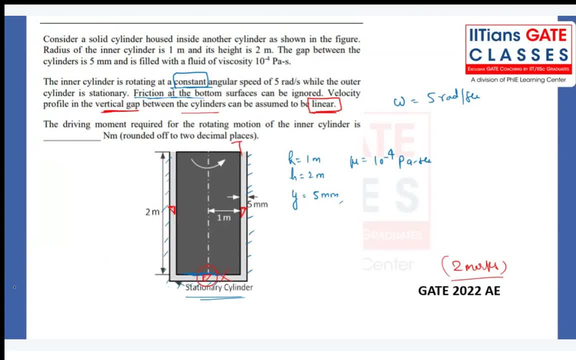 to resisting power, then what will happen? we may not be able to rotate that cylinder with the constant angular speed, right? so yeah, so the net torque must be equal to y into alpha in the direction of motion, but we know that i into alpha angular acceleration, that is. 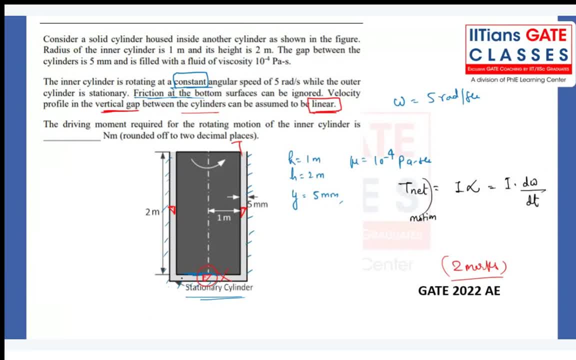 d omega by dt. i believe that engineering mechanics, they have covered this one now. now omega is what constant omega is. constant means what d omega by dt will be zero. the net torque means what applied torque and in the opposite to the direction of motion the resisting torque will be acting. that equal to zero. so applied torque, whatever we have to find that. 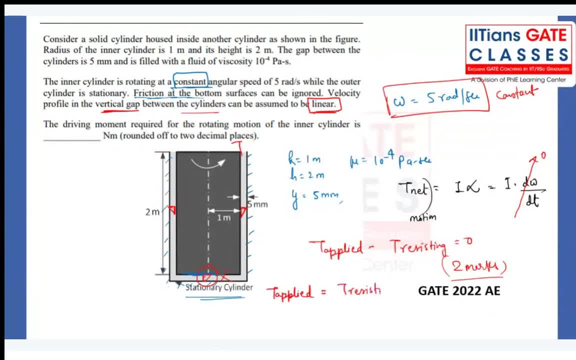 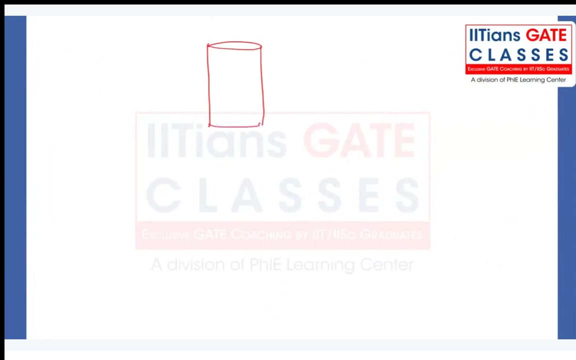 should be equal to resisting torque. that should be equal to resisting torque. that is our very, very, very, very first thing that we have to understand now. make a note of it. now you try to understand what i'm telling to you if i draw once again cylinder and when you just look at very carefully this one. 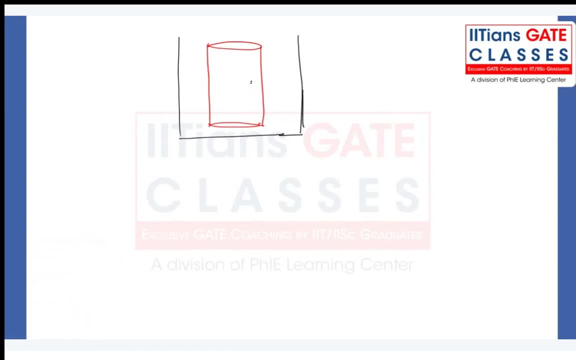 what you are assuming that here, that whatever the gap is there, right, we are assuming the gap to be whatever the gap is there, that gap is a linear velocity profile and what we are thinking about certain this case, what you can think of some the case is, if i draw the 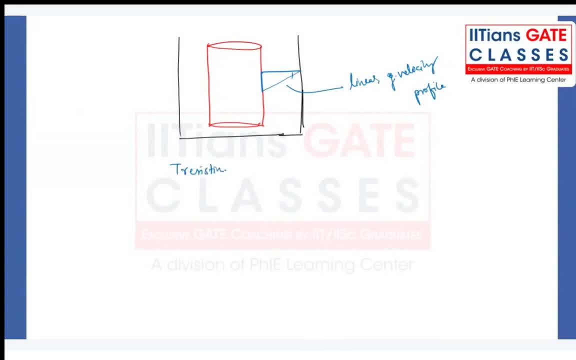 and what you can think of some. the case is, if i draw the resisting torque, what is the formula for the resisting torque force into radius now, what is the force, what is the resistive force? mu into du by dy into area, into radius right. but the big thing, the big question mark over here, is that we have to understand there. 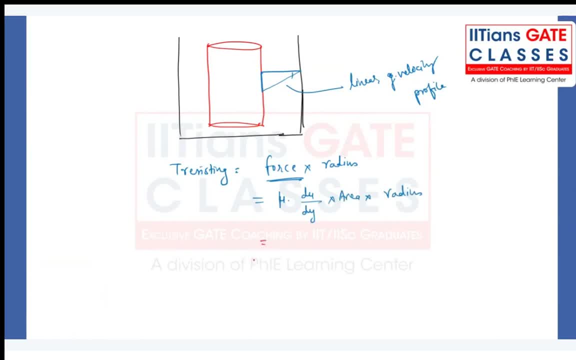 is a linear velocity profile, my dear friend. so you have to understand, we can write the linear velocity profile, my dear friend. so you have to understand, we can write. we can write v by h, whatever the gap is there. v by y being right into area. what is the area? 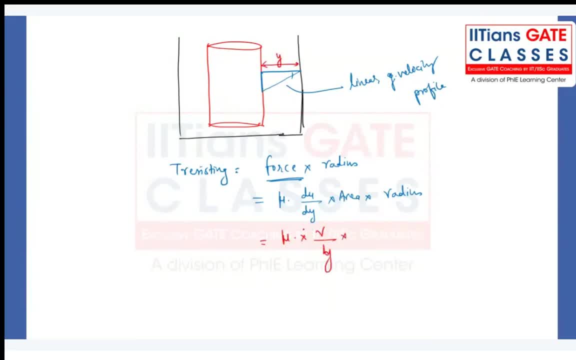 on which it is acting. what is the area? my different, it is acting on a complete length of that cylinder. what is that? 2 pi r into l. that is the area on which the, this liquid, is offering some kind of resistive force. so what? we can write 2 pi r1 into l and the radius. 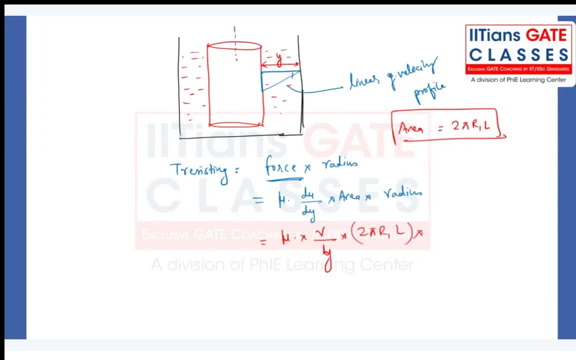 will be what, my different, we are have to take the movement about this one. then what about the air movement? radius, that will be once again r1. but the big question, but the big question mark over, is that: do we need to perform any kind of integration? no, right, because radius is not. 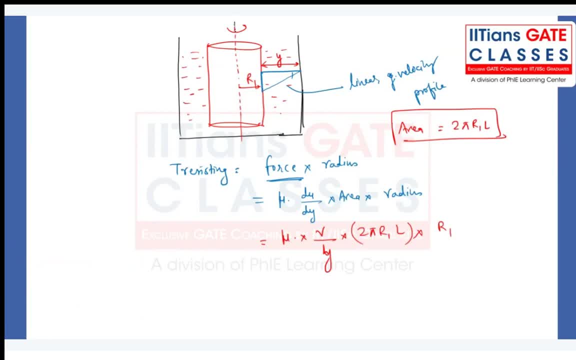 changing when you look at from the point of rotation. this is the point of rotation right, this is the center for rotation. center of rotation and we have to take the movement about center of rotation for every fluid layer is having the fixed radius, a radial distance right. fix the radial distance, so we need not to perform any kind of integrations. 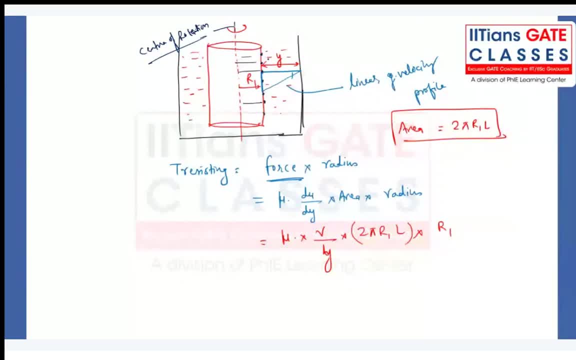 right, we need not to perform any kind of integration over here, right? remember that. so that's why we are taking this one now again. area, you might be thinking, sir area, we can consider 2 pi r1 into l, 2 pi r2 into l. that also can be considered, sir 2 pi in a better sense, sir it. 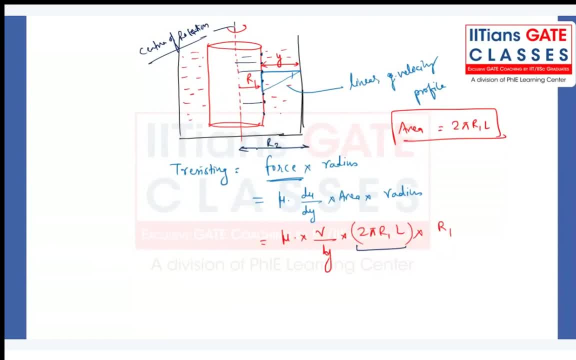 should be 2 pi r2 into l. for the كل Además 7, it should be 2 pi r2 into l. for theних times, r1 plus r2 divided by 2 into L. Frankly speaking, that should be the value, But they have given the. 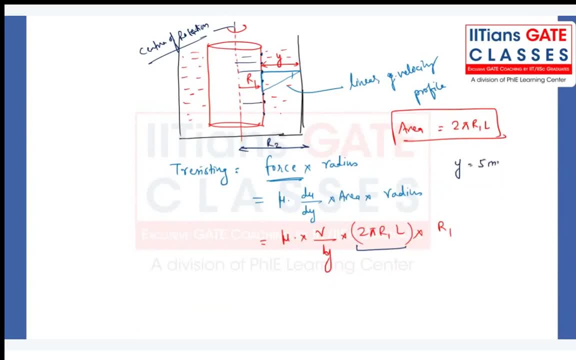 gap very, very small, even though you try to put the value of r2.. What is that r1 value? What r1 value? they have given 1 meter right, 1 plus 5 mm right. When you add it, you will be. 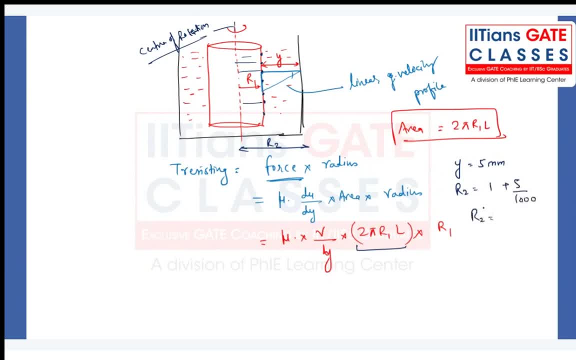 getting very, very low value right. It is almost equal to r2. equal to what r1.. So directly, I can write 2 pi r2 into L, or I can write 2 pi into r1 into L. The result will not change right. 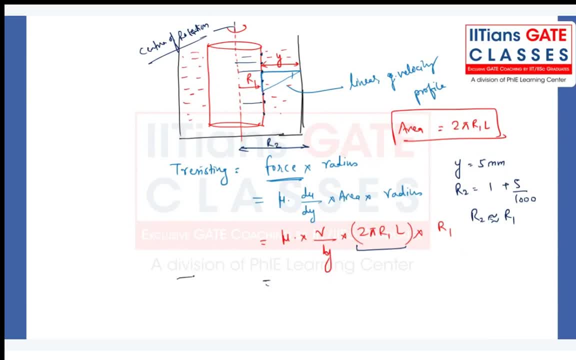 So now, when you just put the value, this will be my applied torque, That will be my resisting torque, That is, mu into V will be what r1 into omega Inner cylinder is rotating with the speed of what r1 into omega, divided by gap, 5 into 10, to the power minus 3, 2 pi. Once again, r1 is 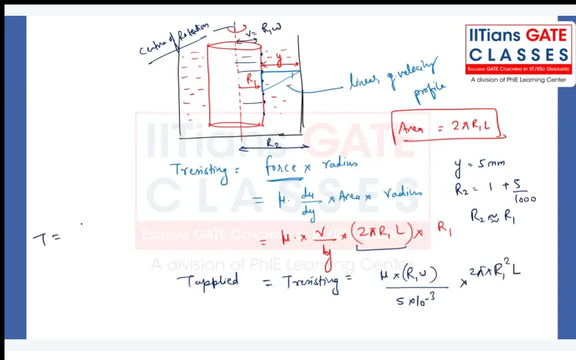 squared into L. So what will be my applied torque? Mu is what? 2 into sorry. What is the viscosity value? 10 into 10 to the power minus 4.. r1 cube: 1 cube Length will be what The length they have given. height is given what? 2 meter. 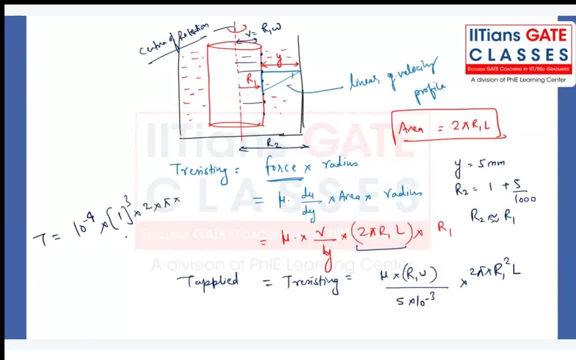 What is that value? 5 into what? Omega? What the omega value they have given 5 radian per second divided by what? 5 into 10, to the power minus 3.. Check it out. All of you are getting the same equations. 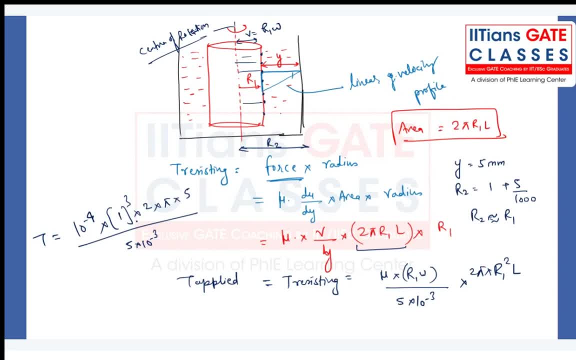 No, but anything we are missing over here. See, there is a 2 pi into 2 will also be there right Into 2 will also be there. Why? Because 2 pi r1 into L is there right And already we have omega value. that is also. 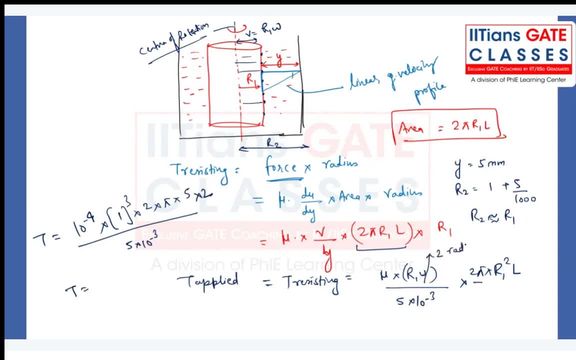 equal to 2 radian per second. Both times will be there. So if you just multiply the answer with the 2,, so you will be getting 1.256. Newton meter, or you can write 1.26 Newton meter. 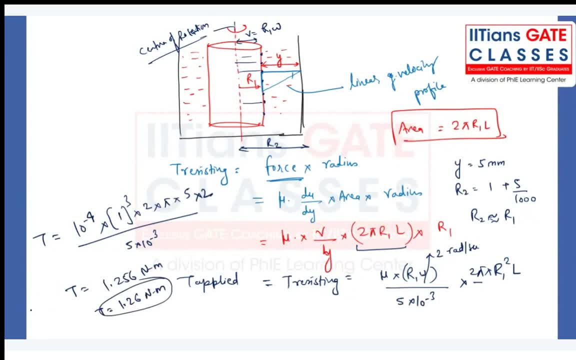 As I discussed in the WhatsApp group. you know I have given the similar kind of problem There. they asked basically the viscosity of the fluid by giving the applied torque. I am asking you, when they have not mentioned anything about the linear velocity profile? 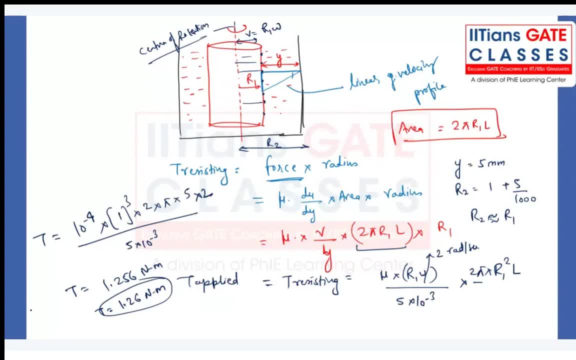 then, what about the velocity profile? When they mentioned nothing about the velocity profile, Tell me guys. Well, when they mentioned nothing about the linear velocity profile, you want to know the velocity values. Well, to get the velocity value, you have to use the K per second right. 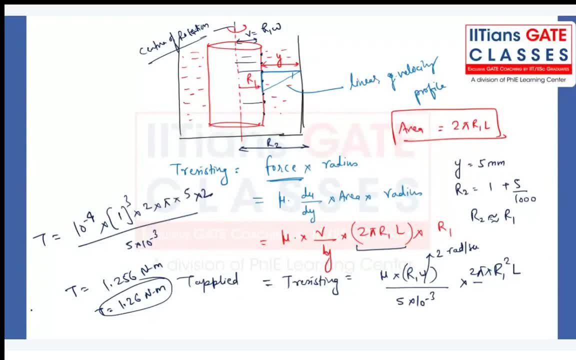 Yes, And if you do that, then the velocity of the fluid is now the velocity of the fluid. Now we are going to talk about the system in which the number of things are going on. What we're going to do now is we are going to call it K and you're going to call it. 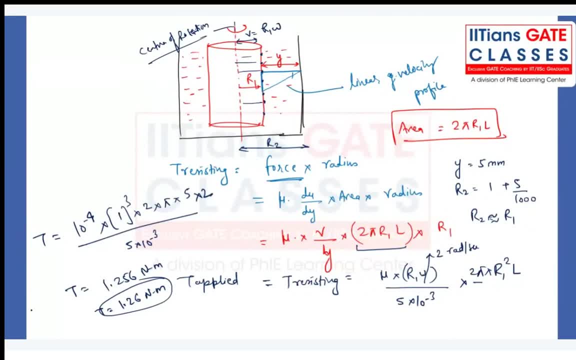 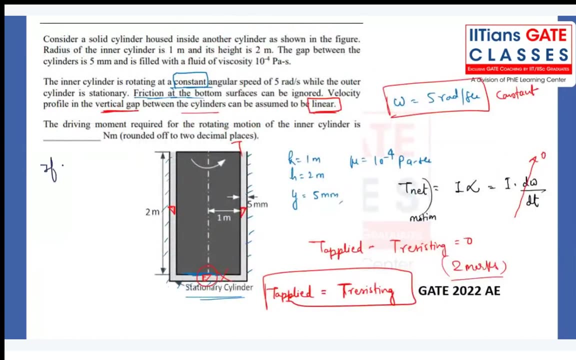 the K-1.. All right, Okay, Thank you. All right, Bye. So when they have not given anything about the velocity profile, remember when the velocity profile they have not given. so if velocity profile is not given, for this case, I am talking. 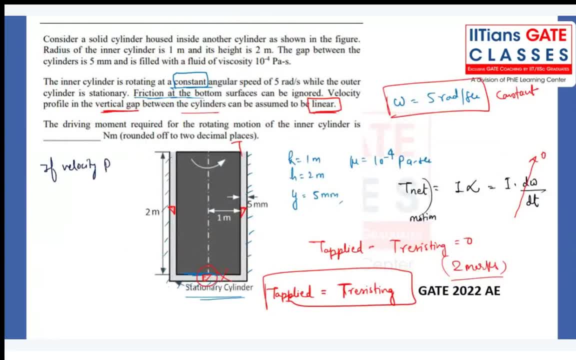 about this case. if velocity profile is not given, then it is a hyperbolic variation. It is a hyperbolic variation. they can ask in MCQ question, right, make a note of it Now. why it is a hyperbolic I will discuss at the end of the class. let me discuss some. 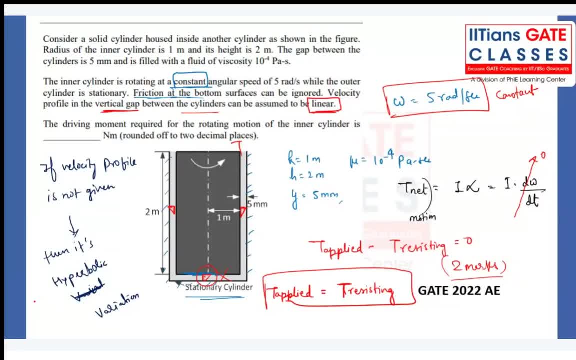 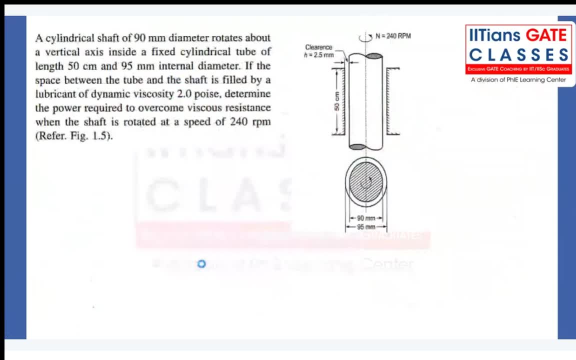 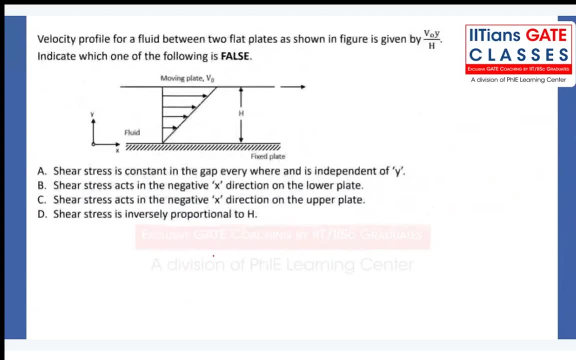 of the few questions. few more questions, then we will see that. now try to solve this particular question. yes, try to solve this question and tell me the answer. Thank you, tell me, guys, the velocity profile for the given cuvette flow, simple cuvette flow. they. 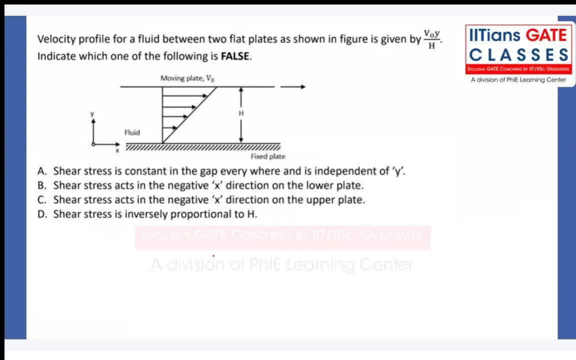 have given and what they are asking. see velocity profile is given as linear velocity profile. right, when you see at any layer what is the velocity value v naught into y by h, that means it's a linear velocity profile. linear velocity profile we i told you right there: stress will be constant. du by dy mu. 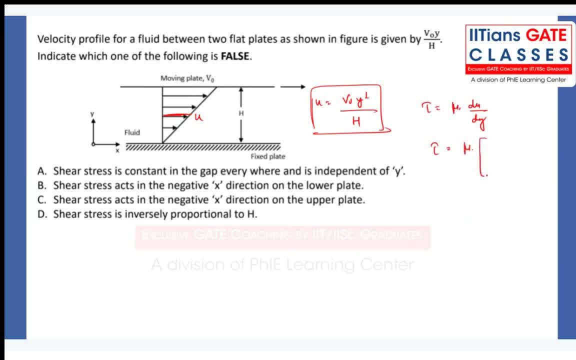 into du by dy. if you just do the differentiation by different, you will be getting what v by h v naught into y by h v naught into y by h v naught is constant. h is constant, mu is constant. this means this will be constant. 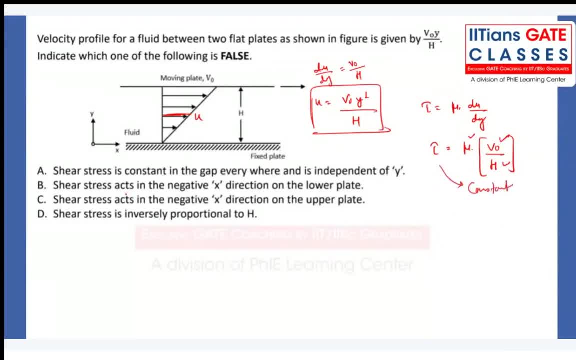 the shear stress will be acting in the negative x direction onto the. what lower plate, correct or incorrect? shear stress is inversely proportional to h. that is correct statement. this is statement. is what correct? the shear stress is constant in the gap everywhere and independent of the y, as you can see from this equation. that is also correct now. when i told you in the last 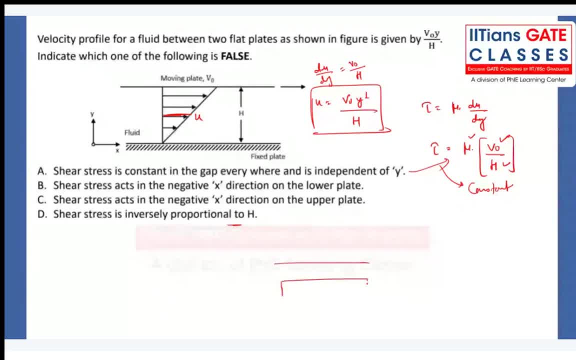 class is false, right. and what about c statement? same thing is applied to third line of the fluid element, right. so we have discussed there, we have discussed very clearly that when it will try to move in the C statement, sales stress acts in the negative X direction, onto the upper plate, That is. 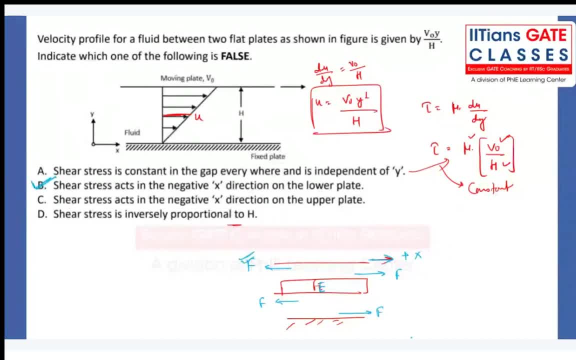 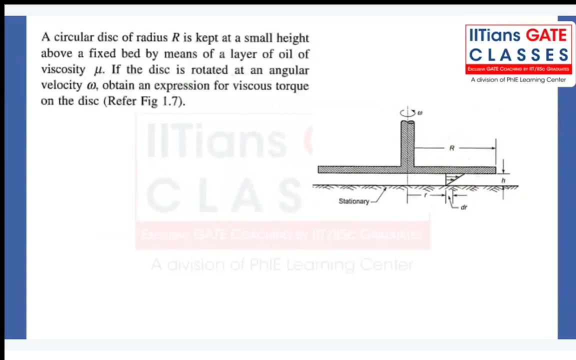 correct, Yes or no, guys? Now can I move to the next one? Now you try to solve this particular question and tell me the answer: A circular disc which is being given in the problem. Now there is a circular disc in which we have the fluid, as you can see. Now we have to rotate it. 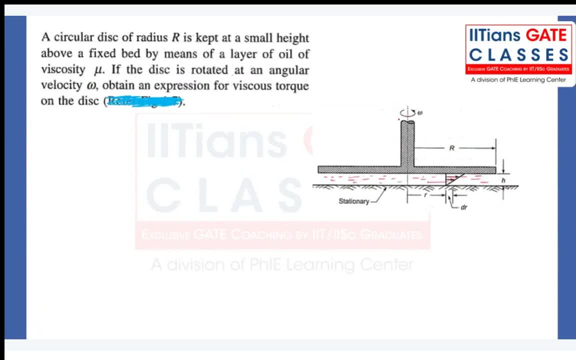 by some constant angular velocity. Definitely we have to apply some kind of torque right to maintain that speed. They are asking: what is that viscous torque onto the disc? They are asking: what is the viscous torque offered by the fluid on the disc? Now you can see that the disc is not moving. So you can see that the disc is not. 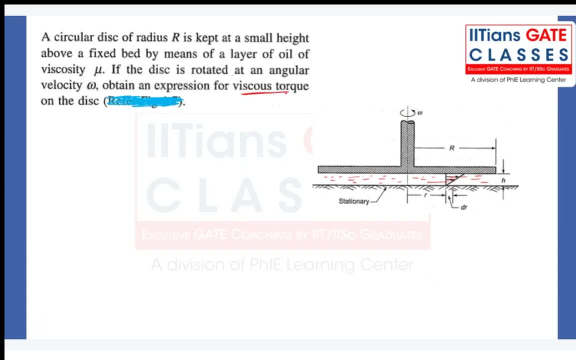 moving. So you can see that the disc is not moving. So you can see that the disc is not moving. Now I will try to solve this and tell me the answer. Okay, let me give you the option, Just wait. 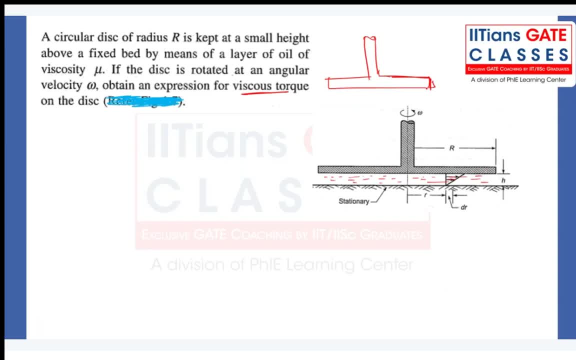 Okay, option number: a new five mu? r to the power four divided by two h. five mu? w r to the power four divided by h. two pi mu w? r to the power four divided by h. the option will be zero, Thank you. So again, very simple question, but little bit of understanding is required. 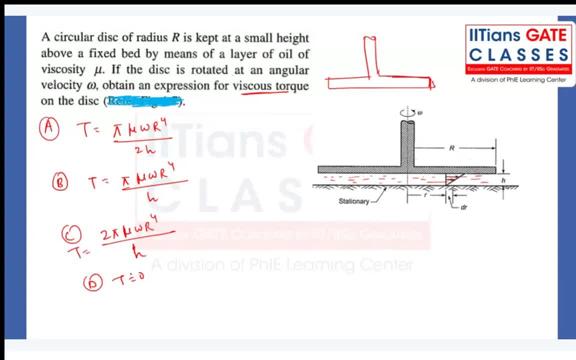 When you understood the concept of what you see In the previous problem, You might have seen the concept right. I told you one word: we don't need to perform any kind of integration. But right now, when you just look it over here, right? 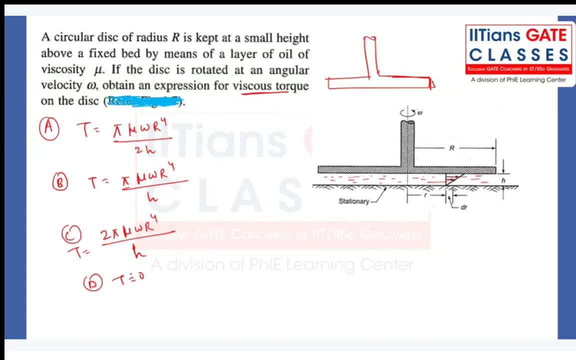 When we just lie right, this resisting torque, The resisting torque might event force into r Right, right. when you observe from the center of rotation- this is my center of rotation, this is my center of rotation- right from the center of rotation, my different, all the fluids. 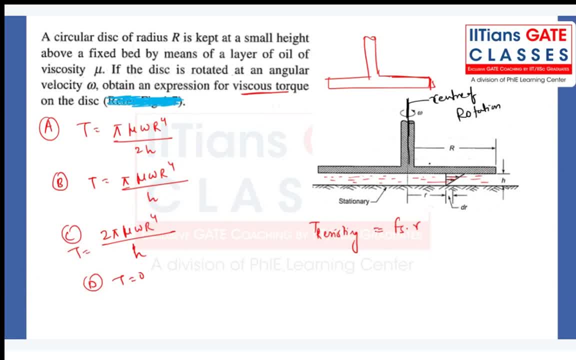 are not at the same distance. see, when you keep on moving, the radial distances keep on changing. definitely we have to perform the integrations, but they have. clearly we have to assume that whatever the small height is there, definitely we have to assume the velocity profile to be linear. 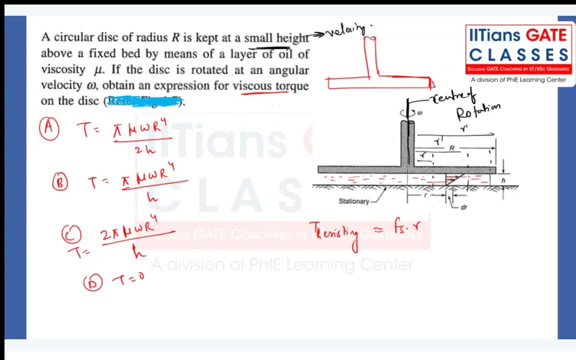 one velocity profile to be linear, one we have to assume here over here definitely they will mention in the problem: velocity profile has to be linear, one mu into v, by h. that is a gap because of the linear velocity profile into radius, right into area. what is the area on which this forces? 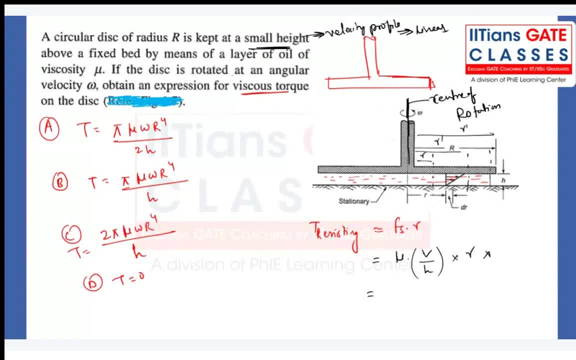 will be acting, my different when you think of the area, when you draw the top view and at any radial location, when you consider the small elemental area, this elemental area- my different- which i have taken at a distance r from the center of rotation, having the thickness dr. so what is the area on which it is acting? 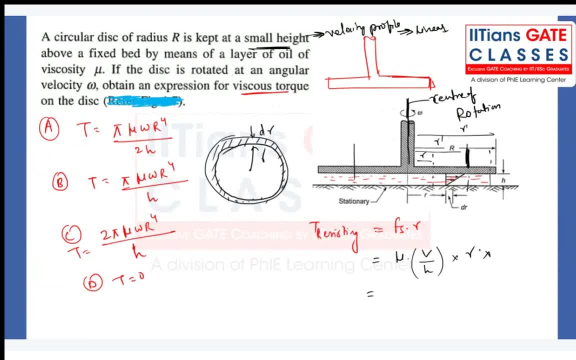 you only try to assume right: 2 pi r into dr. 2 pi r into dr right now. now, once again, yeah, correct, once again you try to assume what is happening over here, what is happening over here. so mu into velocity will be what r into omega. now, we cannot write constant r into omega. 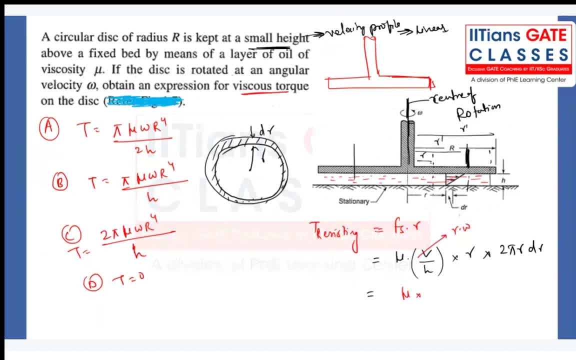 right, as every fluid is having this different, different radius sent from the center of rotations r into omega, into r 2, pi r, dr by h. this will be dt. now i have to do the integration. so definitely, from 0 to r, right from 0 to r, i need to perform the integrations. so what i will be? 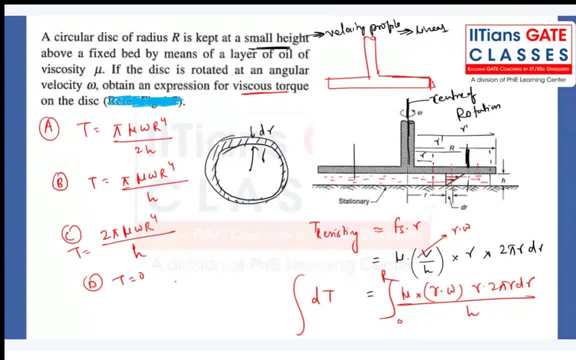 getting my different. if you just do the power integrations you will be getting what pi into mu, into omega, into 2 pi. integration of what r cube into dr by h. so t will be what 2 pi, mu, omega by h, r power 4 by 4. so when you just do that you will be getting the answer as a 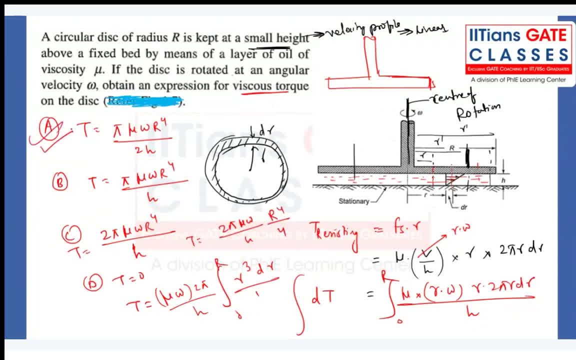 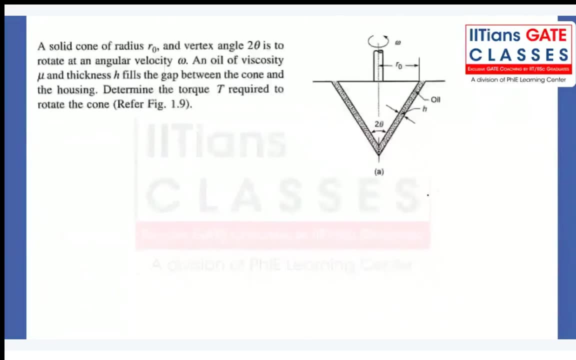 in the earlier case, all the fluid elements are. all the fluid elements are at the constant distance from the radial center of rotations, right? see, in the last problem, i depend you assume that here, whatever the fluid elements are there, they are rotating at the constant distance from the radial center of rotations, right? so what? i will be getting my different. 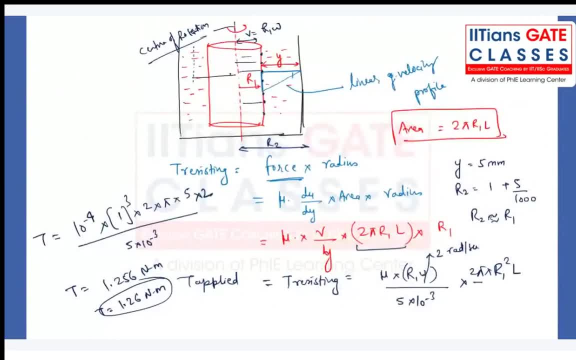 is pi at the fixed radial distance from here to here, that mean radius. we are assuming linear velocity profile. let's suppose, for example, this will be the mean radius. all the fluids are there at the same constant radial location. see from throughout the length, this fluid element, this 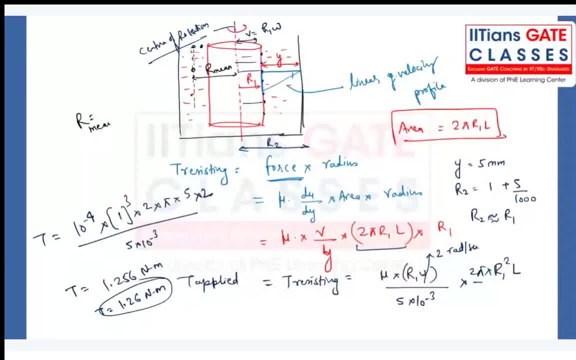 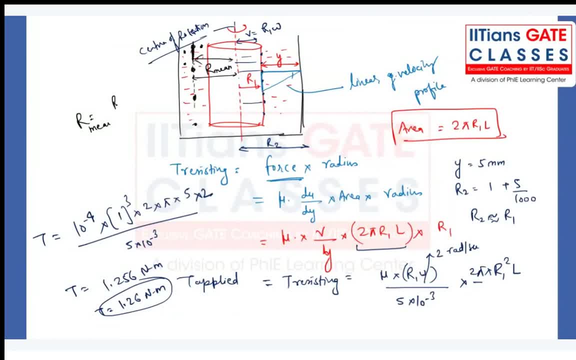 r mean is what r 1 plus r 2? but the gap is very, very small, that r 1 is almost equal to r 2. so you can write r mean that is equal to either r 1 or that is equal to r 2. answer will not change. so 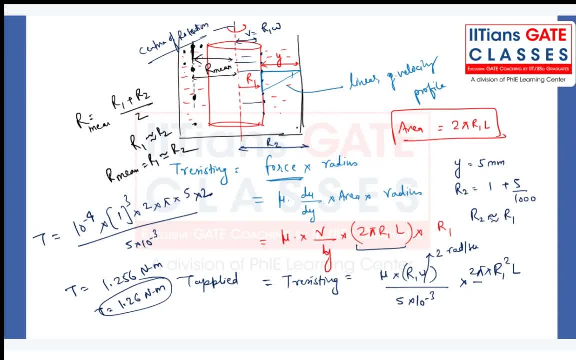 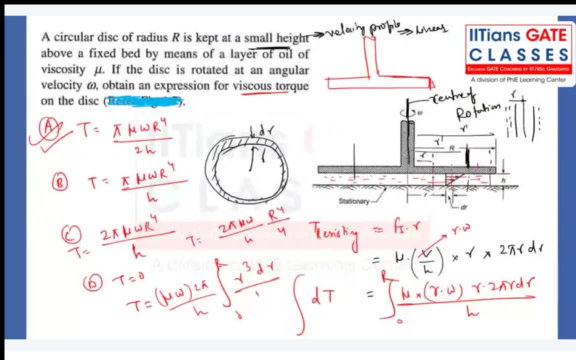 no need to perform any integration over there, but here, when you focus your attention, definitely we have to perform the integrations right. see, at this location, these fluid particles are having what this are. when you just change the distance, what will happen? this is having different radial distance. 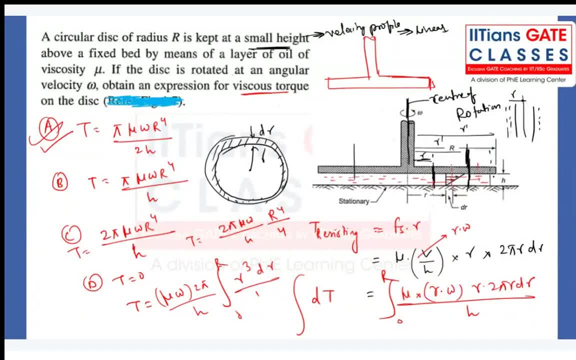 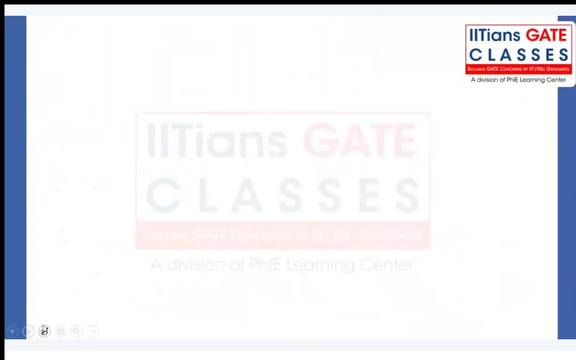 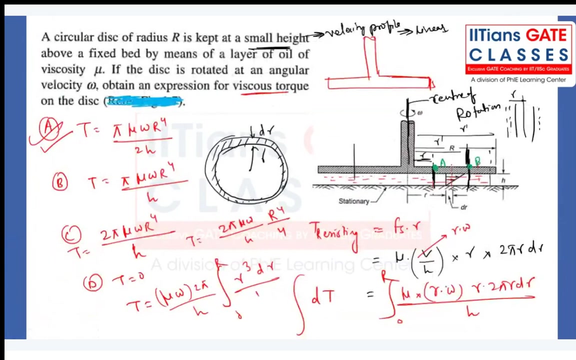 right. so definitely we have to do the integrations, make a note of it. so when you just consider fluid element, for example, if i give the naming, if i give the name, suppose here it is a, here it is b. for both fluid particle a and b the radial distance is different. 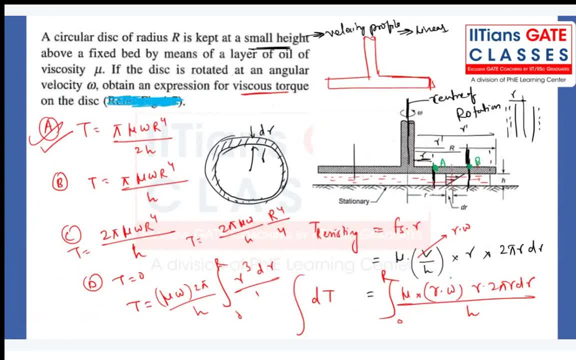 whereas in the earlier case what will happen is that the radial distance will be different. what we have assumed this is a cylinder, now a particle and b particle. they are having the same center of radial distance from the center of rotation, but now it is different. is that clear, all of you? 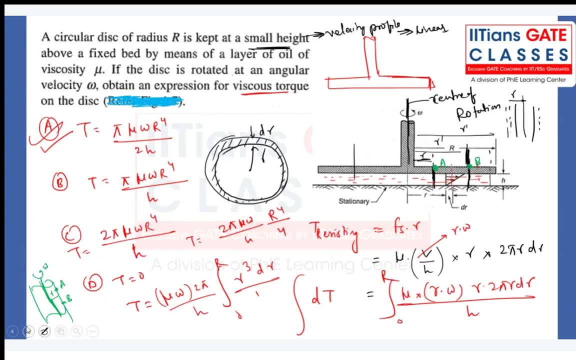 tell me guys, so definitely this question can be asked in further upcoming gate year. is it done? once it is done, let me know we can discuss few more example done so. so try to solve this particular question as a homework. so try to solve this particular question as a homework. 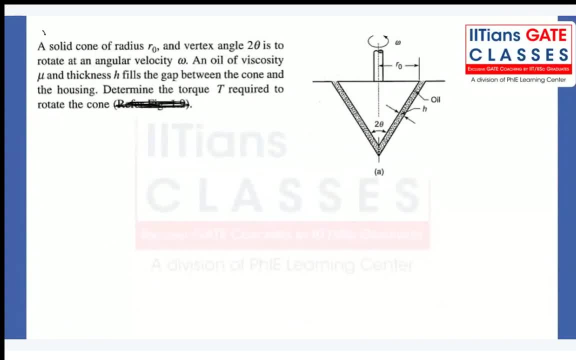 make a note of it or take a photo of this. now there is a conical shape right. slight difference will be there. angle theta will be coming into the picture, but it is in the numerator or denominator, whether it is a sign or cos, that you need to find once again in the gap. you can assume that, whatever the linear 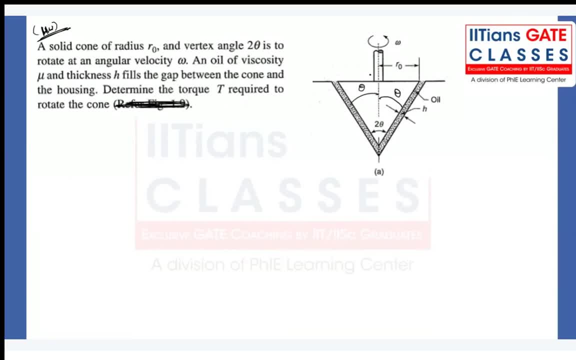 velocity profile is there right, but with the linear velocity profile you are actually going to find that therons Ch, ken. Let's go again to Now. all of you have noted down. can I move to the next one? 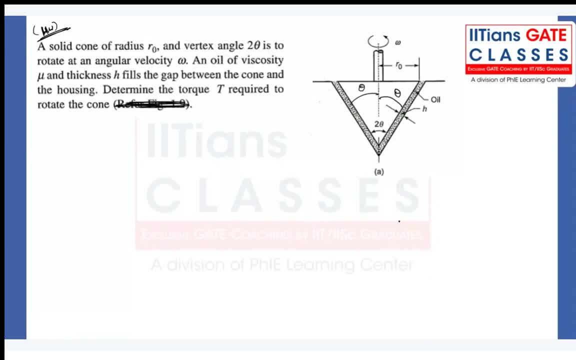 See, in all the questions you might be thinking they are asking torque. What if they will be asking the power torque into omega? so omega one more time it will be coming. remember that That will become omega square right. See this question I have taken from Subramaniam. 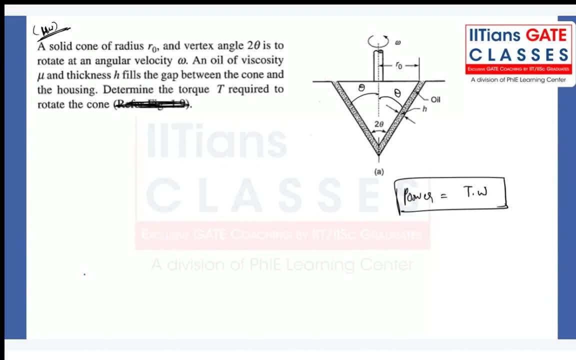 There are more questions are there on this particular topic, but I will be suggesting you to solve from the essential only right, Okay, Okay. So maybe you can follow FM white for solving the numericals. Is it done? Can I move to the next one? 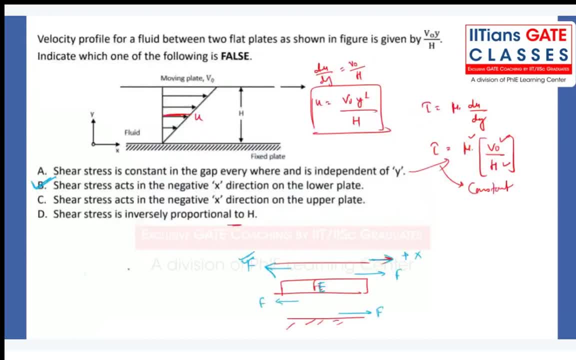 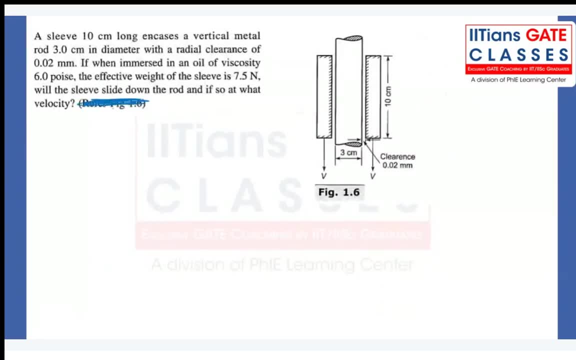 No. So yeah, you can try to solve this question also as a homework and let me know in the next class the answers. Maybe you can note down the answers. I can tell you the answers. 2.66 centimeter per second. 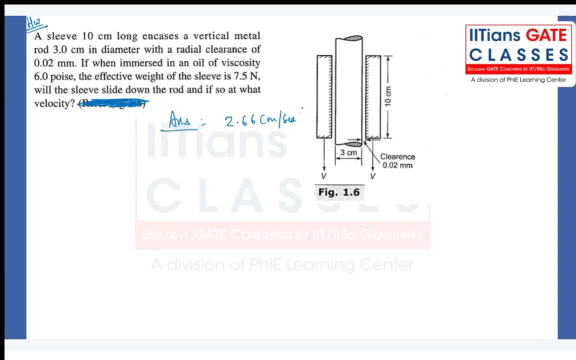 So, yes, you can do that. I will help you solve this question first. Hey guys, What will be happening if I consider, Suppose, if I will be giving you some hints? I will be giving you some hints- hints not for this question, but i'm asking you one question. 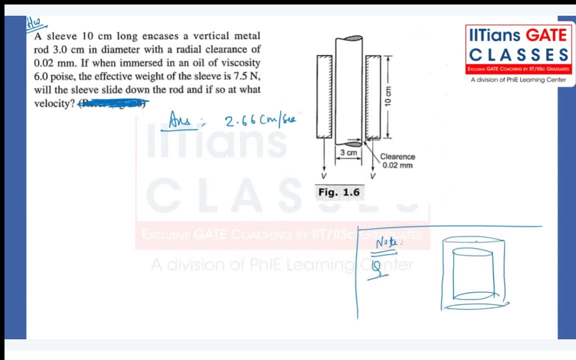 for example, there is a fluid and maybe you can consider: both are there in a container, like this, concentric cylinders, and maybe you can think of: there is a liquid over here, and then this is rotating in one direction and this is rotating in another direction. for example, 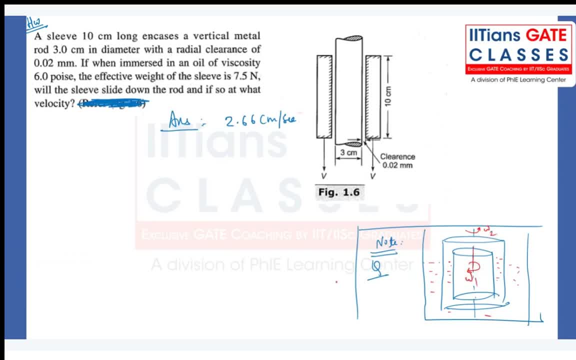 both are rotating in the opposite sense. for example, there is some mechanism or by which both the cylinders are rotating in the opposite directions, assuming the linear velocity profile. what will be my different? uh, what you will like, right in the resistive force. so when you write the resistive force, sales stress, into area in that sales stress you can write: 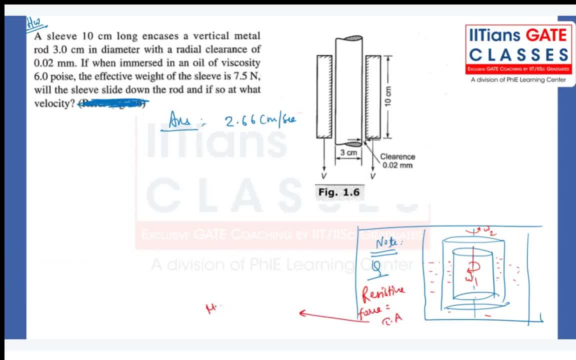 v, mu, into what? whatever the v we are writing, you know actually, two pi, whatever the radius is there, into, well, this is actually the relative speed, relative velocity, but the moment we have seen that outer cylinder is being fixed one, so we are writing only the one v. 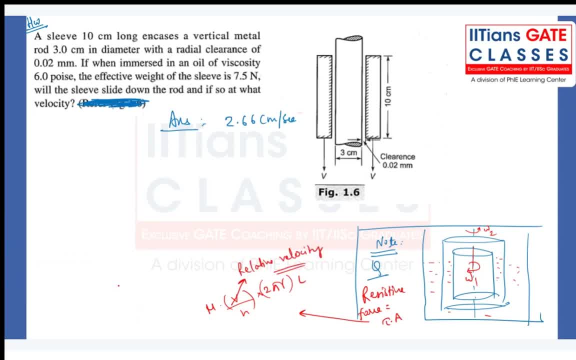 so we are writing only the one v. but when both the cylinders are rotating they will be added. the relative velocity will be added when they will be rotating in the same sense, they will be subtracted right. so this is some of the typical mechanics. one problem for the mechanical right for aerospace, you can. 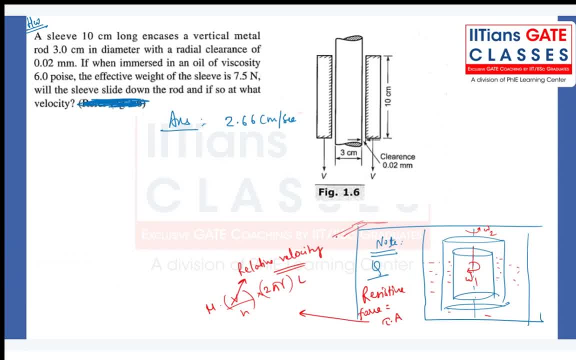 just neglect that as not that important. yes, correct, as you can see, the radius is not creating any trouble for us as r1 and r2 almost a very, you know, very, very similar value. right, as the gap is very, very small and we are assuming linear velocity profile. 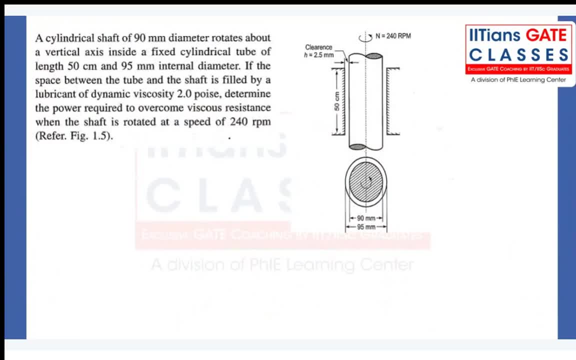 again, same problem you can solve, as we have already discussed in gate 2022. so you can note down the answer for this question. also, what is the power required to overcome the viscous resistance? so note down of 14.5. what take a picture of this directly, don't you know? basically, note: 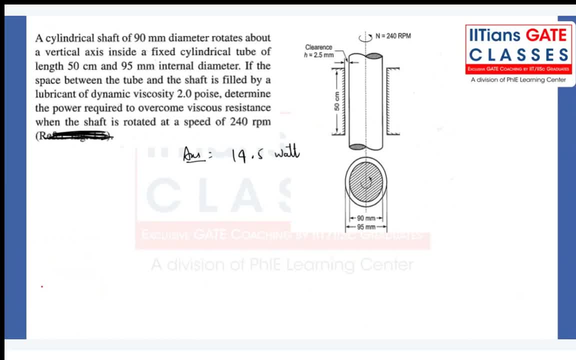 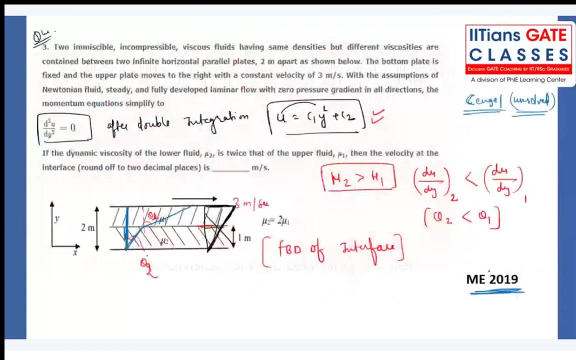 down, don't make a note of it, but you just take the picture of this you done all of you have noted down. can i move to the next one? so now, guys, uh, we have to just think about the rheology. that is a branch of the science. 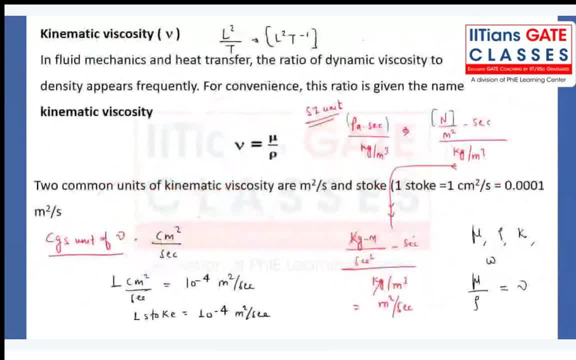 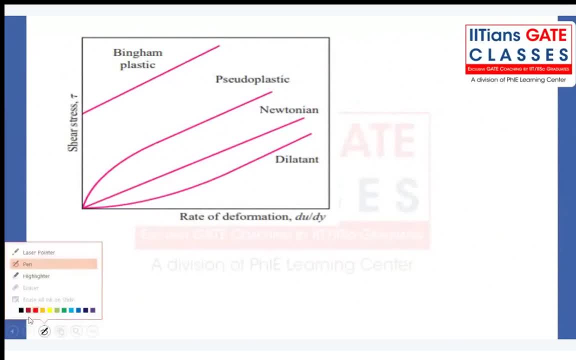 which deals with the different types of fluids. here i'm talking about this one. so No doubt rheology. It is a branch of the science which deals with the study of different types of fluids in a flow. One more definition: non-neutronium fluids. 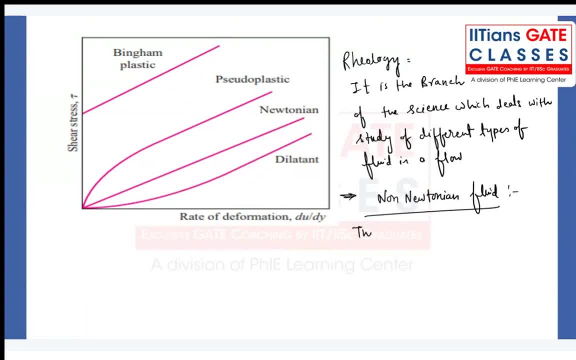 The fluid which does not obey Newton's law of viscosity is called as non-neutronium fluid. Now there are two types of non-neutronium fluids. One will be time independent fluids- Time independent non-neutronium fluids. Other will be time dependent non-neutronium fluids. 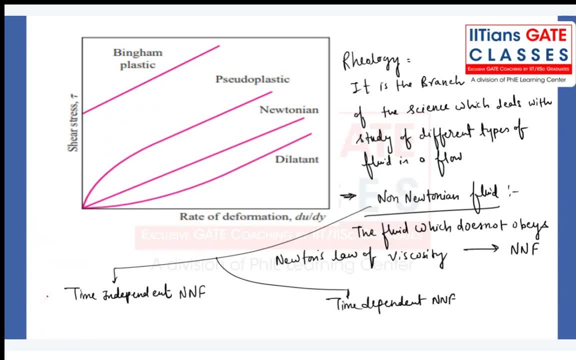 But the big concern over here is that: what is the relationship? So that is going to be? tau is equal to A du by dy to the power n. Now, what is the meaning of A And time? independent fluids will be: note down: B plus A du by dy to the power n. 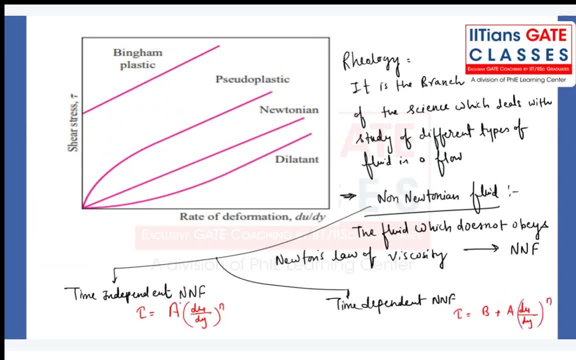 Where A is nothing but consistency index. And what is the meaning of B? B, we can note down flow behavior index. And what about n? That is the exponent Right. That is the exponent That depends on the types of fluid. 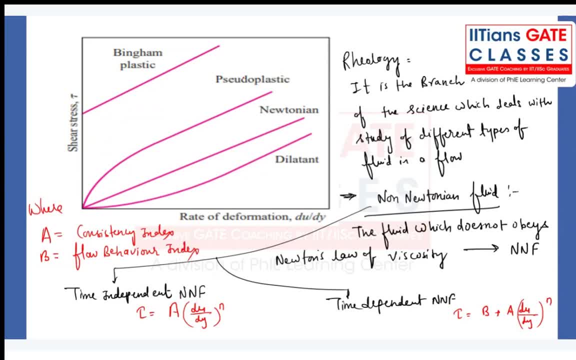 Right When I talk about the pseudo-plastic fluid. for the pseudo-plastic fluid, n will be less than 1.. B will be 0.. And by looking the nature of, say, the stress and rate of deformation, now tell me the. 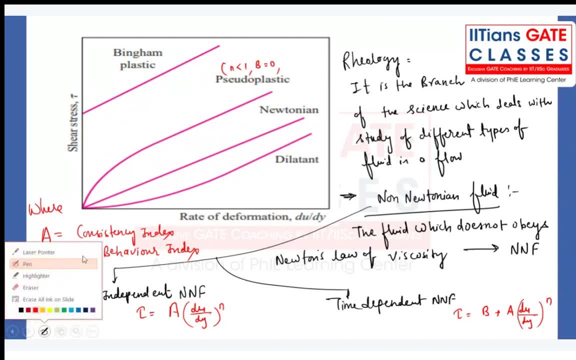 slope is increasing or decreasing For pseudo-plastic fluid. Yes, For pseudo-plastic fluid, the slope is increasing or decreasing. Slope is increasing or decreasing. Tell me guys. Very high slope, Very, very low slope. Slope is decreasing. 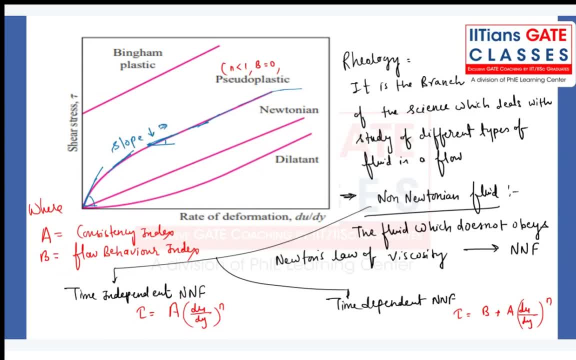 This causality will decrease. That is why pseudo-plastic fluid is also called as shear-thinning fluid, what we call shear thinning fluids. Make a note of it. We also call this fluid to be shear thinning fluids. What is the example? No, no, no, It is the graph, something like: 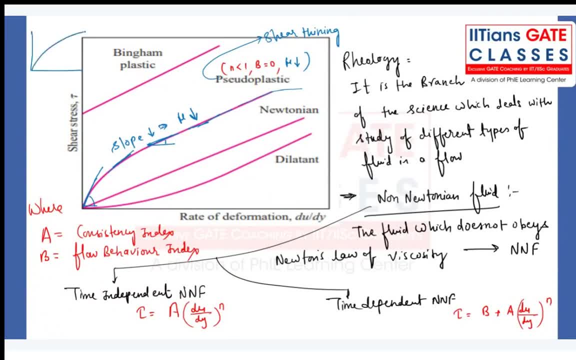 this, Remember. it is like this Slope is always decreasing, right. So shear thinning fluid. what is the example of pseudoplastic? Tell me guys, Anyone know that example for pseudoplastic fluid? Tell me guys, Milk Blood. 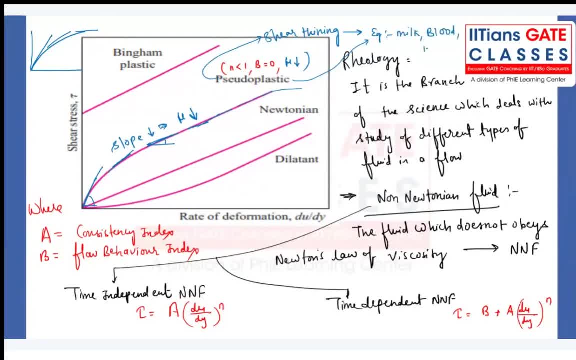 Ink, ETC, Or maybe ketchup. also, you can think of. What about dilatant fluid? Dilatant fluids: n will be greater than 1, b will be 0, mu will be increasing. See slope is what Continuously. 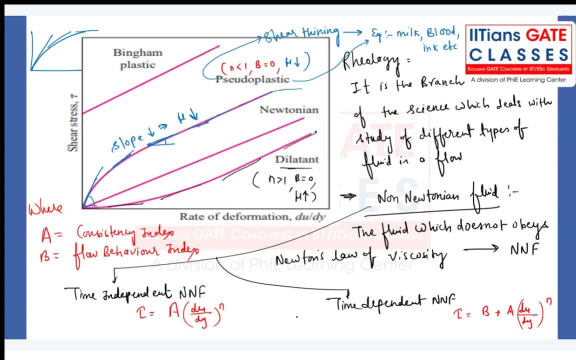 increasing. you know The slope is continuously increasing. That is why we also call that to be shear thinning fluid. What are all the examples of that? What are all the examples of shear thinning fluids? Sugar solution, right Sugar solution, Sugar in water, solutions That you can think of? 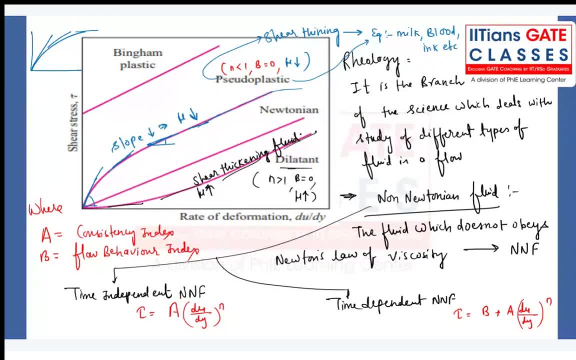 dilatant fluids. No pence will be considered. Whatever you are telling about the pence, that will be time dependent fluids. Some pence we are considering in the thixotropic fluids, What we say gypsum, whatever the gypsum paste is there and all that is the time dependent fluid. So you 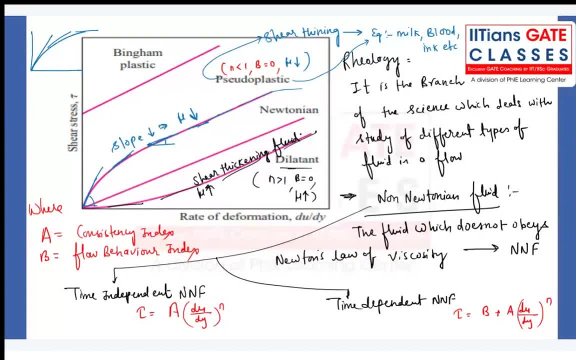 can say gypsum paste. Whatever the pence are there, that is nothing but thixotropic. What about bingham plastic Now? bingham plastic is basically certain fluid which telling me that at initial, for the some amount of duration, we have to apply shear stress, Why we have. 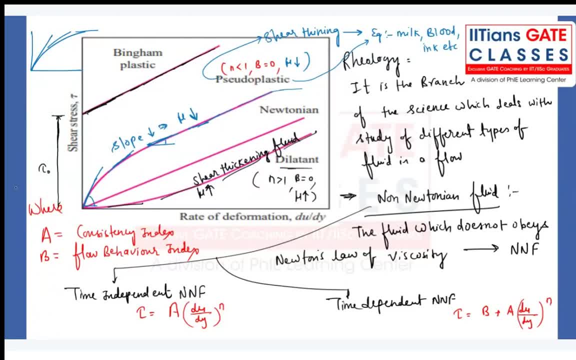 to apply the shear stress Now in the bingham plastic fluid. if I tell you the example, that is the toothpaste. Now toothpaste is not behaving like a water. in which tube is there Directly? when you open the, whatever the cap of the tube, directly, liquid will come out. No, paste will not come. 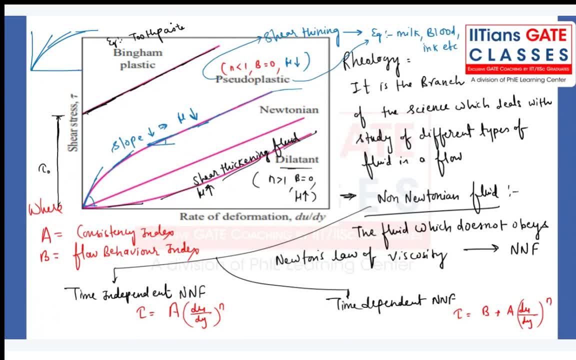 out. We have to press it, That pressing part. we say that turn off. That is the example of the bingham plastic fluid. Can you tell me some other example of bingham plastic fluid, Drilling mud? Again, you can think drilling mud as the example of bingham plastic fluid. Make a note of it. 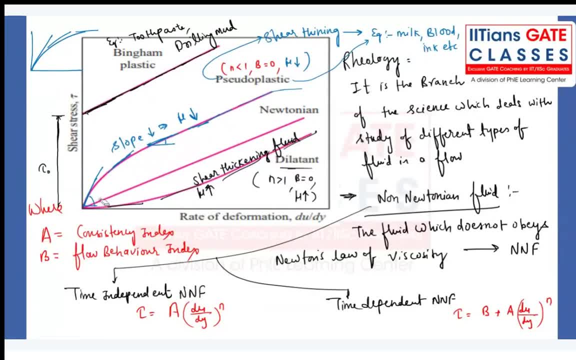 Let me just clear this part. Once it is done, let me know These are the fluids till now. we have discussed- that is the time- independent non-Newtonian fluids In our whole fluid mechanics or maybe in aerodynamics. you may not be bothering about those things. 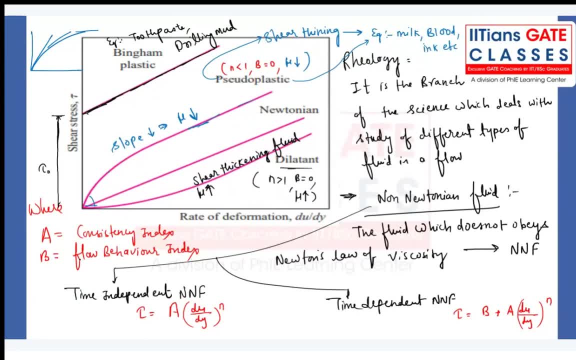 you know, non-Newtonian, Even in the Navier-Stokes also, we are directly putting the value of final formula, whatever the equation we have. that is for the Newtonian fluids. We don't discuss anything about the non-Newtonian fluids. We don't discuss anything about the Newtonian. 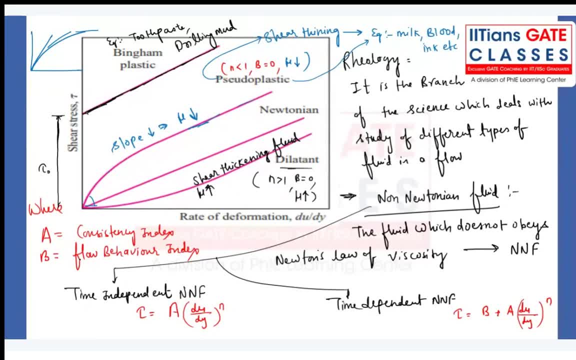 fluids. We don't discuss anything about the Newtonian fluids. We don't discuss anything about the Newtonian fluids Because, when you take the example of the aircraft air, that is the ideal gas we are treating like an ideal gas again. that is, once again, the Newtonian fluids, Yes or no, guys? The 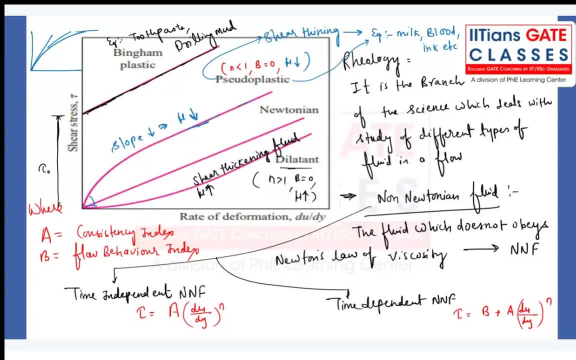 air which is flowing on the aircraft. what is that? Newtonian fluids, right. So there is no meaning of studying the rheology. being aerospace engineer Of course we should, knowing this thing, but again, not required for the gate examinations. 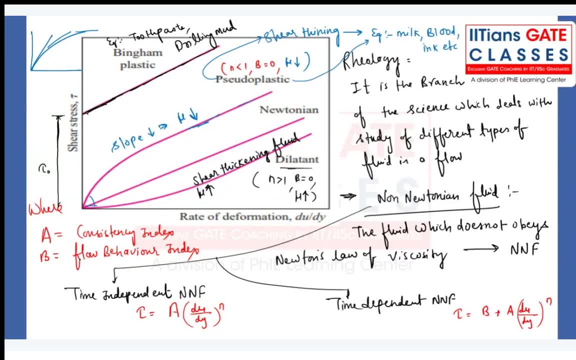 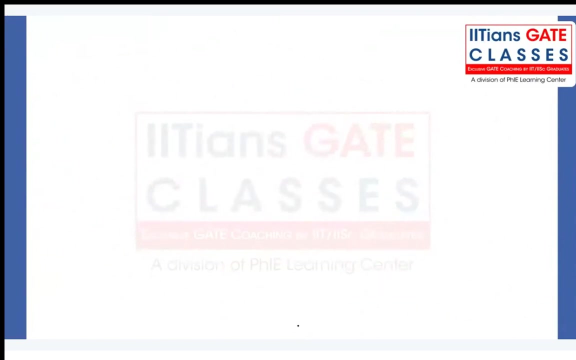 can i move to the next, uh, next, particular page? is it done for all? is it done now? you try to make a note of this. so i'm talking about this time dependent non-newtonian fluids, tau versus du by dy. so what you will observe, you will observe that 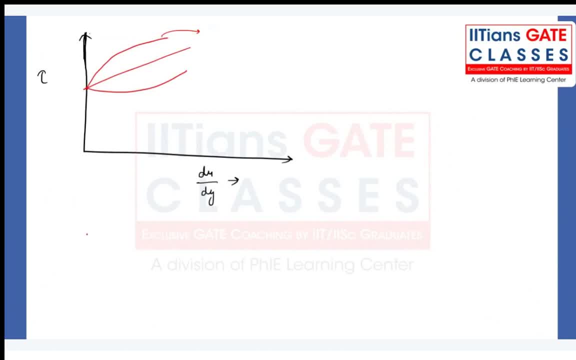 this is nothing but thixotropic fluid, what we are calling thixotropic fluid. that means here. thixotropic fluid means: what is the advantage over here? n will be less than one, b will not be equal to zero, and once again you see the slope of that slope. 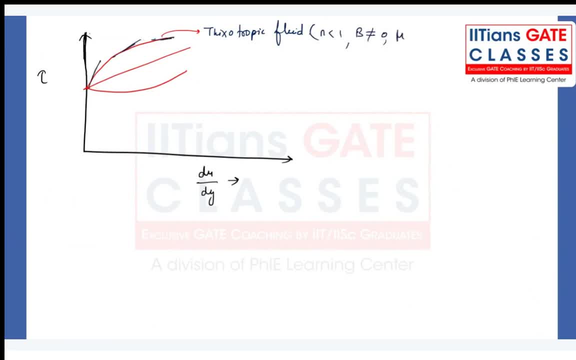 is higher, slope is what decreasing, and slope is what this cause of viscosity, whereas in the newtonian fluids you observe that the newtonian fluid viscosity is not changing with respect to rate of deformations. this is called as rheoplastic, a hebour pacted fluid where n is greater than 1, not equal to 0. this is something like this: 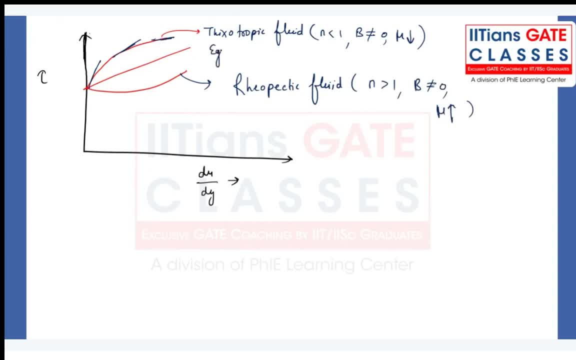 what are all the examples of thixotropic fluid? what are all the examples of thixotropic fluid, of thixotropic fluid that represents the soil? uh, buckingقةUC-RH, please, 말베 и 베�Ter. the examples of thixotropic fluid, my different. whatever the paints are there, right, but some. 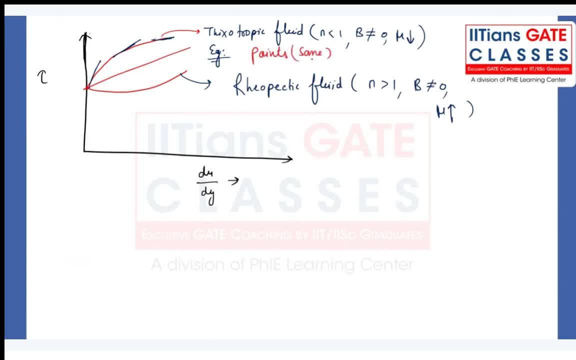 paints, not all right. and what are all the examples of rheopactic fluids? gypsum paste. that means when you try to see, when you, when you observe the video- youtube videos- of gypsum paste, when you search it, when you keep on applying the rotating shear stresses, when you just keep on applying these shear stresses, what you will observe? that it is become thicker. 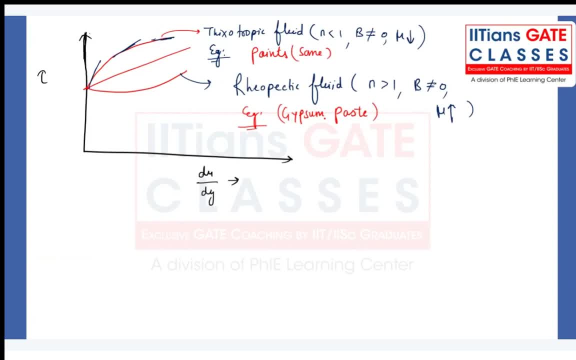 and thicker. with respect to time it will become thicker and thicker. you try to observe the experiment right. and we know that gypsum paste. we use it for basically what: plaster surgeries and all you know- basically to any parts of the body in which we have to do the plastering. 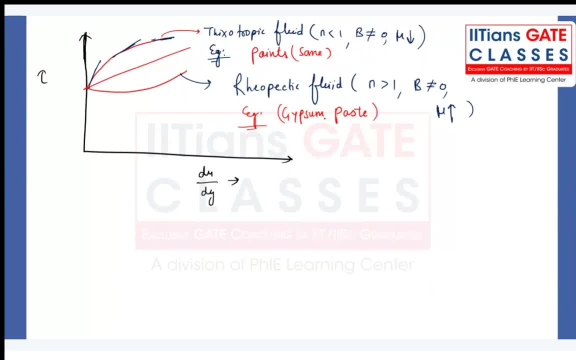 there we use this gypsum paste, right. so again, in the biomedical field, non-newtonium, or branch of the rheology, is a very much significant. you know that plays a very crucial role there, right. but for aerospace or being mechanical, we mostly talk about the newtonian fluids. 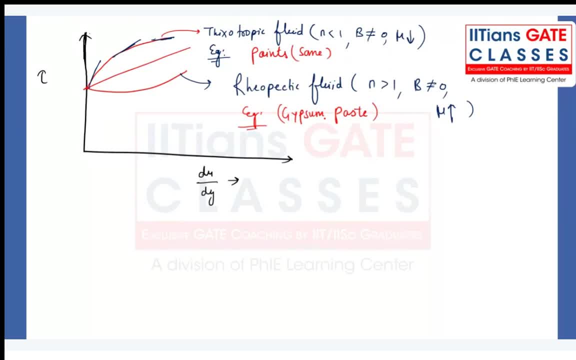 right, and so we are just going to be talking about the newtonian fluids here, and we are just going to be talking about the newtonian fluids that are present in these gases, and then we are going to be talking about the x-ray, and then we are going to talk about 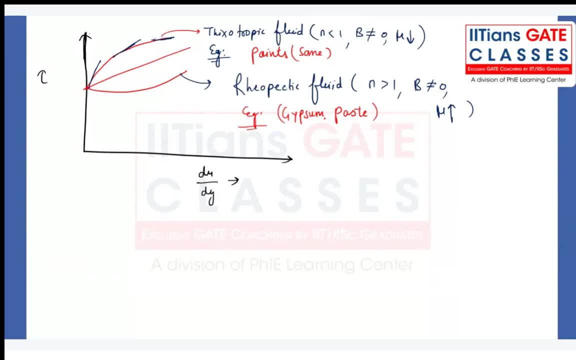 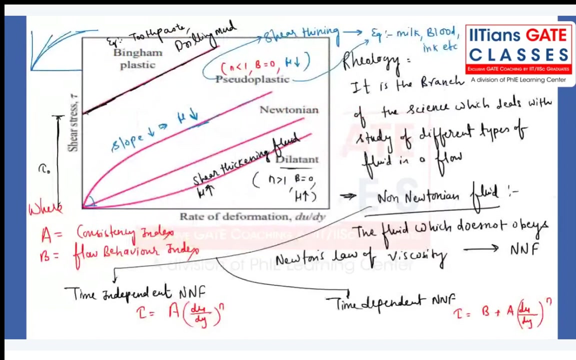 the gypsum paste. right, and that's it for today. anyone else who wants to speak about gypsum paste, please feel free to do so. let's move on. Thank you, See, guys. so, yeah, What are all the examples of dilatant fluid I have not discussed. 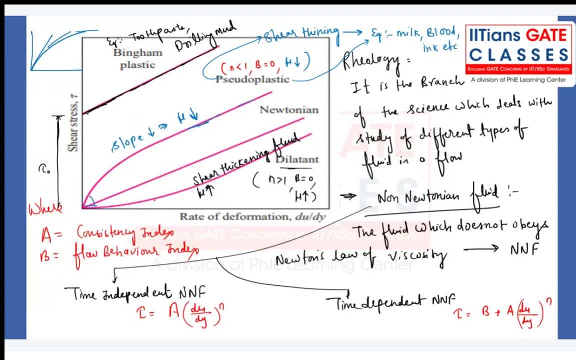 What is that? Sugar in water solution, right Where you can write. You can write over here: Sugar in water solution, Sugar in water solution, Or you can also have sand solution. Once it is done, let me know Now. 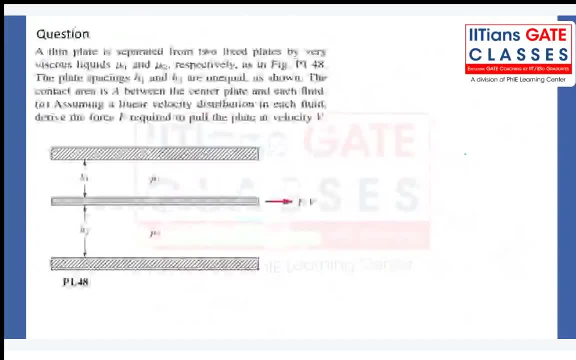 See, try to solve this question. Sorry See, it is a very simple one right Here. that is a fixed one. Bottom is fixed. So what will be the velocity profile? The velocity profile will look something like this: 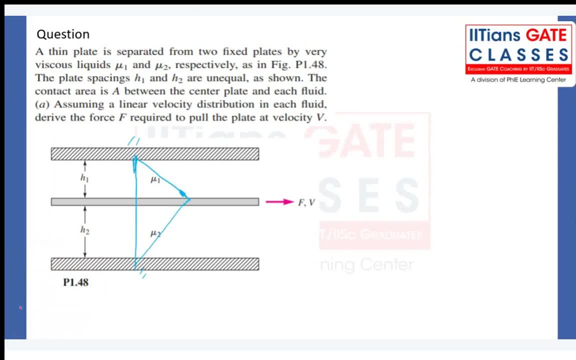 Here what we have done, Here what we have done. A thin plate is separated from the two plates- This is fix plate- by the various viscous liquids mu1 and mu2, respectively. as shown in the figure, The plate spacing h1 and h2 are unequal. 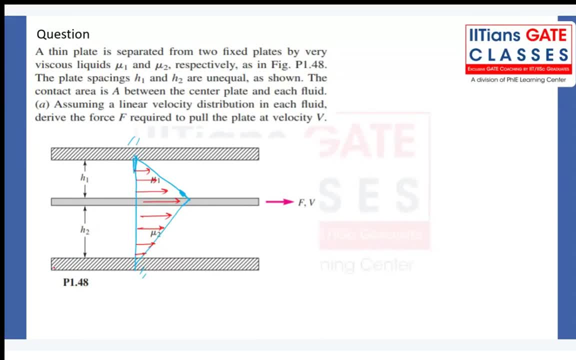 The contact area a between the central plate and each fluid they have shown in the figure. Assuming the linear velocity profile or linear distribution in each fluid, the driving force f that is going to be required That pull the plate at a velocity v. 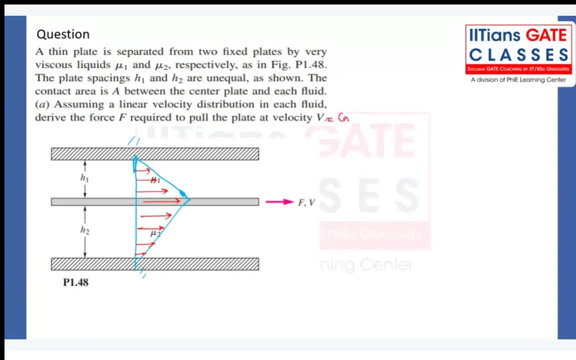 That is a constant velocity. So net force in the direction of motion will be mass into acceleration. So acceleration will be zero because a is equal to what dv by dt, being known that v is constant. So when you do the differentiation that will be zero. when you draw the free body, 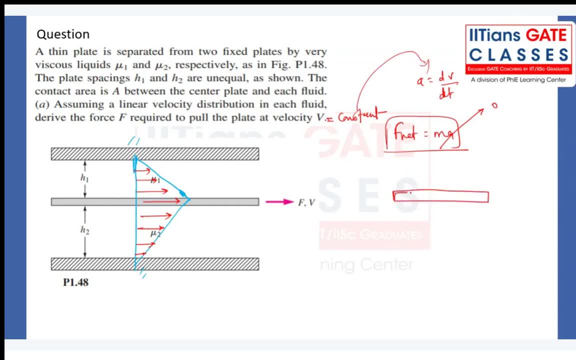 diagram of the middle plate right. What will be the free body diagram? What will be the free body diagram, My dear friend? it is a very simple. when this plate is moving in the forward x direction, this plate will offer some kind of resistive force in this direction. in the negative x. 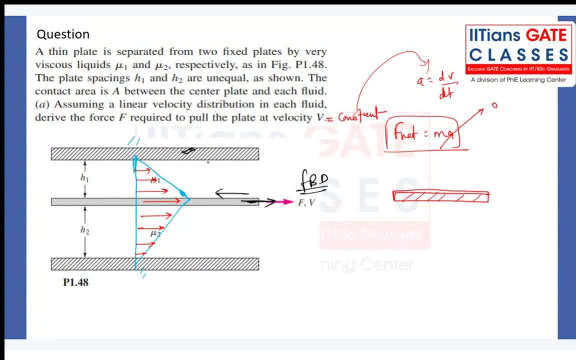 directions and it will offer like this: right, Let us suppose this is F1,, let us suppose we call this to be F1. Bottom plate will offer some kind of force in this direction. that is F2,, F2, right. So the net force will be what? 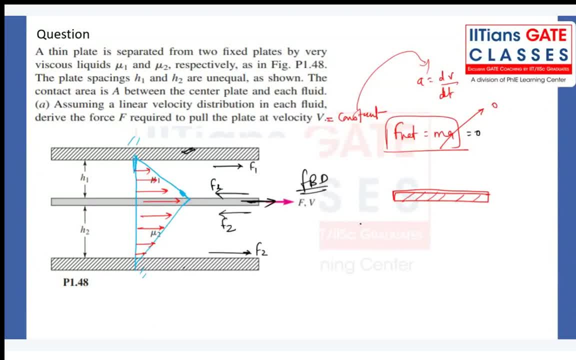 That is equal to zero. So net force in the direction of motion will be what That is. equal to say this one F will be what F1 plus F2,, F will be what F1 plus F2.. Now, what is the F1 value? 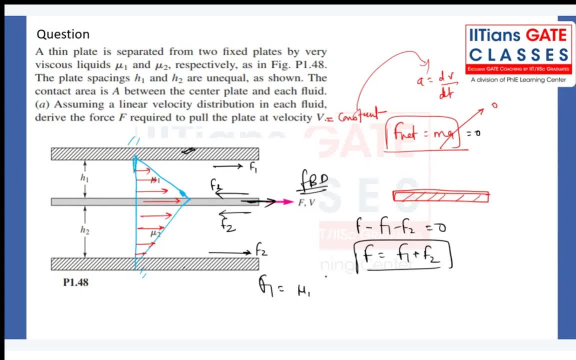 That is a very simple mu1 into. this is what mu1,, this is what mu2, mu1 into v, that is the plate velocity, v by h1, right, And what about F2?? mu2 into v divided by what? 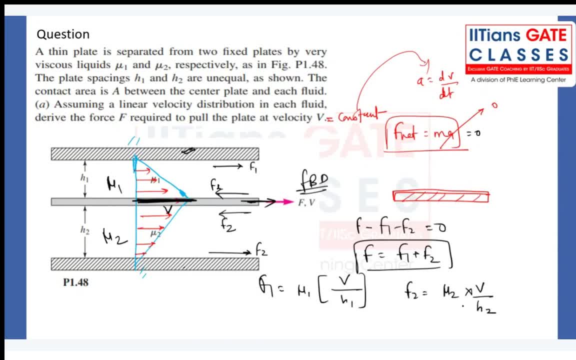 h2.. So that we have to add, we have to find the values of F, that is, mu1, or maybe v by v, by into what, mu by h1, mu2 by h2.. Make a note of it. 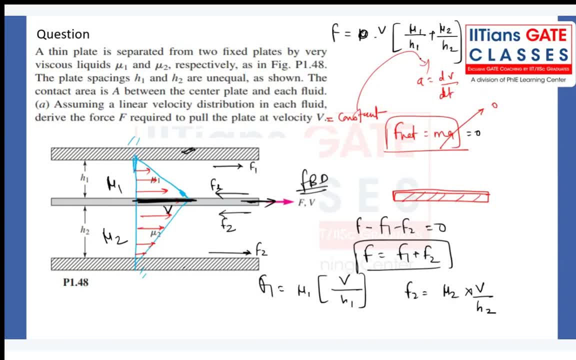 And again, we have to write the area also right Into area, into area, into area where area can be written, as, whatever the length of the plate, into what Width? No Length, into width. That will be the area on which say, the stress will be acting. 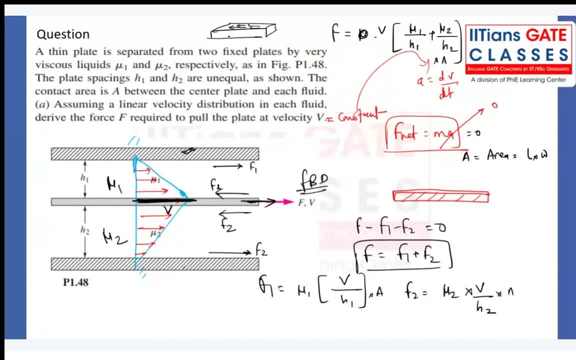 What we have not understood: Whether this particular force is clear. No, The force offered by the plate onto the plate in the negative x direction, that is F1.. When the plate is moving like this, what the this particular plate will say? 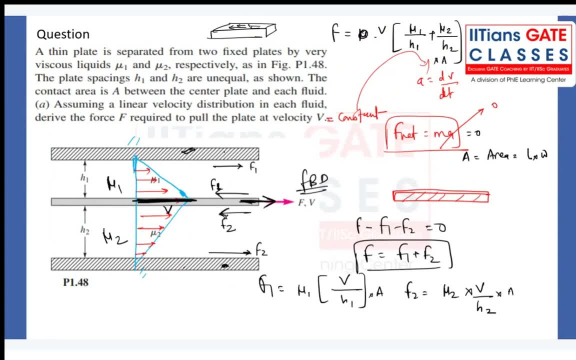 You come back once again. Getting my point. In all the previous examples we have provided the velocity and force to the top plate fluid element and the bottom plate. This is separately. we are discussing some different cases. Getting my point? 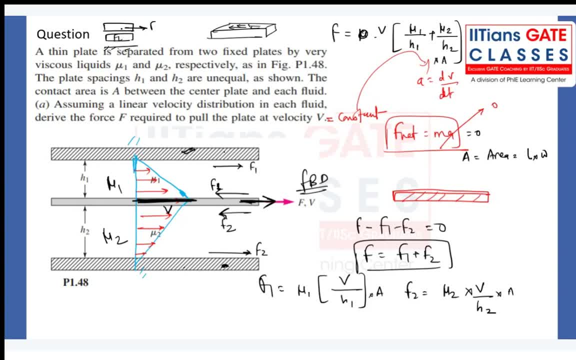 The net force in the direction of motion. Yes, The net force in the direction of motion. In the engineering mechanics. what you have done, that In the direction of motion, what is the force? F, F1 is what Opposite to the direction of motion. that is why negative. 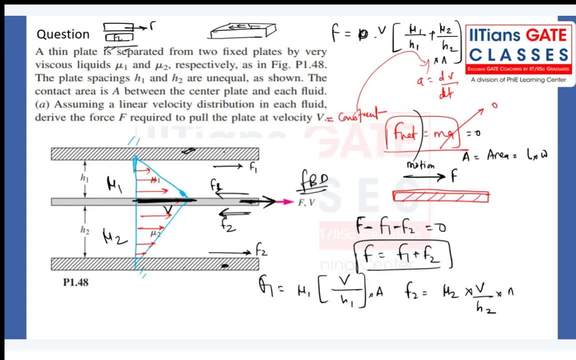 F2, that is also negative. Getting my point: Yes or no, F, F1, F2.. Remember, fluid is not doing anything. F1, F2, F3,, F4, F5, F6, F7, F8, F9, F10, F11,, F12,, F12, F13,, F14,, F14,, F15,, F15,, F16,, F16,, F17,, F17,. 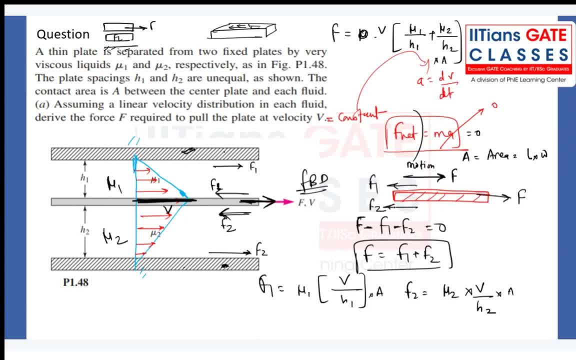 F18, F19,, F20,, F21, F22, F23,, F24,, F25,, F26,, F27, F28,, F29,, F30,, F31, F32,, F33,, F34, F35, F36,. 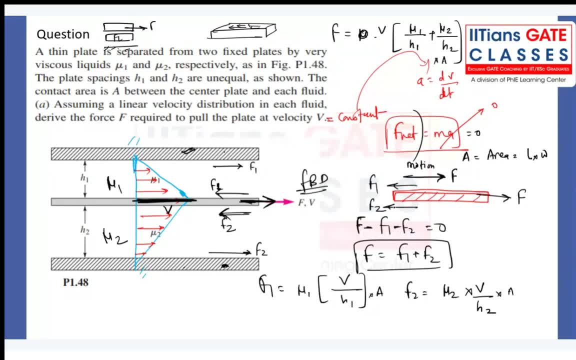 F37,, F38,, F39, F40.. Remember, fluid is not doing any kind of acceleration. Even whatever the discussion happening, suppose, at this location, even though you might be discussing drawing the velocity profile, we are going to have the same value, same 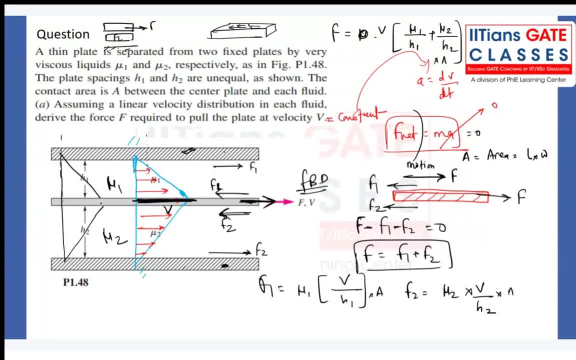 velocity profile that we say fully developed flow. We will discuss what is the meaning of fully developed flow and all. So, whether you place the origin here or here, it does not matter, Yes or no, It does not matter Because it is not having any kind of acceleration. 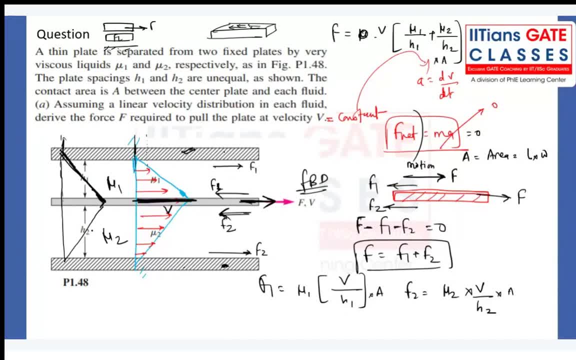 Just like your bike. you know you are moving at some speed, but at a certain point of time you will increase your speed. You know, by lowering the gear. then what will happen? You will be having some acceleration Further. you try to change the acceleration also you will be having a jerk. 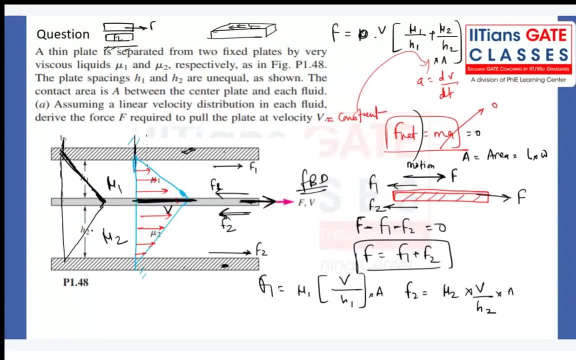 But here those things are not happening. in the case of fluid element, For a simplicity analysis purpose we are taking pulling the velocity, pulling the plate at a constant velocity. Remember that If not, then definitely they have to give some time, and all in the problem itself if 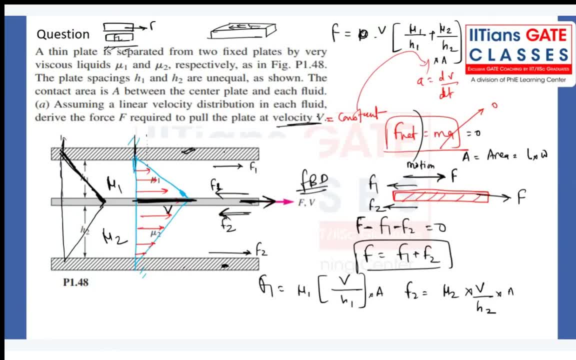 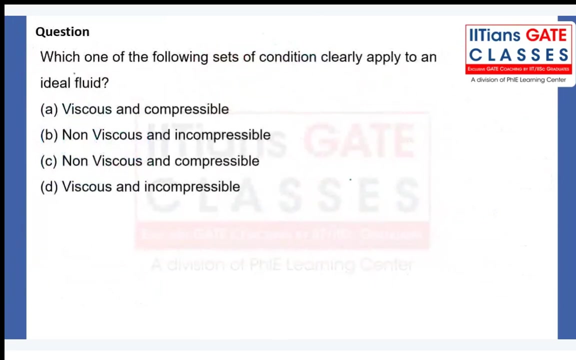 the fluid element is having some kind of acceleration. Also done. all of you, can I move to the next one? All of you, All of you Done. So we have discussed something about this. I will discuss about the ideal fluid separately. 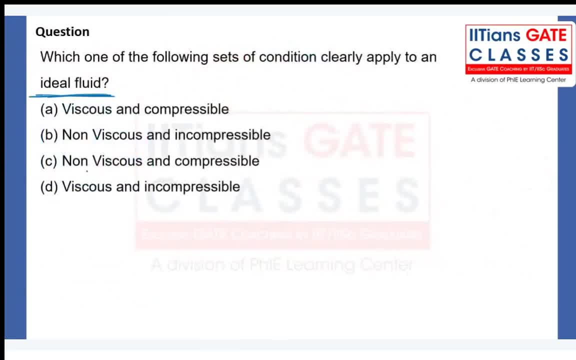 As of now, you just make an answer for this Non-viscous and incompressible Ideal fluid means which is not having any viscosity. No viscosity, no surface tension. Density will also be fixed constant. Make a note of it, Very important. 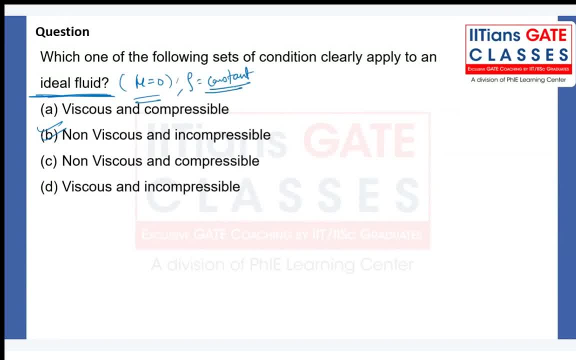 So I have given some homework problem We tried to solve. Put some effort. Tomorrow we have class in the morning, Before that. today night you have another class after this. So in the morning you wake up, you know, and you try to solve those homework problem Maybe. 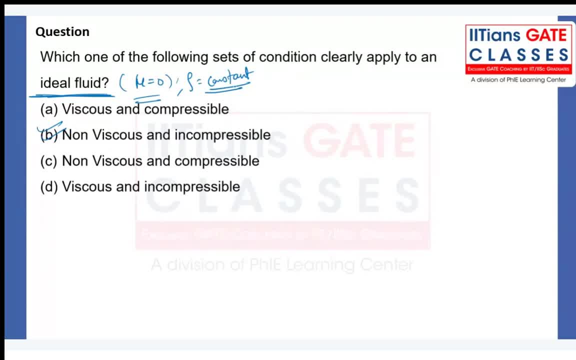 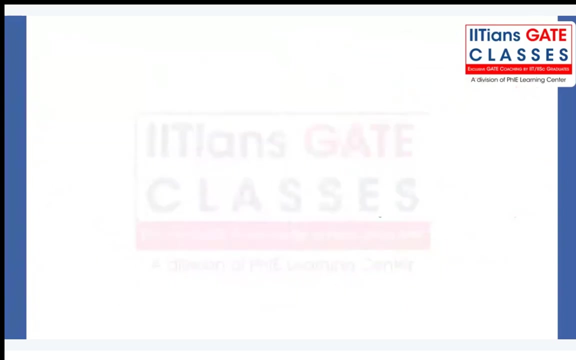 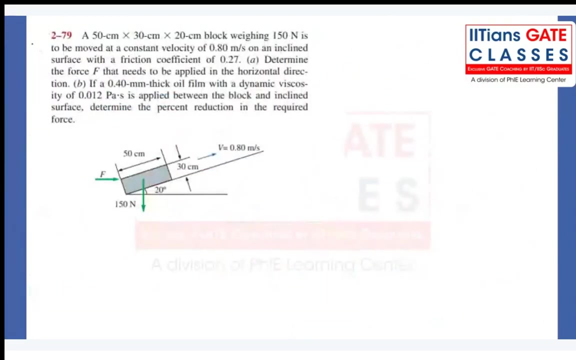 after the class. definitely you will be relaxing. Then, after you know, tomorrow morning you can just wake up early and you try to solve it. Put some effort, you know, Okay, So make a last one That's a homework one. This is again very important question. 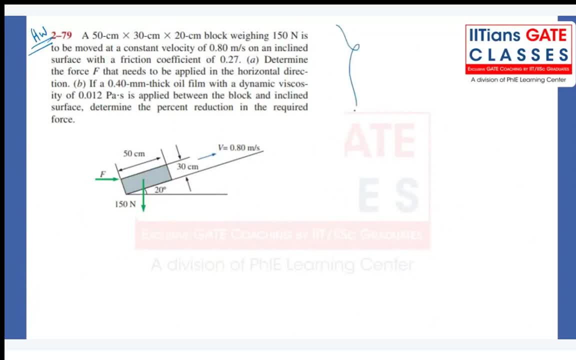 I will discuss this question also tomorrow, But you tried it. At least you tried, And if you need the answer, I will give the answer. also, What is the force? what they are asking? The percentage reduction, or maybe I am giving you the answer for a part. that is a force: 57.15 Newton. 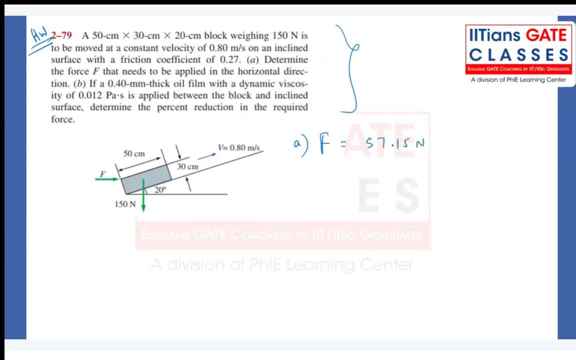 At least you try a part, Not now. So engineering mechanics you can make use of some. you know application of engineering mechanics that you have covered already. So try to cover variety of problem, each and every problem, In fact, I cannot discuss. 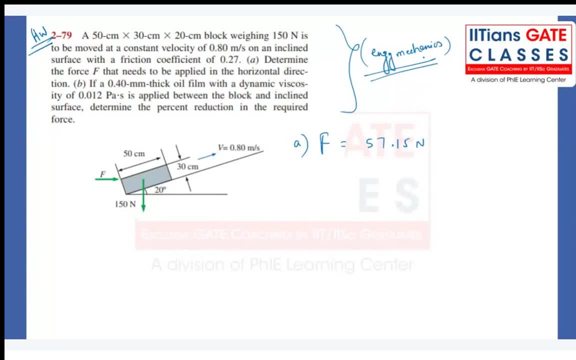 in the class also. So you have to be depending on what, depending on yourself, to you know, have the clarity, Make a one note notebook. you know, suppose fluid mechanics You start solving from the chapter Number one, Number two, Number three, Number four, Number five. 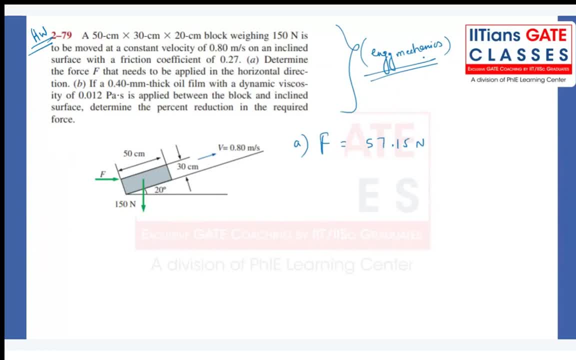 Number sixril. Chapter number one. Chapter number two. chapter number three: objetivo splendor. number ten: All the problem- Don't think like a rough book- That particular book for the first time whenever you're solving, and all the concept regarding every question you'll try to note. 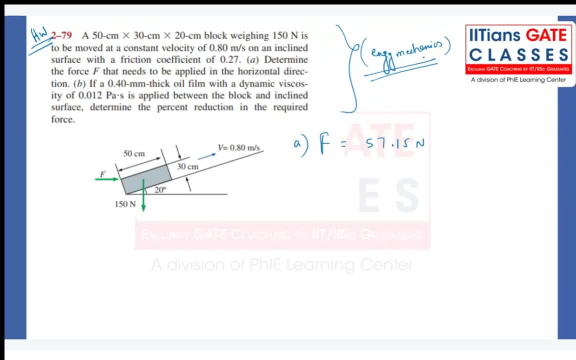 down there itself Along with the solution. Whatever you are feeling about that topic, you make a note of it And after that, second time, when you do the review journey And when you solve- uh, you tried to increase your the speed for time. what did you try? 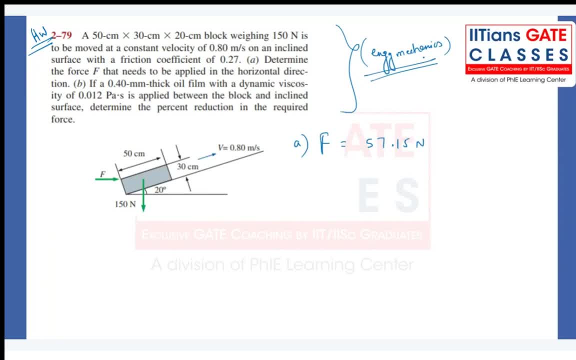 to improve your speed. Yeah, the revision time. you will feel that, okay, this notes. what if you are stucking in between? again, you need not to go back to the lecture and see. you will only have to see what you have written in the notebook, right? okay, this is the mistake i'm doing. actually, i have written the concept there. 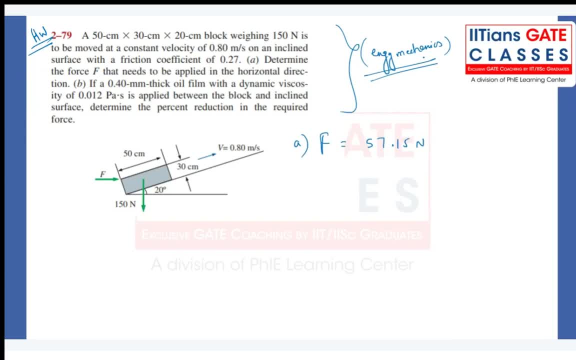 but now i have to revise that concept. okay, this is actually the point i'm missing. now i need to go back to those points and then i can solve the problem so that you can save the time. actually right, remember before actual gate exam 10 times. you have to do the reason. 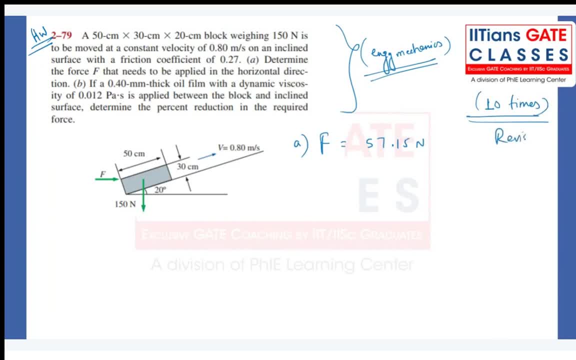 for each and every subject. that is a mantra for only and only any topper. you ask whether he will be, you know, uh, saying anything, but he might have done the reason multiple times. right, that is impossible to crack each and every problem in gate exam or getting 60 marks. 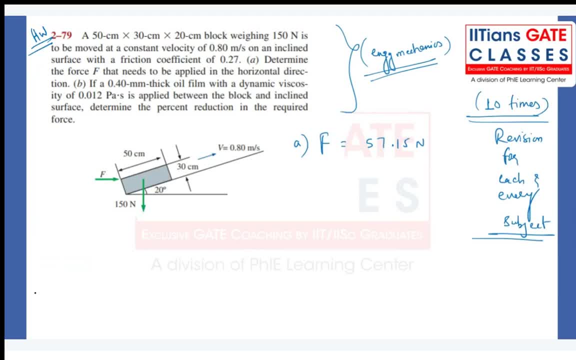 in, basically aerospace, in actual gate exam without proper reason, because you will not be getting formula itself. you know, in actual time. if formula itself is not coming into the mind, then how can you think about the concept? you should first play with the formulas, right. then you think of, uh, think of what? all the conceptual understanding, and what problems. 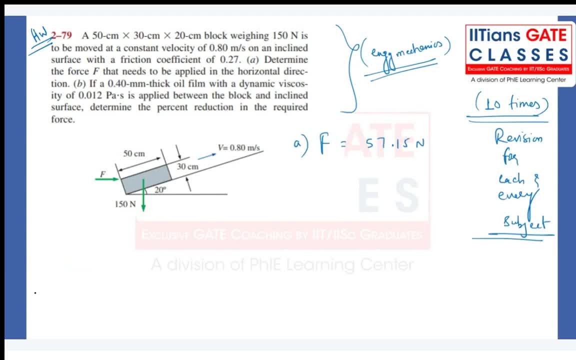 for that, only one solution is there. always you wake up in the morning and you try to take the uh empty seat, whatever the seat is there, and that particular seat, without seeing the notebook. only one time you see that right. second time you write each and every one, suppose, chapter. 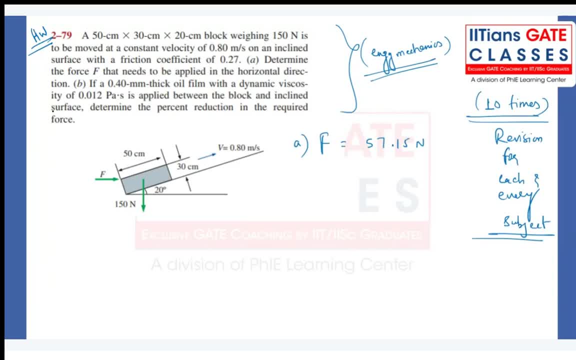 i stupid properties. whatever you remember, you try to write on your own whether it is a formula or definition, and after certain point of time- maybe it will take one hour or two hours- and you try to match with the actual notes. if it is matching, okay. if it is not, definitely you have to. 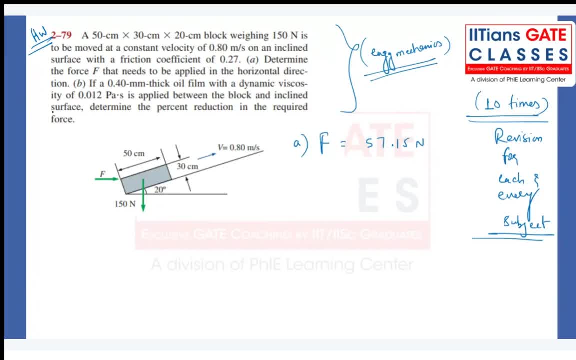 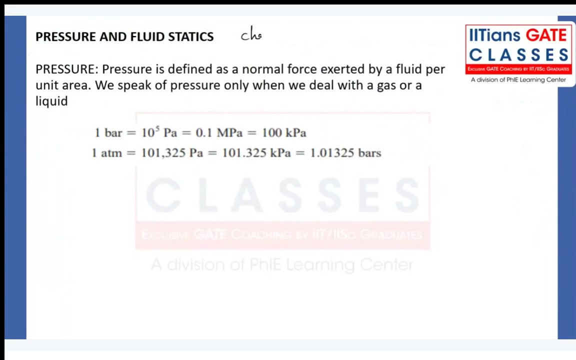 work on your memory part. you have to write again and again, again and again. you know just don't see and try to remember it, try to write and then you make a note of it and try to follow for every subject. right now, note down the chapter number two: fluid statics, fluid statics. now, here we have to. 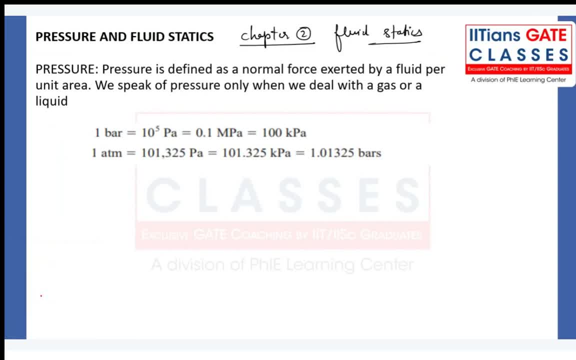 understand one more thing. yeah, pressure, when i talk about the pressure, right, pressure term is a very big term, right, this pressure value. so here you might be thinking that this is a hydrodynamic pressure or thermodynamic pressure. as of now, we have one relaxation over here that i am treating thermodynamic or hydrostatic pressure, that to be same. 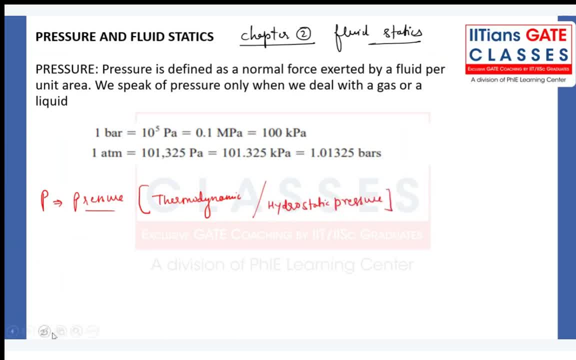 but in certain situations you cannot equate both the both the pressures, that is, thermodynamic and hydrostatic. but in most of the cases- 99 of the cases- you will be having thermodynamic pressure that is equal to hydrostatic pressure. can anybody tell me in the class that? what is the meaning? 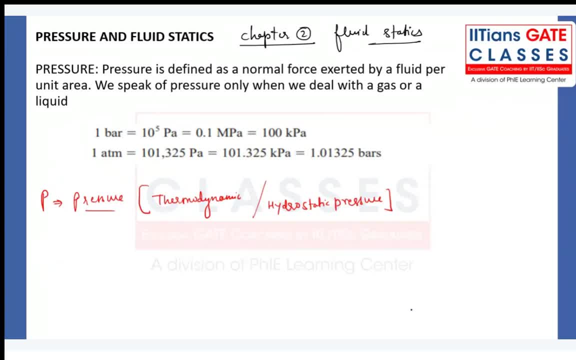 of thermodynamic pressure and hydrostatic pressure. only this slide we will discuss and we will leave for the day so that you will be having another class and you can attend that. first of all, note down the definition of the pressure. pressure is a normal compressive force. you can just note down normal compressive force. 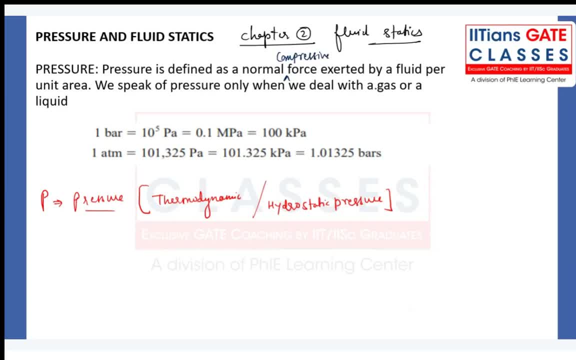 exerted by the fluid per unit area, and we speak of pressure only when we deal with the gas or liquid, because we don't deal with the solid. in case of solid, we will be having the stress right: 3d compressive stress. we call that 3d compressive stress. 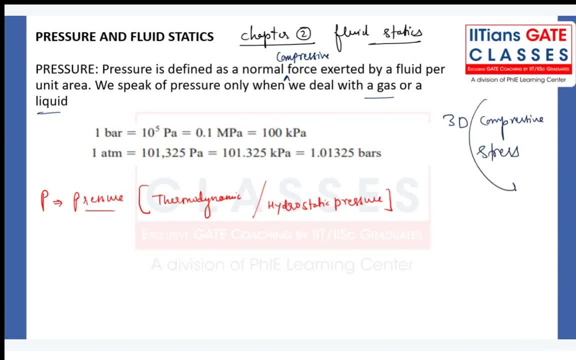 in case of fluid, we call that to be a pressure, but there is a certain difference between the pressure and the stress. both are not same, so make a note of it. hydrostatic pressure might be different. it consists of only translation, uh, translational mode of energies of the molecules. 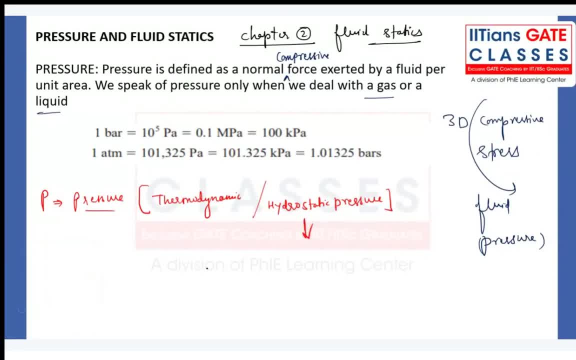 it consists of only translational mode of of energy of molecules. it consists of only translational mode of energy of molecules, whereas thermodynamic pressure, it consists of all sorts of energies, whether it is a translational, rotational and vibrational right, but in most of the cases- remember, in most of the cases- might depend. 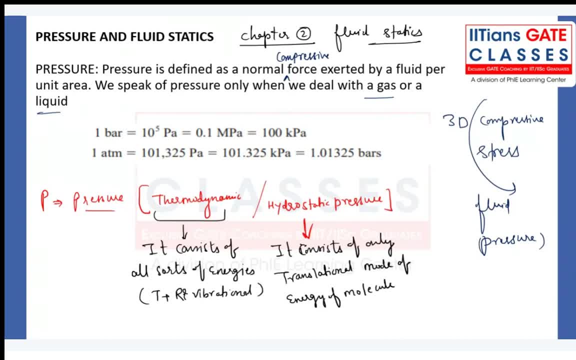 generally, we are dealing with the translational mode of molecules, right? basically, whatever the translational modes of the, you know, energies will be there that we are considering. that's why we say thermodynamic pressure. that is equal to hydrostatic pressure, that is equal to the free energy that we are talking about. so now let us talk about the 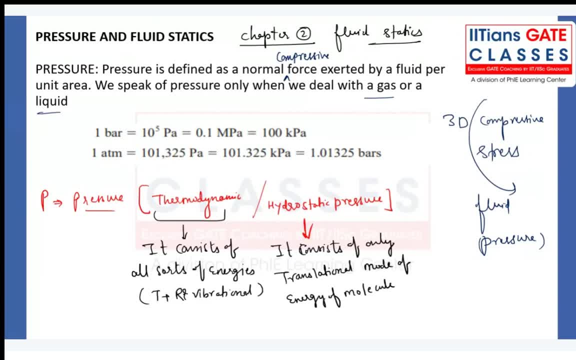 correct pressure. yeah, correct pressure is a scalar quantity. right, pressure is a scalar quantity. we also call zero order tensor. we also call zero order and the stress we call second order tensor. We don't talk about the pressure in case of solids, we say stress. So whenever, remember whether either fluid is moving or fluid at the rest condition, always. 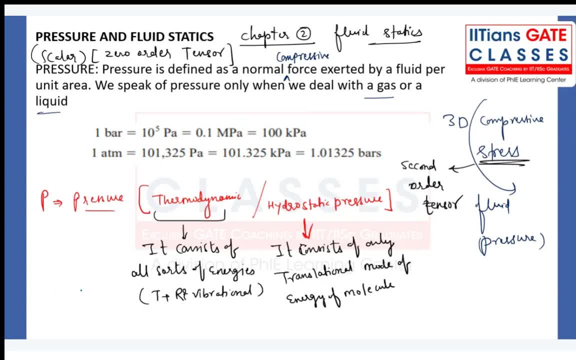 remember, hydrostatic pressure will be acting, that is the thermodynamic pressure, that is the 3D compressive force, or 3D compressive stresses will be acting in a fluid element. Right done So what is the unit of pressure? Pascal? yeah, SI unit is Pascal: 1 bar. we also say 10 to the 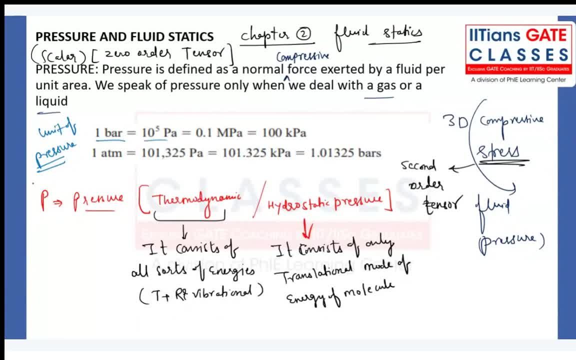 power: 5 Pascal, 0.1 mega Pascal, 100 kilo Pascal, 1 ATM. we say 101.325 Pascal or 101.325 kilo Pascal or 1.01325 bar. That means 1 ATM is greater than 1 bar. yeah, 1 Pascal, we know that 1 Pascal, 1 Newton per. 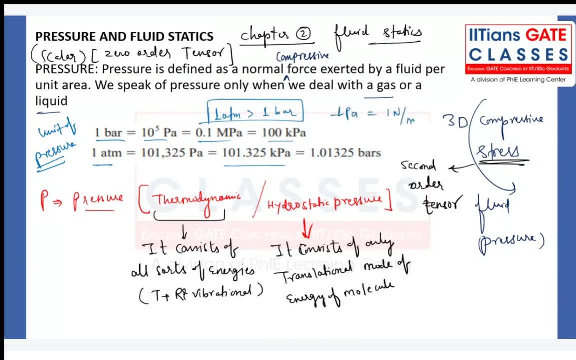 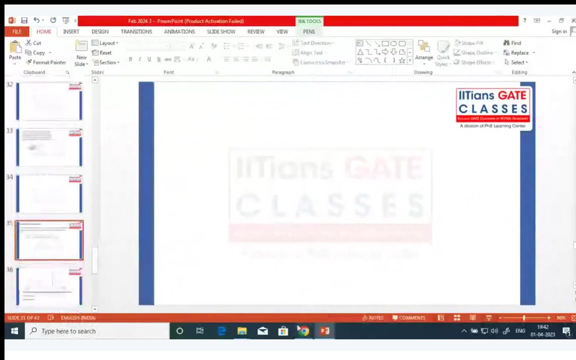 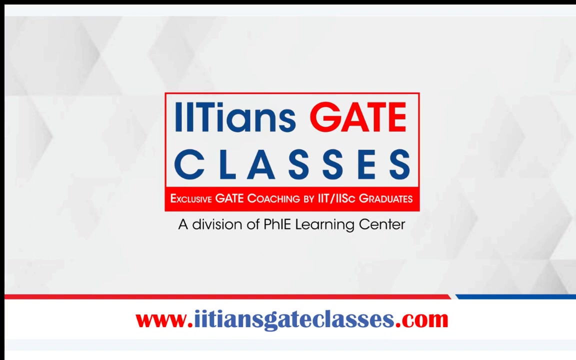 meter square Once it is done. So in the next class we will we will be discussing the absolute pressure, gauge pressure and atmospheric pressure. right, thank you all. Make a note of this. Yeah And for all, All of you have noted down. 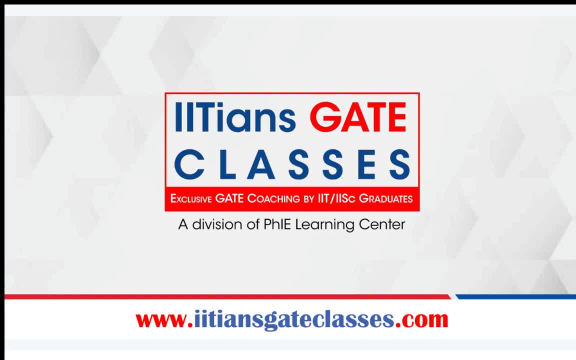 So all of you guys got the slides right, that drive for the FM fluid mechanics, Right, Yeah, So in that I have uploaded the NPTEL assignment also, so meanwhile you can start solving that also. Okay, guys, thank you.